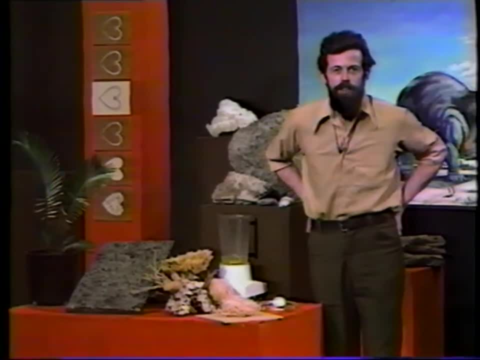 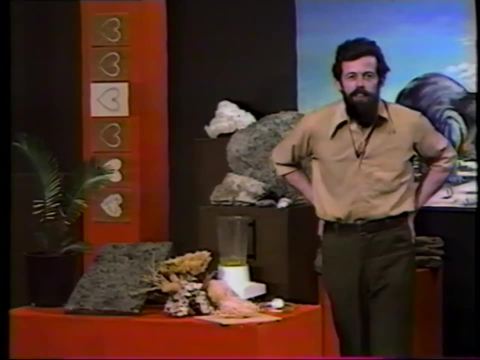 thing like a jellyfish, for example, doesn't have a backbone and belongs to the group of animals we call invertebrates. So that's easy. What, though, is a fossil? Is that as easy? Is a footprint, for example, a fossil, or is it not? And what is it? 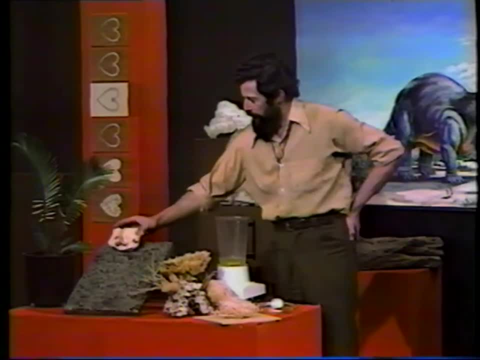 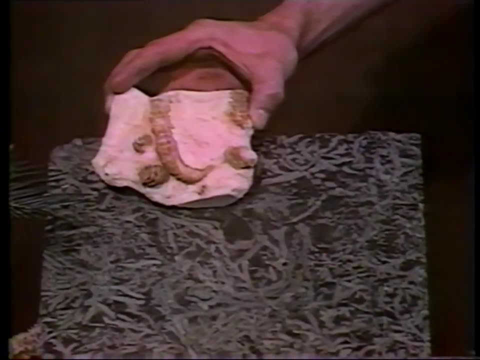 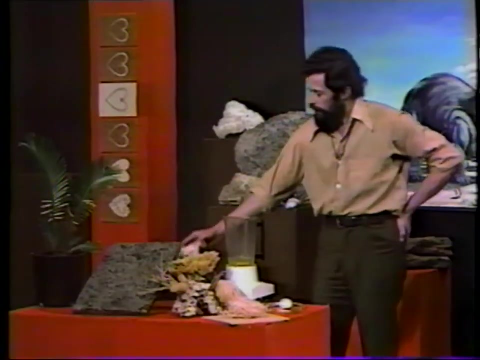 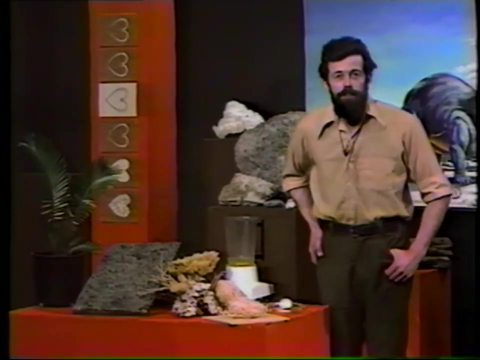 That the branching pattern on the dark specimen has in common with the rather obvious skeleton of an organism, but standing out on the light-colored specimen, Well, a fossil we could describe as any trace of life. So a footprint is a fossil. A footprint, for example, of a dinosaur. 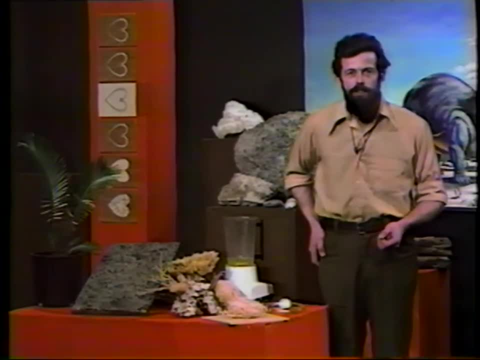 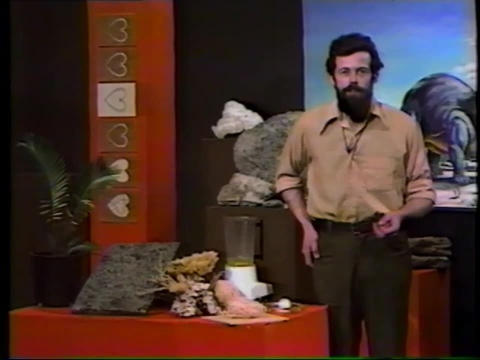 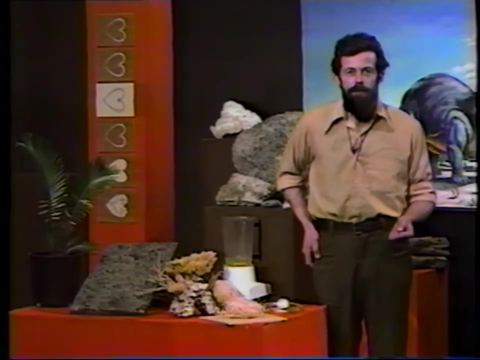 in rocks of 150 meters. A fossil that was found nearly a million years ago tells us that there were dinosaurs around in that place at that time. It tells us just as much as the fossil of a shell, for example, in the same rocks with tell us. The footprint is a different kind of hint, But it's indication, an. 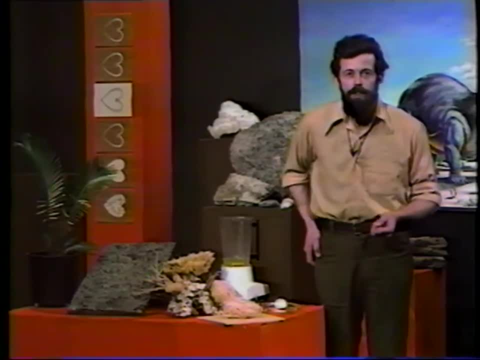 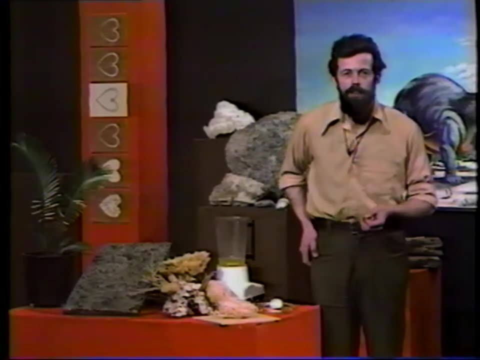 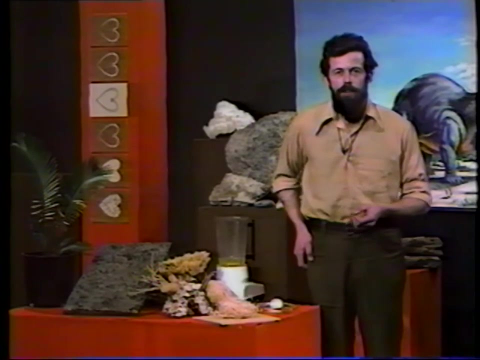 indication of organic life. A protein that we manage to trace in a rock could also be called a fossil. In that case, we would probably call it a chemical fossil. The branching pattern on the pattern in that dark colored rock were what was formed by burrows, by organisms burrowing in mud. 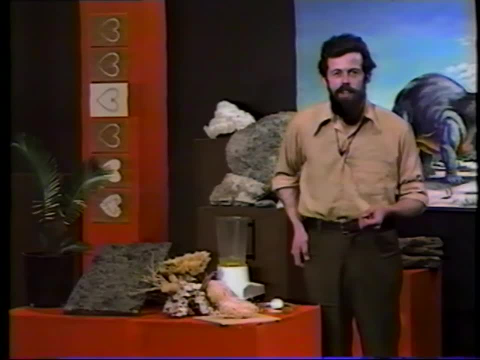 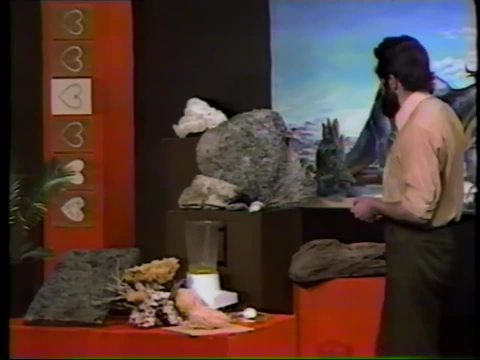 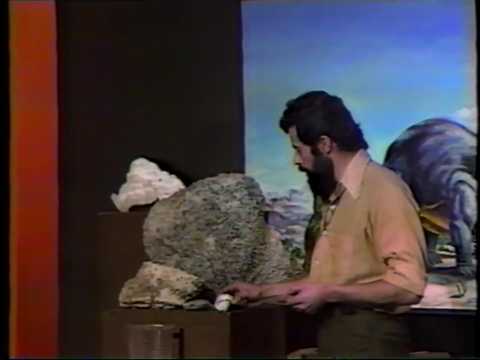 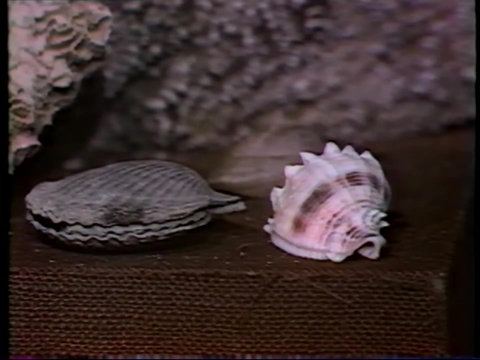 we would call out a trace fossil. it's a trace of life rather than the organism itself. let's have a look at what fossils are made of, what they consist of commonly. this is a recent shell, the kind of shell that you could pick up on a beach at the present time. in fact, it's one that I picked. 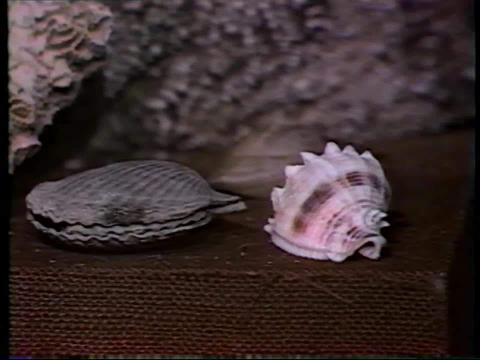 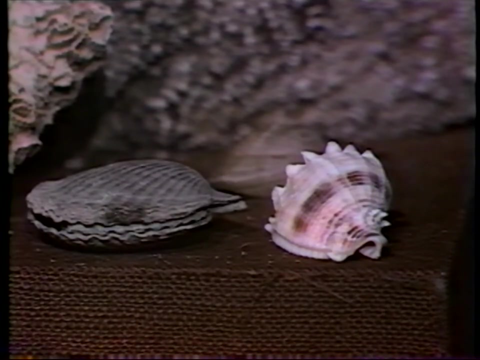 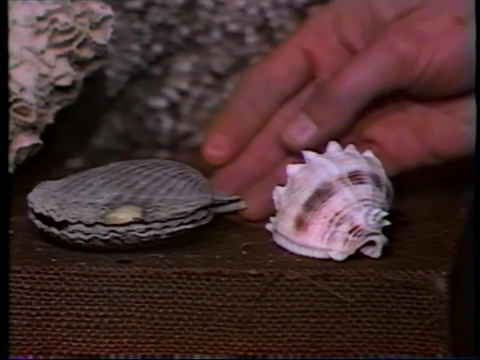 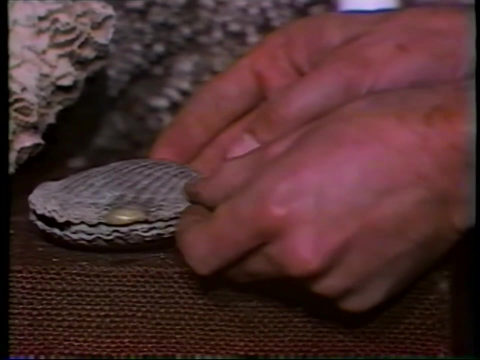 up on one of my forays to Florida, and if we put acid on it, it fizzes. in other words, it's calcium carbonate. that's a test for calcium carbonate. if we put acid on this fossil shell, you, it too, fizzes, and quite clearly, although it's 15 million years old and is quite clearly a. 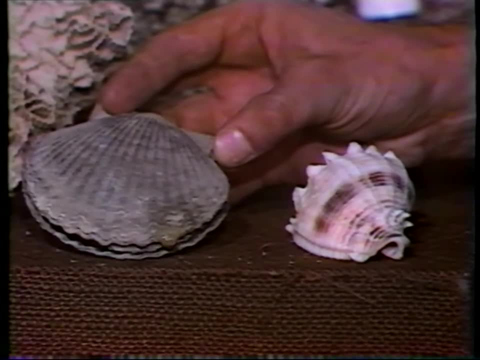 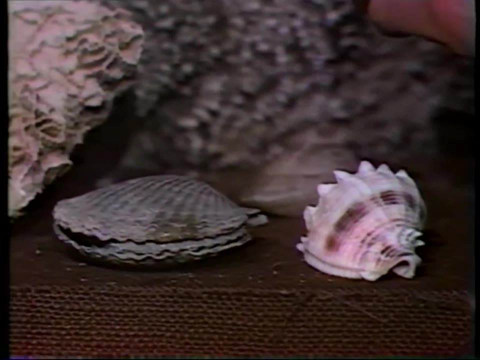 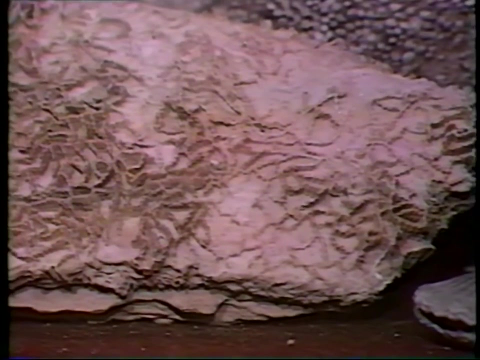 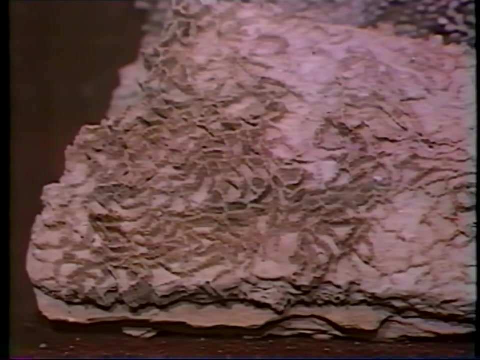 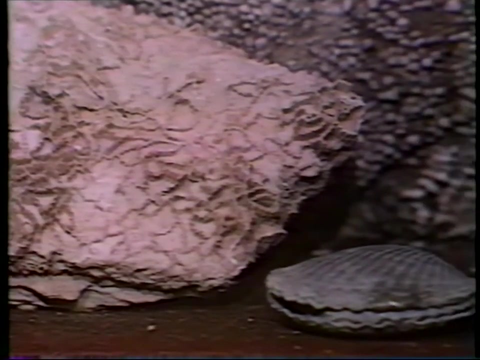 scallop shell and a fossil scallop shell. it still consists of the original calcium carbonate. now let's try it on this same test, on this fossil coral. corals consist of calcium carbonate, but this fossil doesn't fizz. it consists of something else. if we were to test it with a knife, we'd find that it consisted of silica, of quartz and 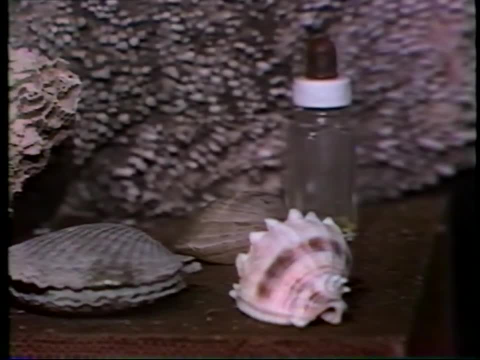 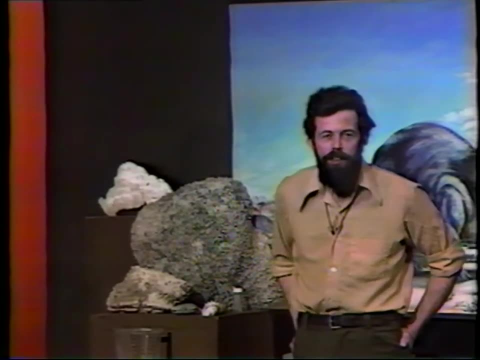 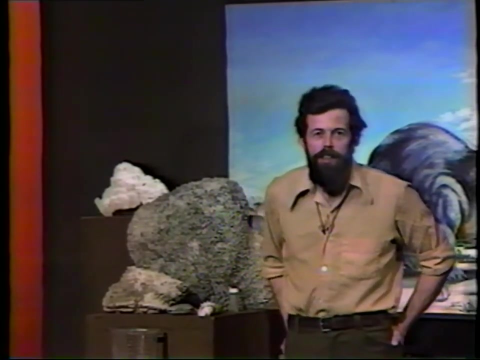 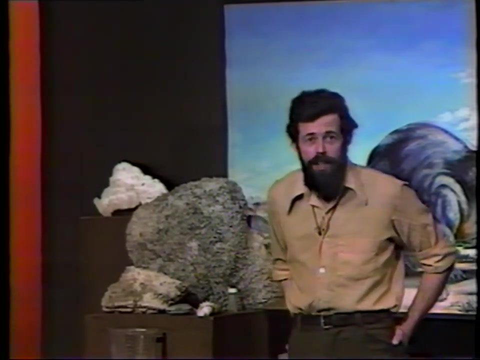 we could find that out simply by the hardness. now, how does that come about? well, if the coral is buried in mud and that mud becomes rock in the way that we've discussed, when we looked at the rocks- weDIFF rocks and the corals correspond to some procedure for the 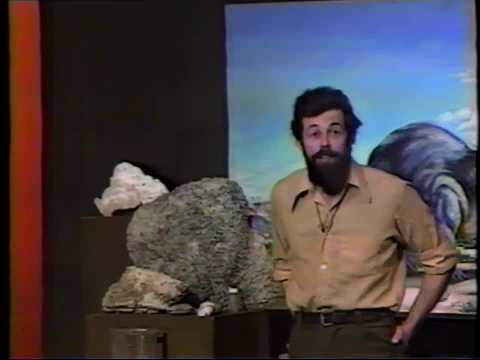 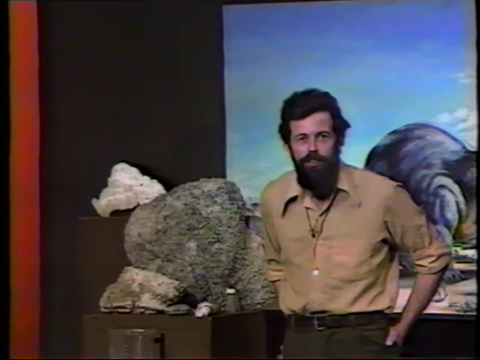 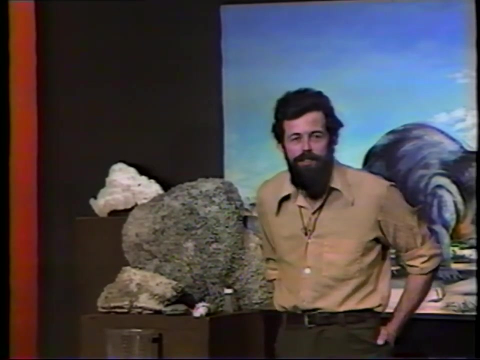 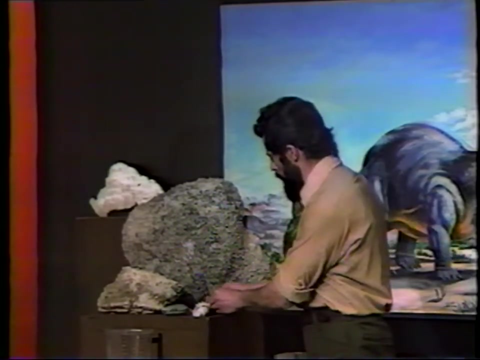 fusion process. after the desiccation process caused by the TC, it causes the athlete to deflate. so if producers take� 땕 in the cavity that's left, So in that way we get a silicified fossil. Let's look at another example In this case. 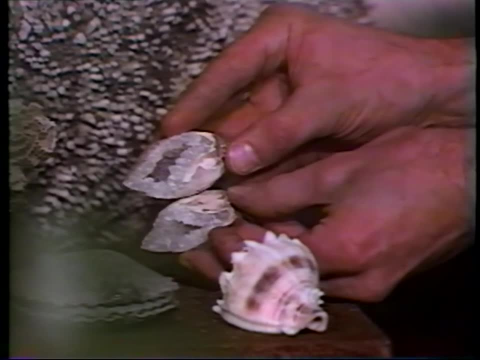 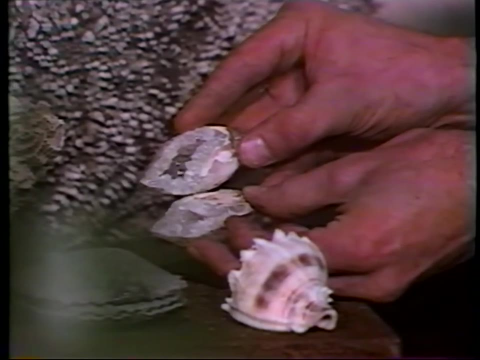 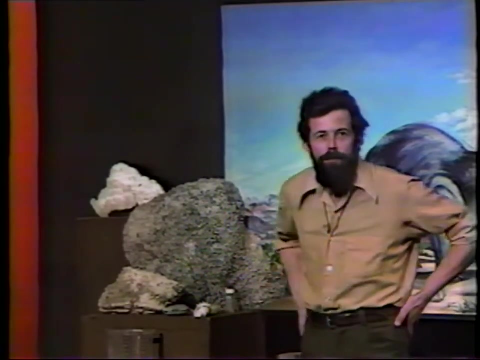 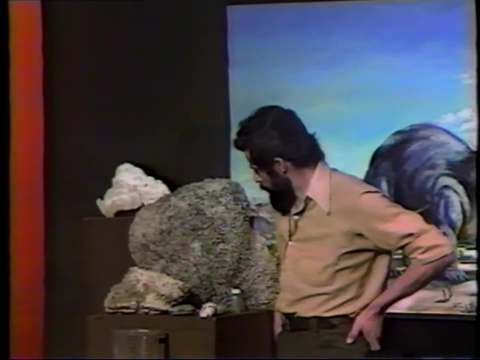 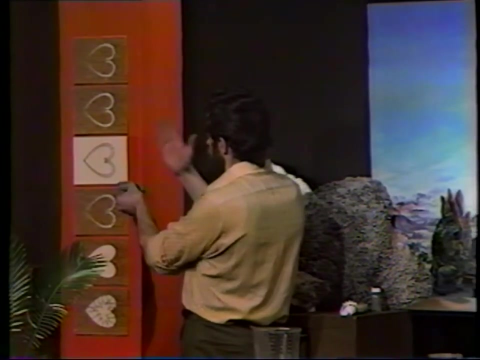 the fossil consists of rather beautiful crystals which we can recognize as quartz crystals. How does that kind of fossilization or that kind of preservation come about? Well, let's look at a series of diagrams which will summarize the processes. Let's cut our scallop shell, for example. 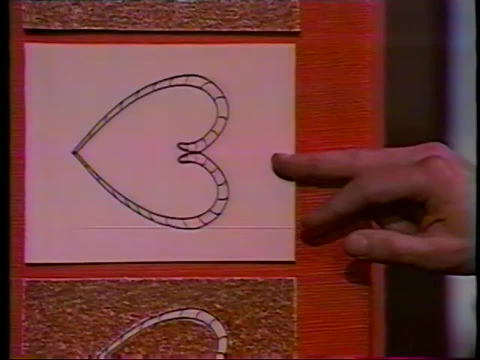 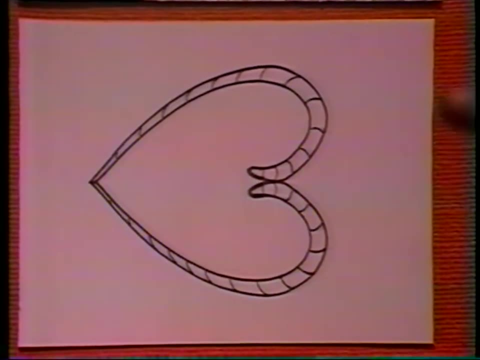 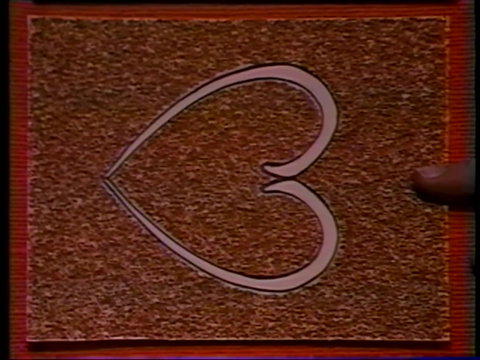 down the middle here, and that's what this diagram represents. Here is a shell as we would perhaps find it on the beach. Here. it is buried in sand, and water percolates through the sand and dissolves away the material of the. 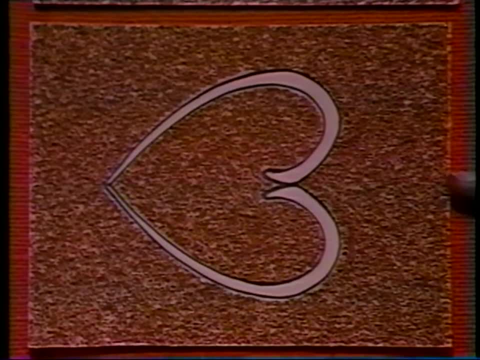 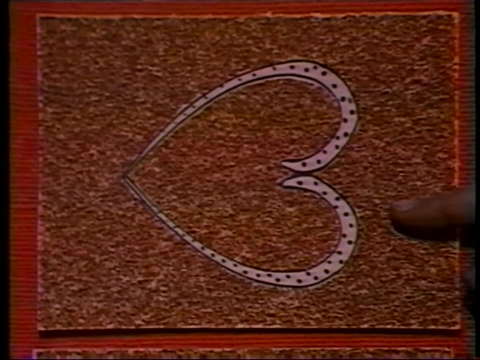 shell, leaving in there a cavity, a cavity in the shape of the shell. Along comes the later, water precipitates in that cavity and leaves us with a silicified fossil. And then here's a shell as we would perhaps find it on the beach. Here it is buried in sand, leaving in there a cavity, a cavity in the shape of the shell. And then here's a shell, as we would perhaps find it on the beach. And then here's a shell as we would perhaps find it on the beach. 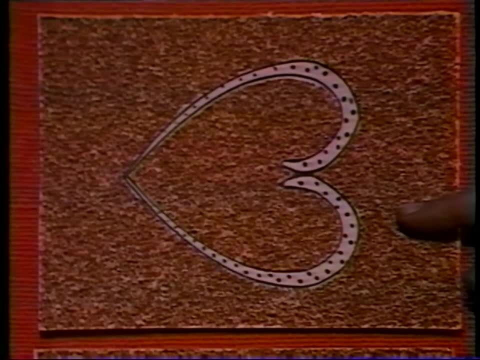 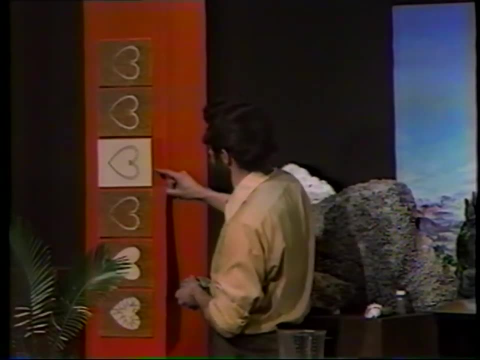 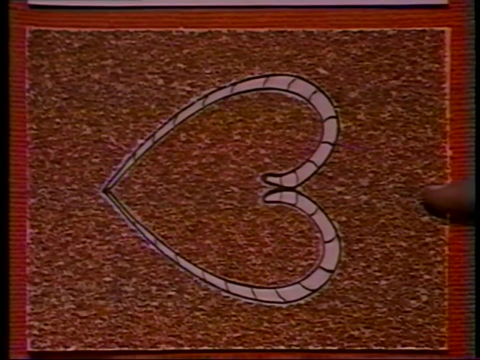 In other words, a shell turned to silica replica of the original shell. Now, that's just one route that we could follow. Let's take another route, from the shell down to this stage, where the shell itself is perfectly preserved in the sandstone. 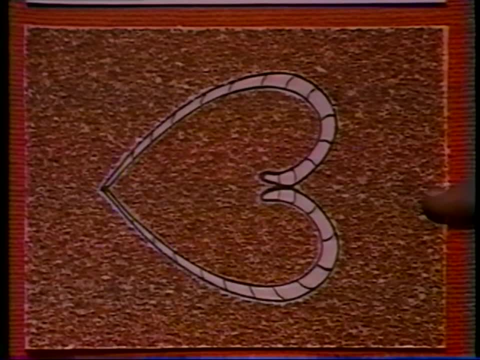 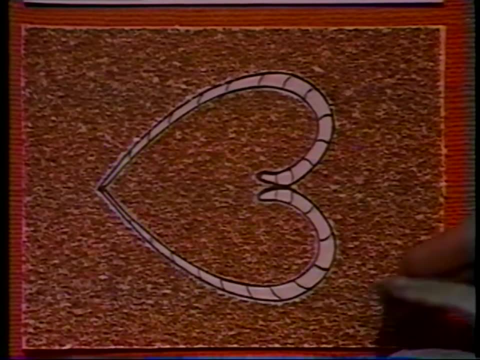 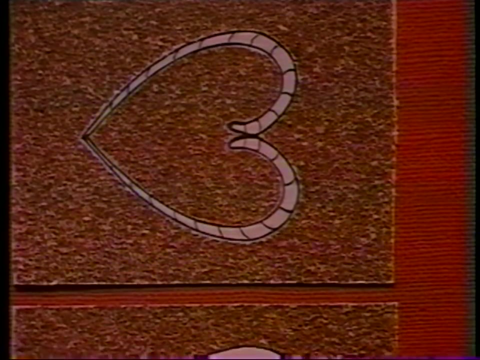 The process may stop there and we may come along with a hammer and hammer out that shell, just as we were able to do in the original shell. we were able to hammer out this one and inside is sand. just as inside this one there is sand. 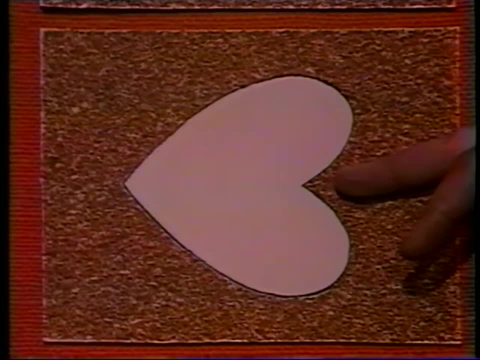 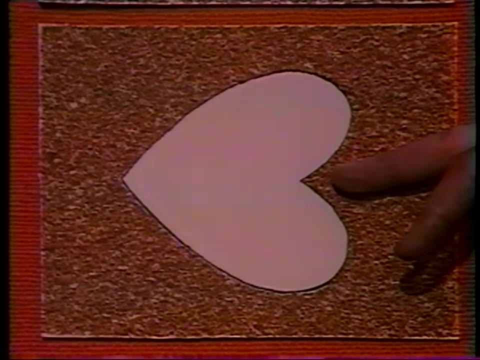 If the shell is not filled with sand and the same kind of acid solution comes along as dissolved away the shell which led to the state of silicification, then we may end up with a cavity, simply a cavity in the rock, rather like a mold of the original shell. 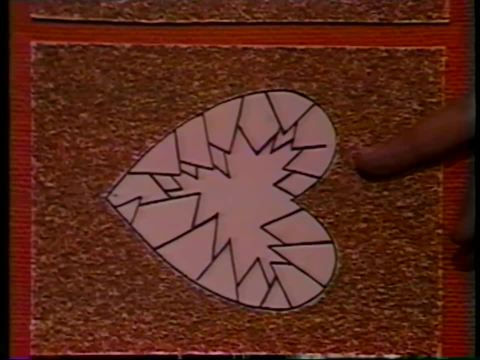 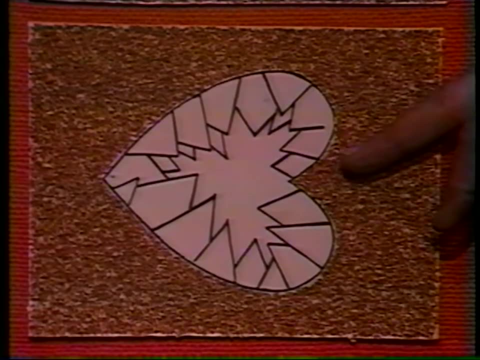 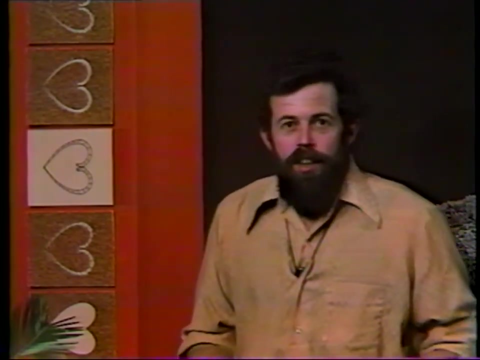 And if then comes along our silica rich solution and quartz precipitates in the cavity, in crystals, then we have the third kind of fossil that we looked at, the fossil with the rather beautiful quartz crystals in it. Now, those are just three ways of getting fossils. there are lots and lots of other ways, but 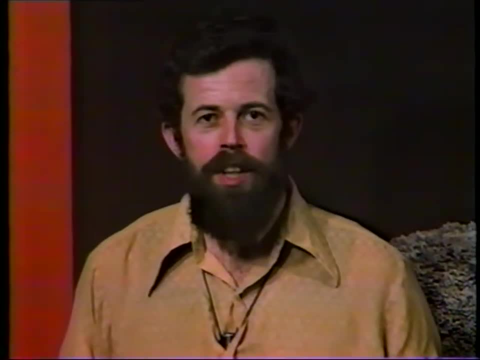 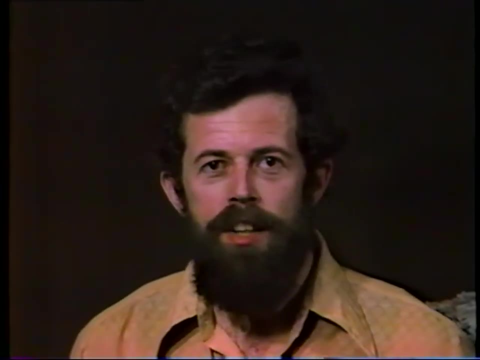 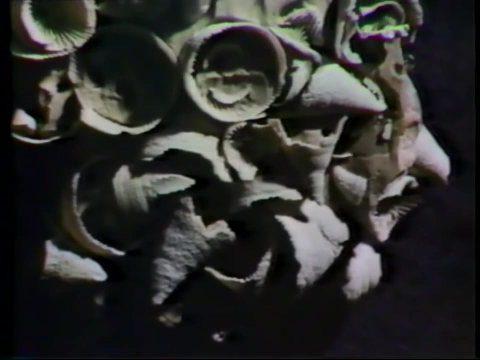 silicification is a very important way because it gives us sometimes very, very beautiful preservation of the most delicate structures of shells and calcium carbonate skeletons. These are Silurian horn corals partly dissolved out of the limestone. Each one is about an inch or an inch and a half tall and about the same across. 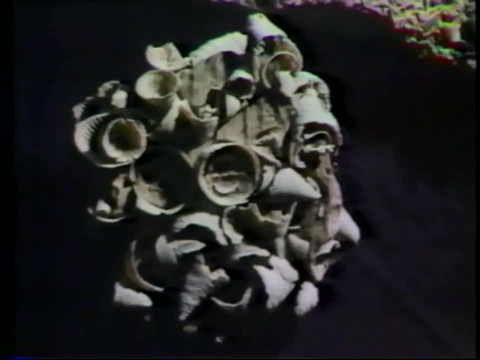 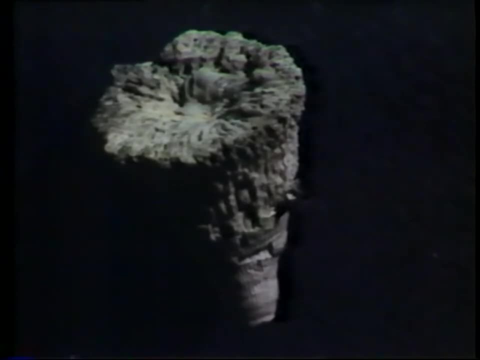 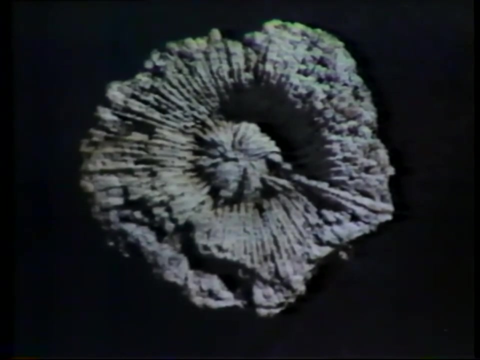 The soft body of the animal sat in each of the cone-shaped chambers. Okay, In this specimen the radial divisions which divided the soft body of the organism into many sort of leaves is visible. This is a view from the top of a specimen that's about an inch across and comes from: 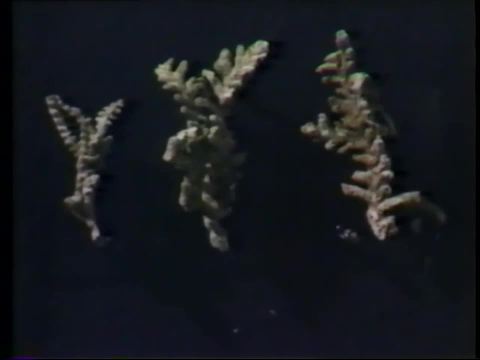 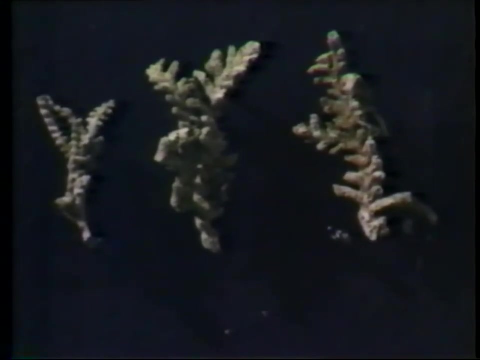 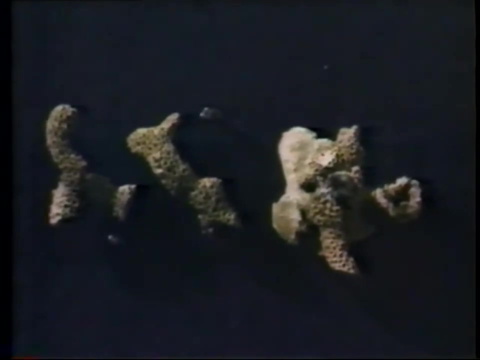 Manitoulin Island. These are bryozoans totally dissolved out of the original Permian limestone in which they occurred. They're also about an inch high, Rather twiggy looking ornaments. These are also bryozoans of a different kind, also from a Permian limestone, quite totally. 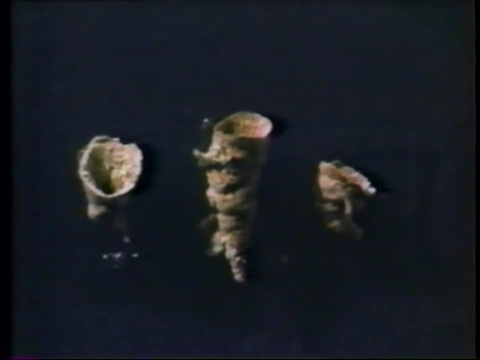 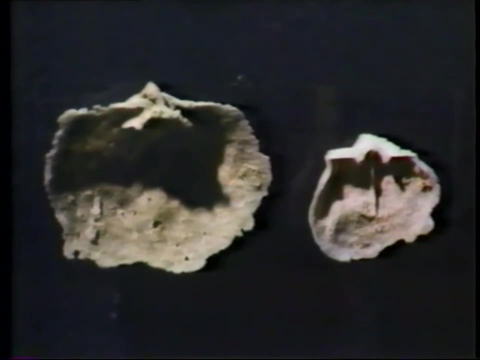 dissolved out. These are very small corals, no more than an inch tall. Once again, each of them was occupied by a single individual. These are brachiopod shells. Brachiopod has normally two shells, so the individual has had its shells broken away. 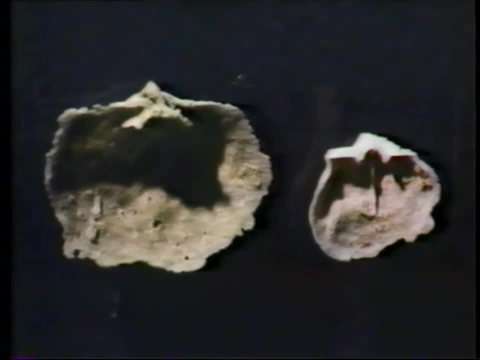 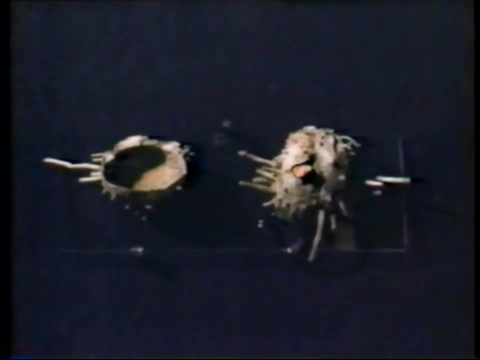 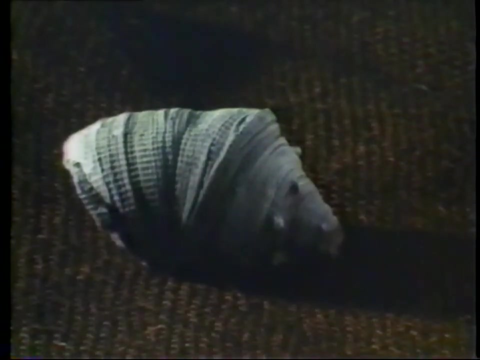 from one another. These have been totally dissolved out, also from Permian limestone. In these brachiopods, external spines which the animal used to anchor itself into the mud of the sea floor are clearly visible. Silicification is not always the means of preserving very fine, delicate features. 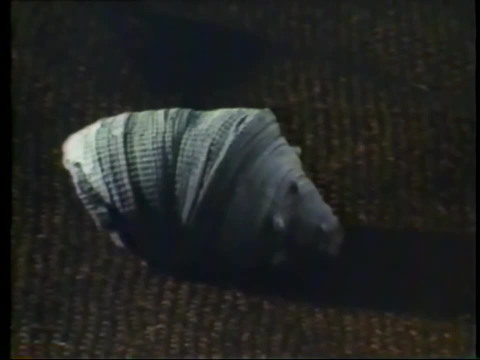 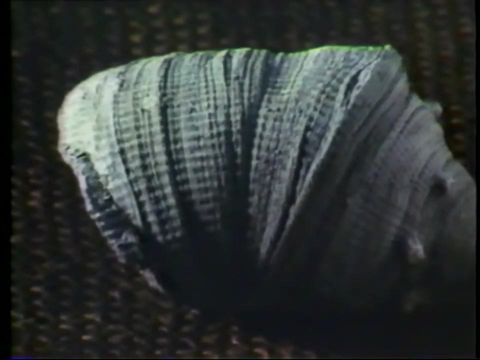 In this horned coral, the growth lines, which are the lines that you can see running around the surface. The corals in the circumference of the coral are still the original calcium carbonate shell. The calcium carbonate was deposited by the coral according to the temperature and the 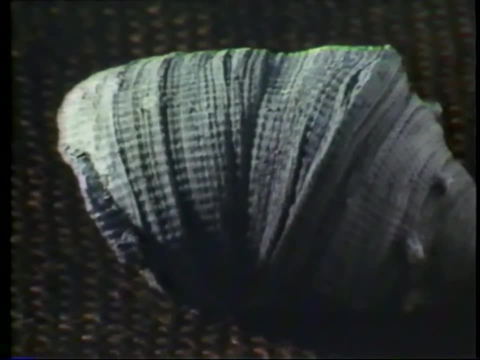 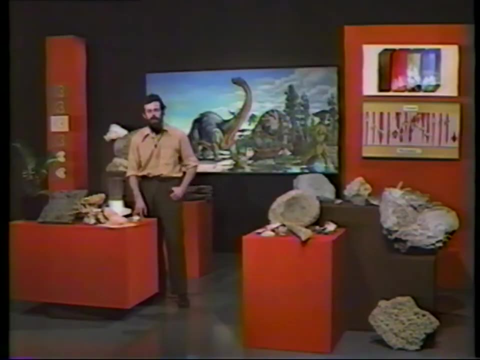 daylight available. It's from specimens such as this that we can draw conclusions about the daily growth of corals. By attempting to recognize seasonal growth and the number of days in the four seasons equal to the year, it's possible to make some estimate from corals as well preserved. 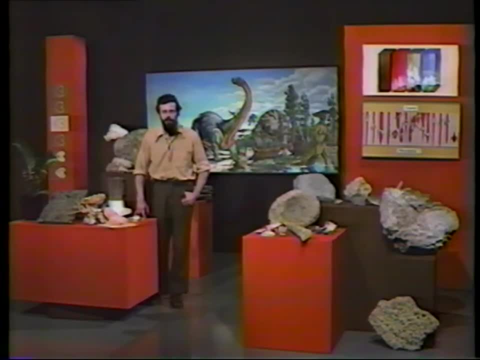 as that one of the number of days that there were in the year at the time that the fossil grew. And strangely enough, it's been found that there are good reasons for believing that in the Devonian and in the Silurian there were a great many more days in the year than 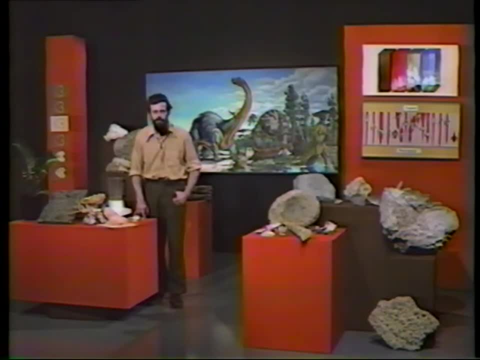 there are now something like: oh, four hundred and ten, four hundred and fifteen days per year instead of three. sixty-five, In other words, there were… The earth was going around… A year faster, was rotating faster, So it's possible to draw some very interesting conclusions. 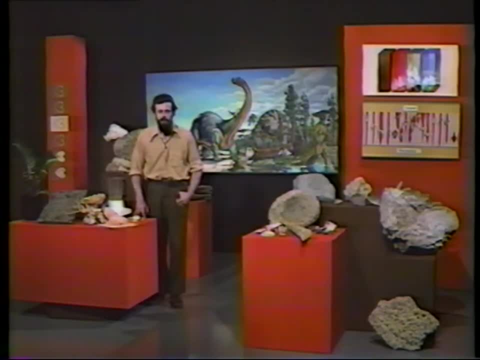 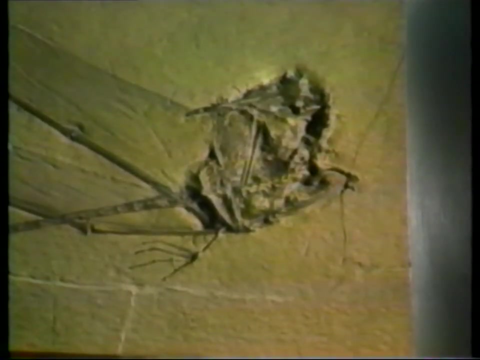 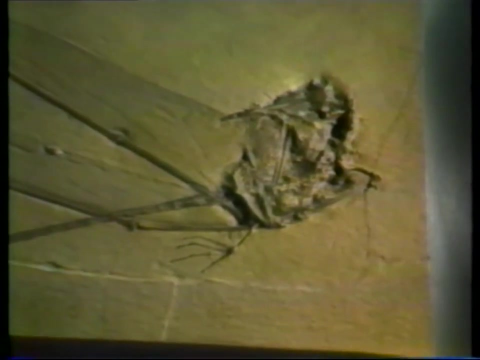 from fossils, if you can read them correctly. Preservation of impressions of membranes is quite rare, but also occurs sometimes. This is the skeleton of a medium-sized Jurassic reptile which was able to fly. The skeleton is quite crushed on the right there. 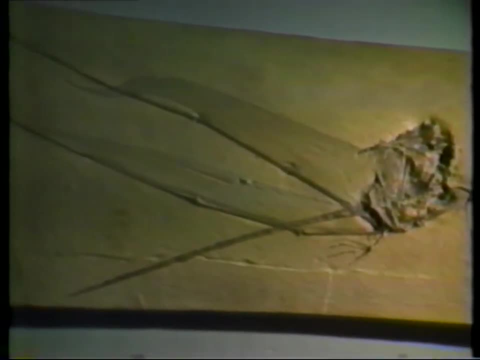 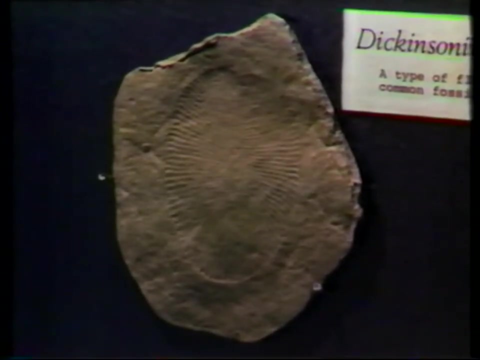 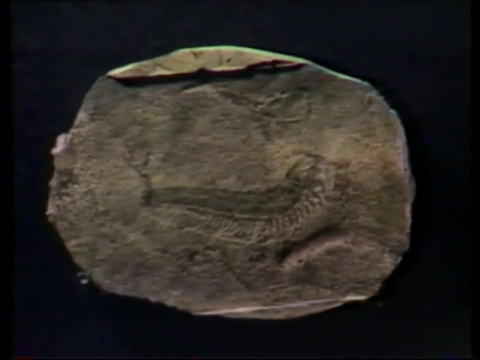 But the membranes which gave the reptile a wingspan of two or three feet are still quite well preserved. This is the impression of a soft-bodied organism rather like a worm, And this is a somewhat smaller but more complex-looking worm. 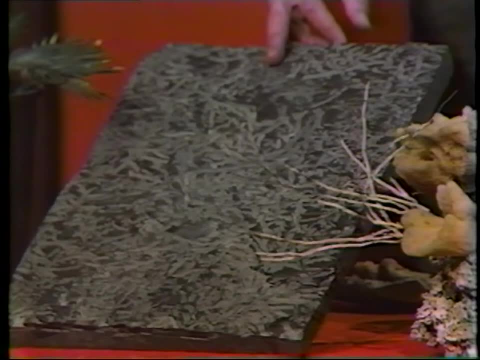 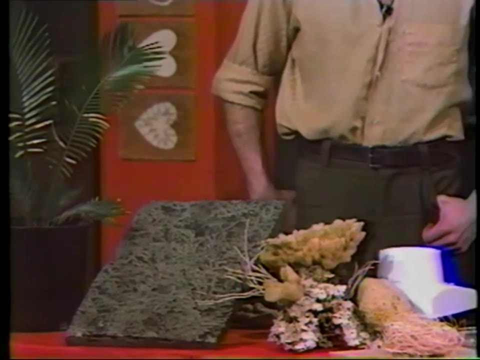 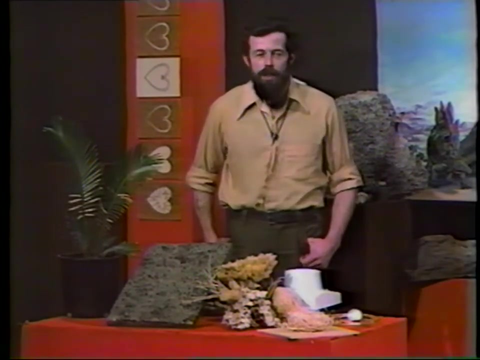 These trails in this once muddy sediment were produced by soft-bodied organisms. So we do get some record, by the means of impressions and by trails, even of organisms that were totally soft and which totally themselves rotted away. There are other peculiar ways of fossilization. 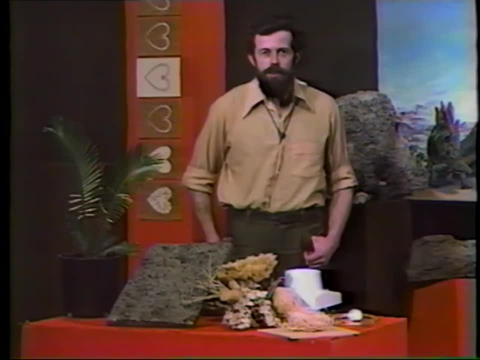 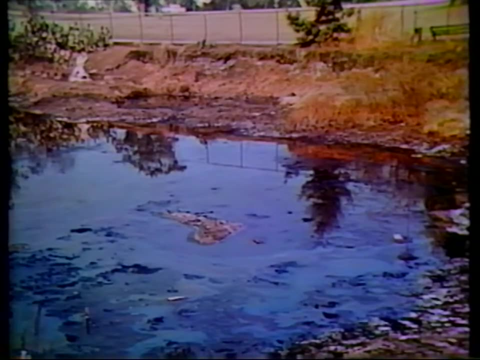 One of the most odd and most unique is in California, where tar pits of a million or two years ago appeared to animals unfamiliar with what tar looked like. obviously, This is the first thing that comes to mind, The first thing to think about when you think about tar. 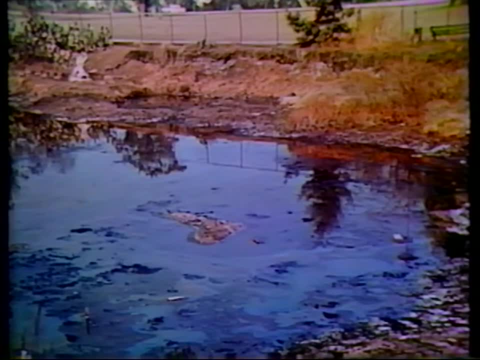 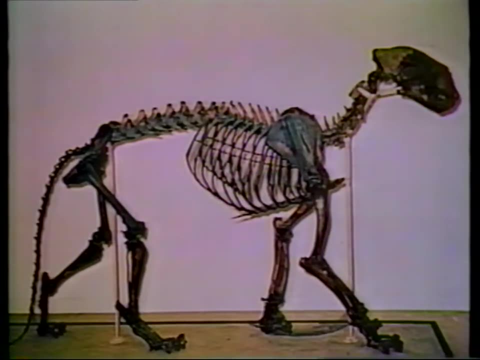 is the fact that it was a species that was eating these good watering holes And they went for a drink And they found themselves engulfed in tar. By fishing out the skeletons, today we're able to make reconstructions of, for example: 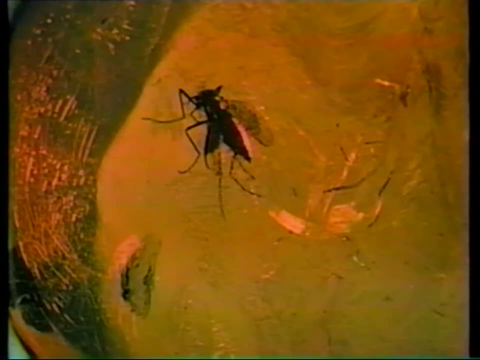 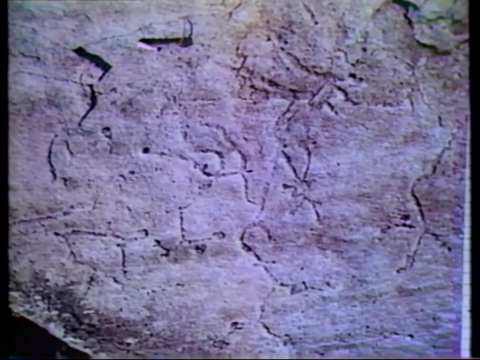 saber-toothed tigers and this panther. The preservation of insects in amber is another rather odd preservation, whether the traces we've got in rocks are fossils or not. For example, these are from a very old sandstone in the Sudbury Basin and we're still not sure whether those are traces of life or 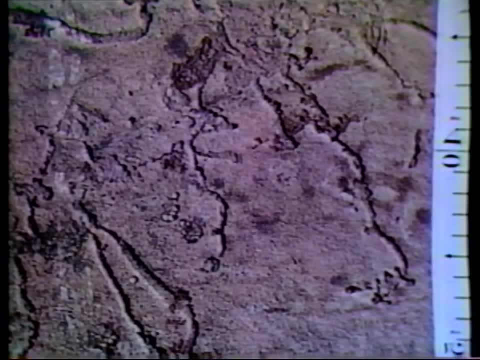 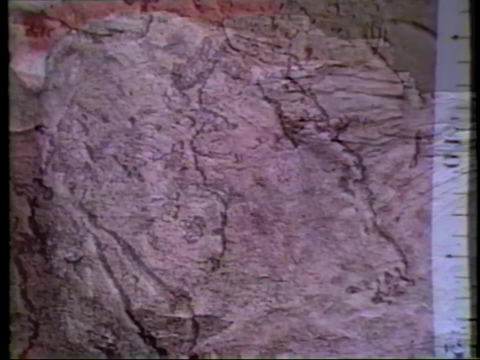 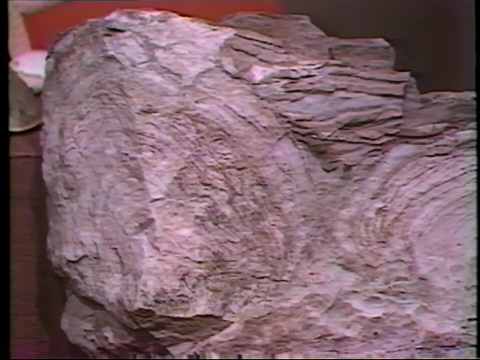 whether they're something that was produced by something that was not living, by some phenomenon of water coming out of the sand or something like that. Now the Precambrian record, the Precambrian fossil record, has got quite a lot of algae in it like that similar to this specimen There. 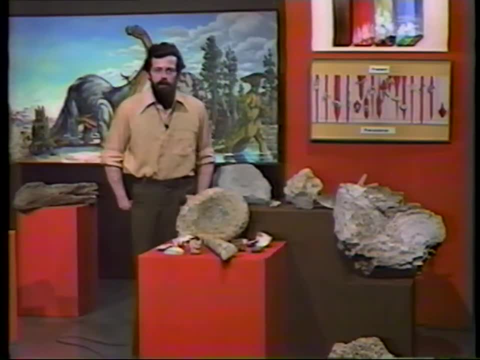 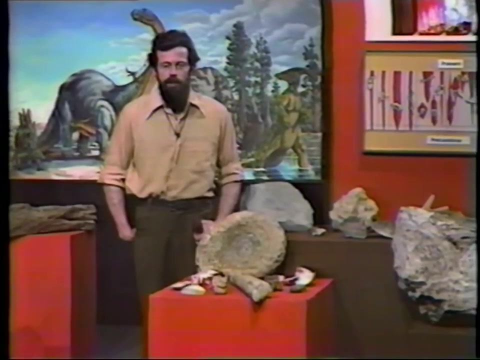 are also in some places the record of Precambrian cells. There are some in the Gunflint Church you may remember. Also at Bitter Springs, which is a sediment, or a place in Australia where there is sediment like that of the Gunflint, but the age is about 900 million years. there's evidence that 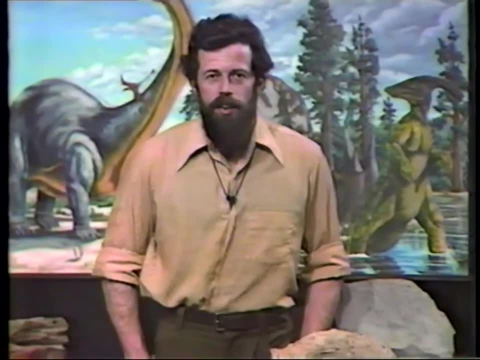 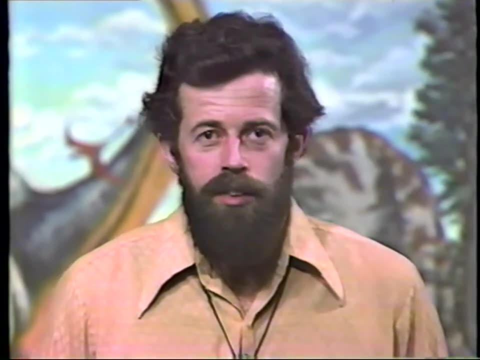 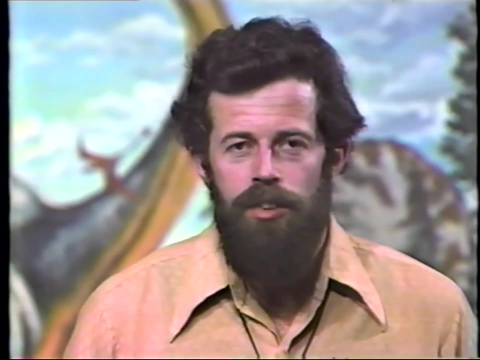 sex had been. There are some cells there which are dividing in a manner which suggests that they were produced by a sexual union And that was very important for fossils or very important for the development of life. Once sex had evolved, then it was possible for variable offspring to be produced and for 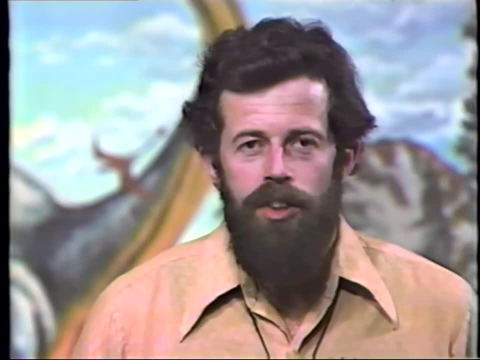 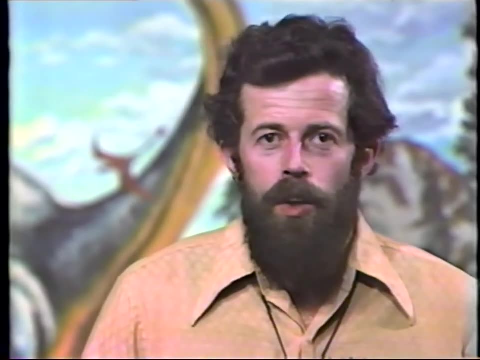 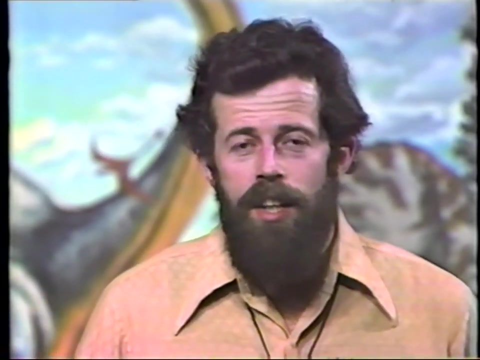 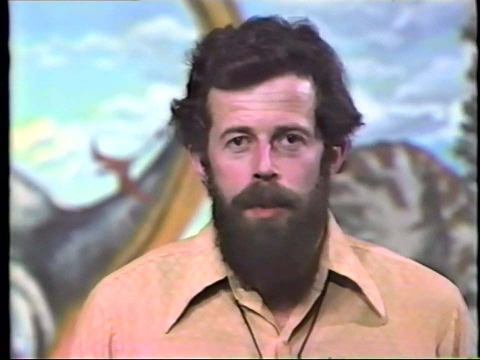 those offspring perhaps to be a little better adapted than their parents and so to, by natural selection, improve the viability of the organisms and to evolve new, better adapted species, and so forth. Now, unfortunately, between 900 million years ago and the next rich fauna, there's a big gap. 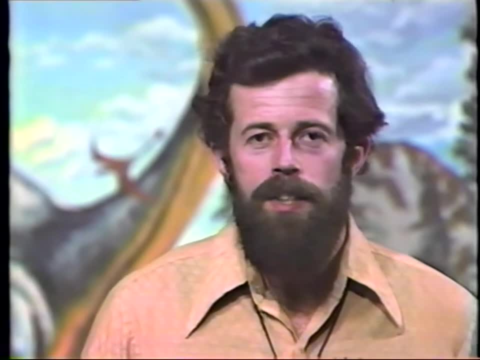 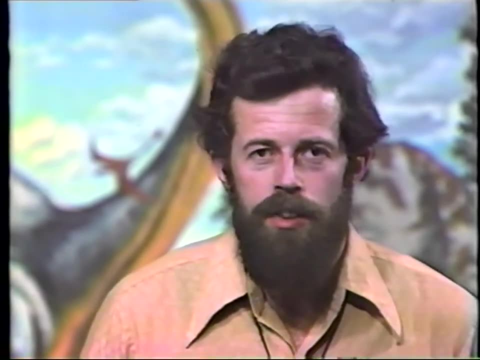 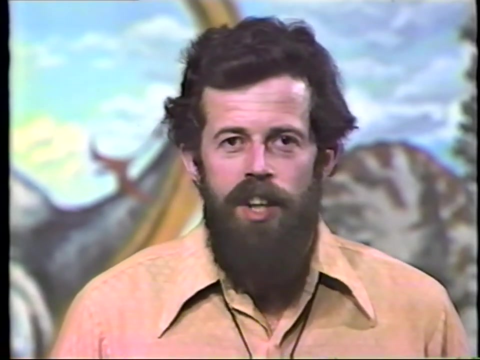 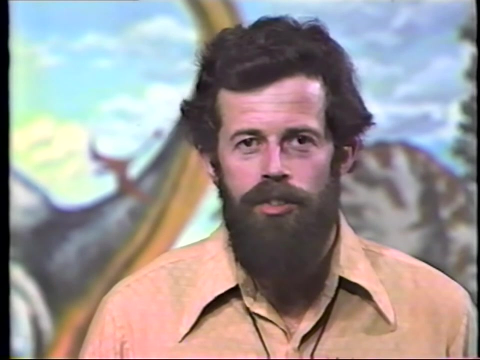 There was a glaciation that lasted perhaps 100 million years, between about eight and seven hundred million years ago, and the geological record is almost blank of fossils. And the next fauna that we find is very, very rich in diversified organisms. The Paleozoic Faunas of 600 million years ago were extremely rich, and this Ediachera, which 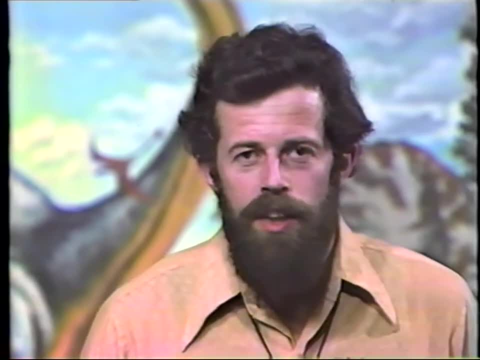 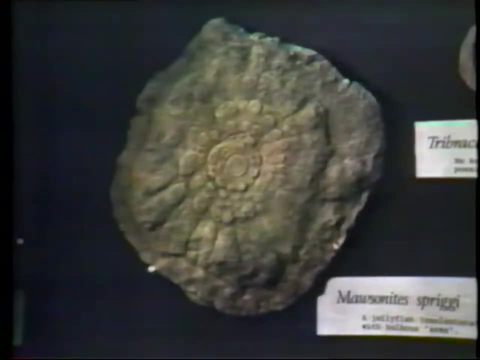 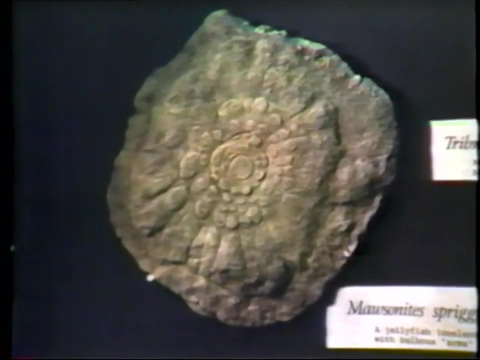 immediately precedes those Cambrian Faunas in Australia is quite rich also. Let's have a look at the Ediachera Fauna. finance brushes, ediachera voices, elders, Canadians of a jellyfish. When it was alive it would have floated near the surface filtering organisms. 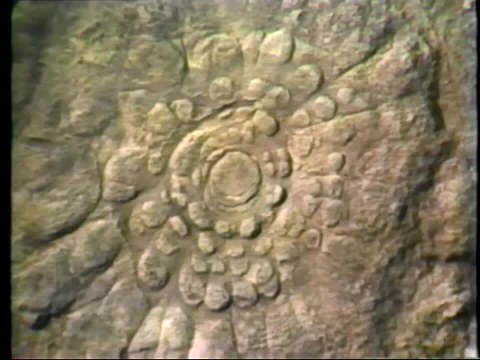 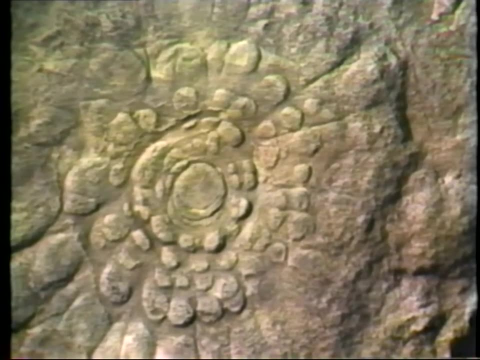 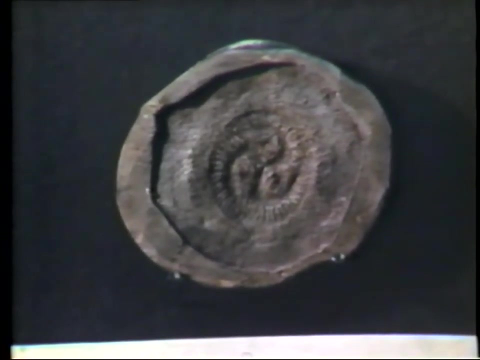 out of the water. It must have become stranded in shallow water or have died and sunk to the bottom. The divisions of its body are quite complex. In the central part of this cast is yet another impression. This organism has no known relatives. It may be related to the. 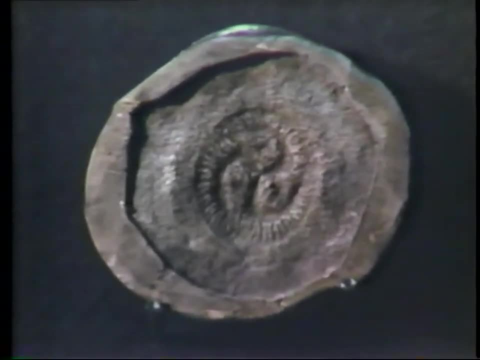 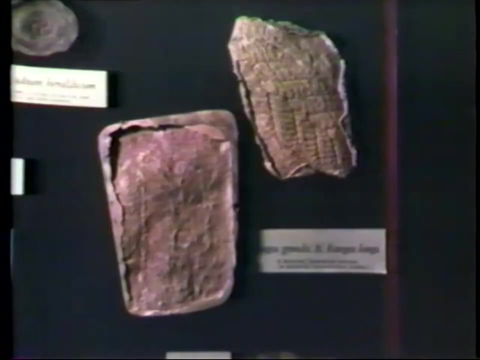 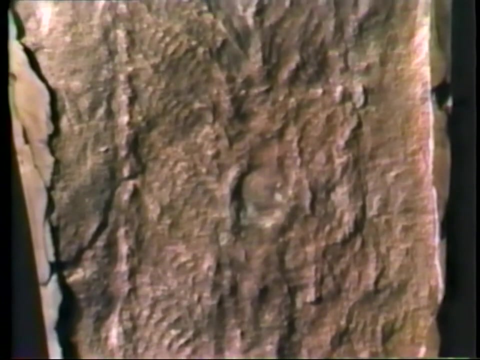 sea urchins, and it's thought to have lived on the sea floor itself. These sea pens, or sea whips as they seem to be, have also only left impressions in the fossil record. They look rather plant-like and probably seem to be a faeces. 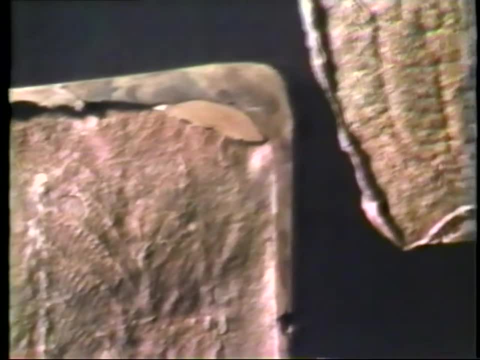 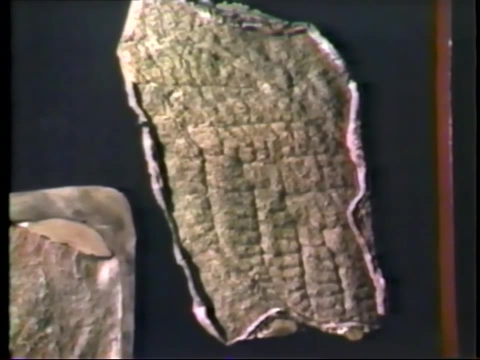 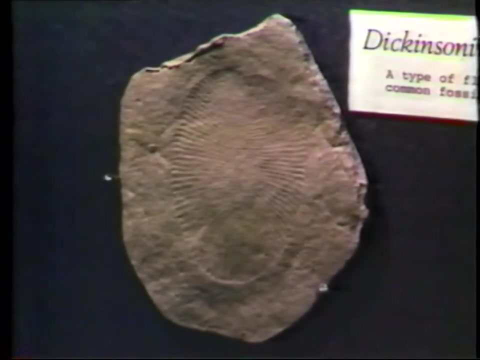 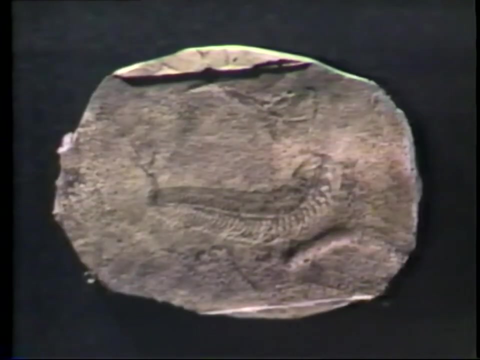 stood several inches high and waved above the sea floor, being anchored at their base. Impressions are rather plant-like. This impression that you've seen already is that of a flatworm-like organism. It's one of the commonest fossils at Ediacaro. 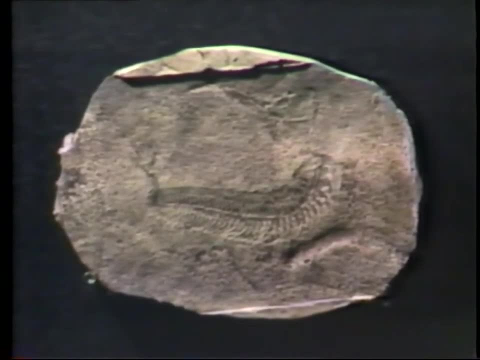 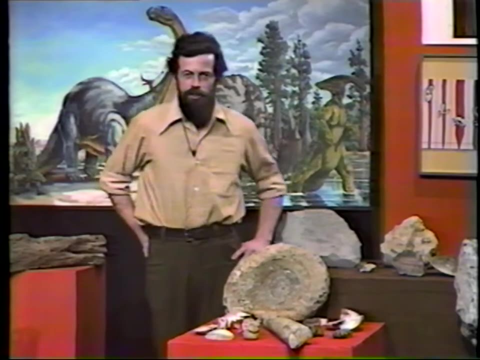 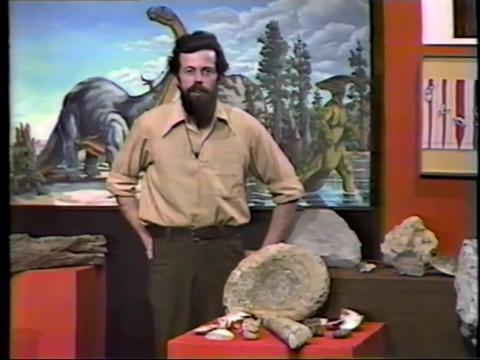 And this that you've also seen is of a worm-like organism that probably lived in much the same way on the sea floor. Let me emphasize what you've just seen there. Those fossils from the Ediacaro Hills of Australia are the first fossils which we find. 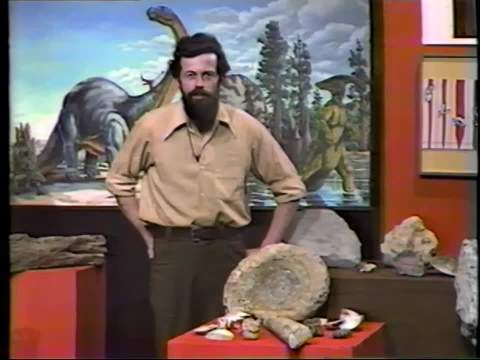 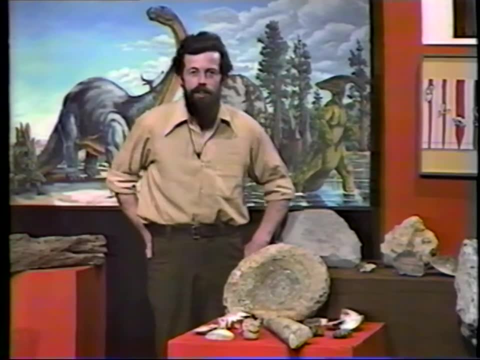 that were composed of many cells. Each of those jellyfish was a many-celled organism. Each of the worms was composed of many cells. That's a tremendous evolutionary jump from the single-celled organisms which preceded in the fossil record 200 million years earlier. 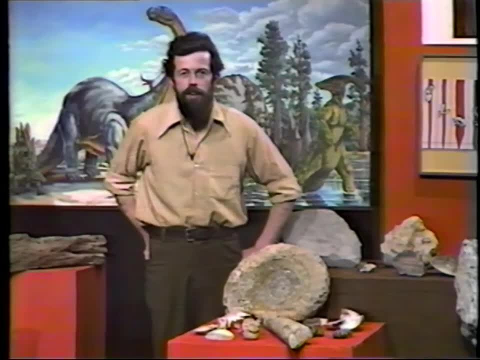 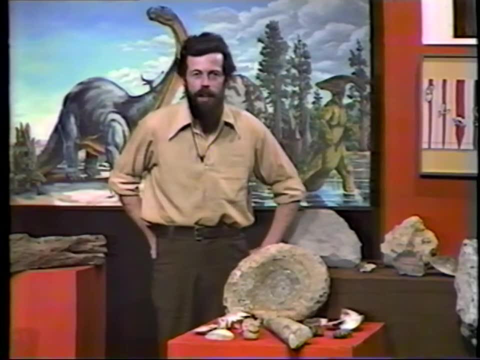 Unfortunately, as I mentioned, there's a worldwide, or seemingly worldwide, glaciation in between those two parts of the fossil record And we don't know exactly how animal life made that jump from single-celled to multi-celled organisms, But it was a vital jump. 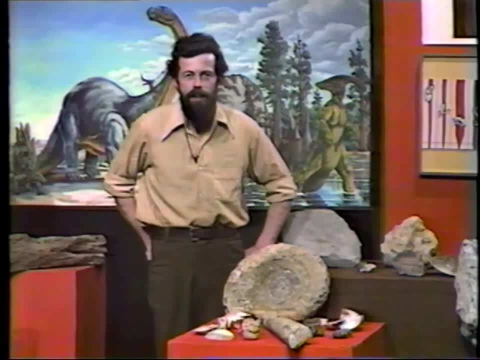 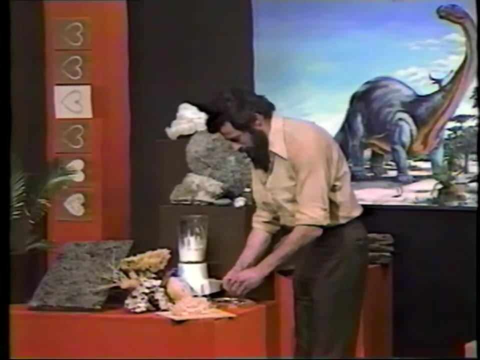 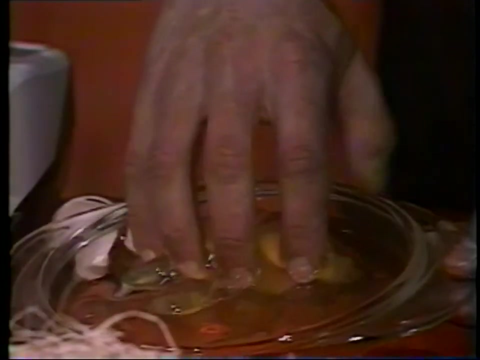 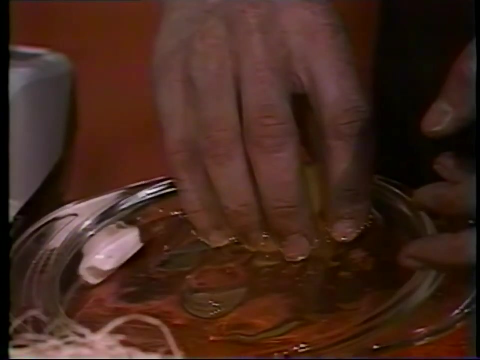 It was vital to the continued evolution of animal life And we can illustrate the kinds of advantages that multicellular existence gave to animal life back in our kitchen, The white of egg is very like the cell material in the single-celled organisms And, as you can see and as you know, it's impossible to give. 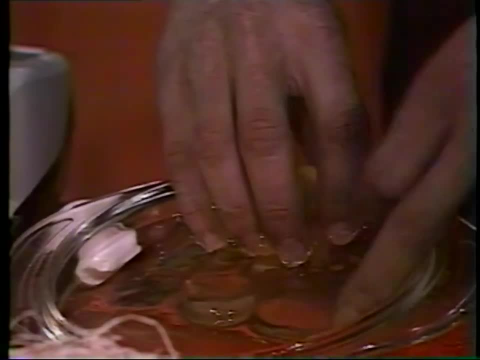 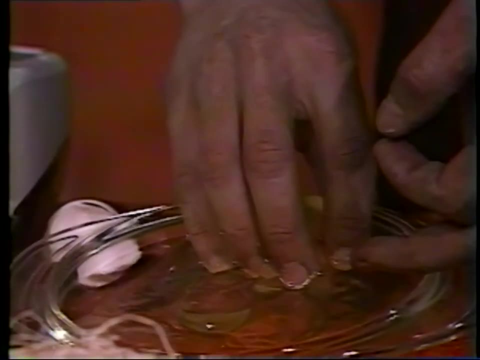 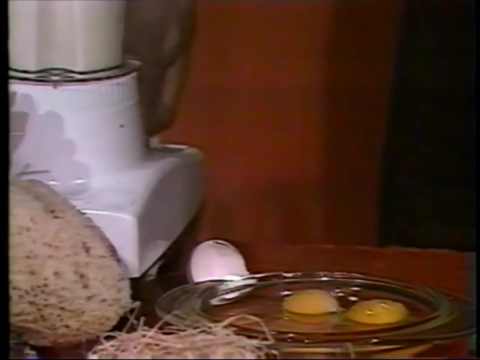 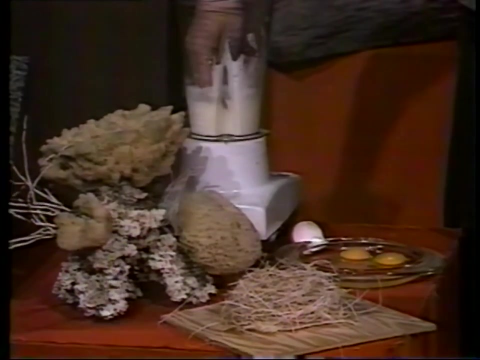 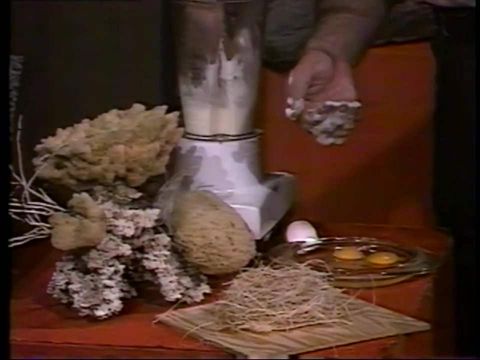 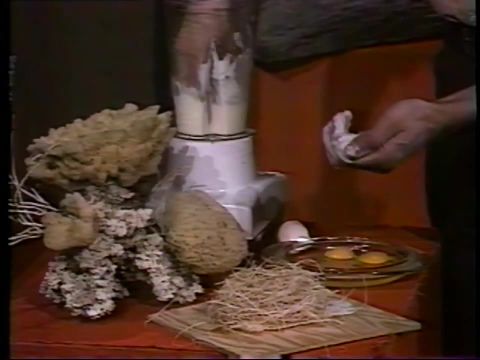 it egg white, any kind of shape as it flops around in the basin there. So a single-celled organism hadn't got any opportunity to build itself into any kind of efficient shape. But if we add a little instant evolution, we have, for instance, a multicellular material. 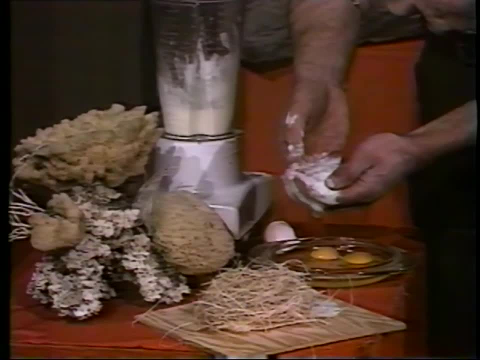 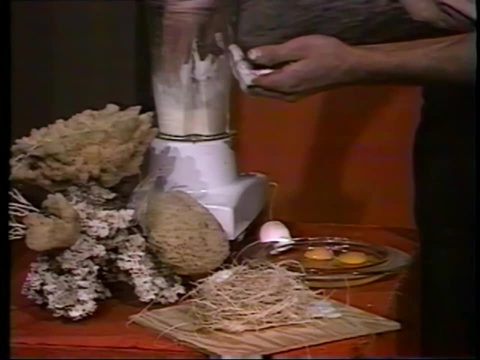 which we can encourage, which will take a shape. Now it should have been a bit colder and it would have peaked like a meringue And we could have molded it into some kind of shape, particularly so it's a little bit more flexible. 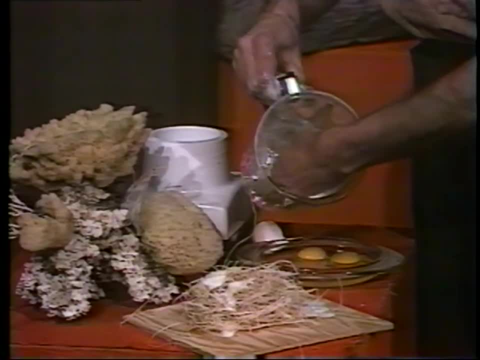 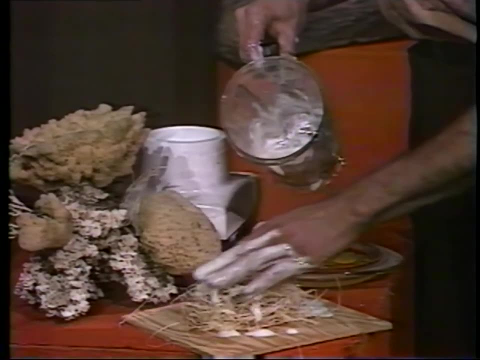 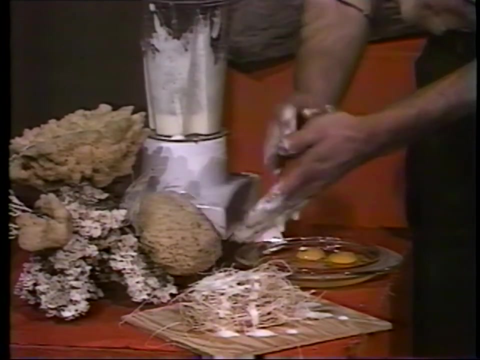 as we're getting closer to the end of the brain. But we can look at the structure of a single-celled organism and see how it's going to change. And then we can look at the structure of the egg whites, And each of the bubbles of the egg white represents a cell. 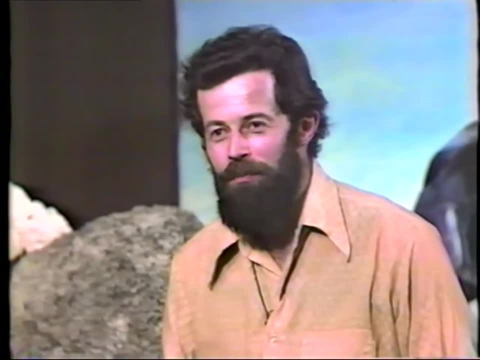 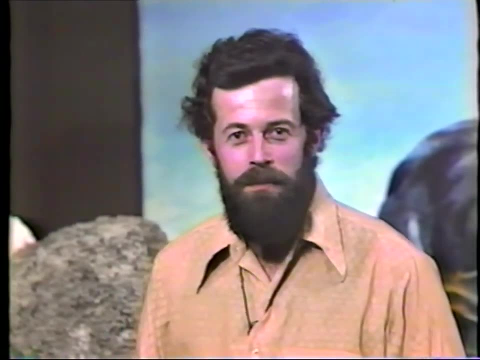 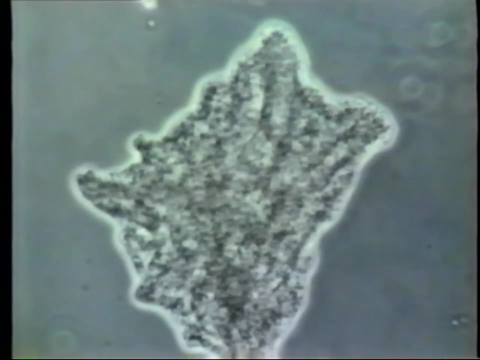 And that kind of structure. it looks a little messy there, I'm afraid, But that kind of structure is what the sponges adopted organisms and the multi-celled sponges. The simple single-celled mode of animal life is typified by 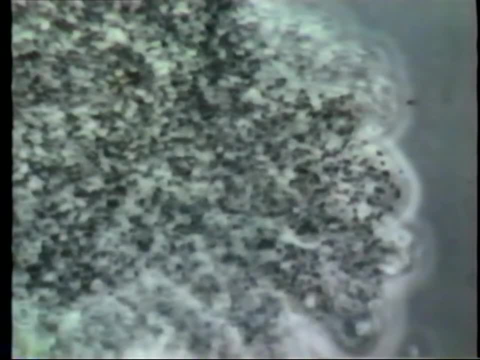 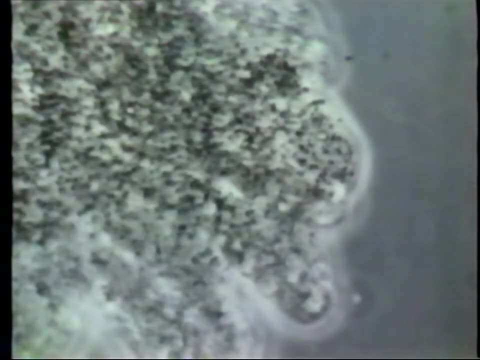 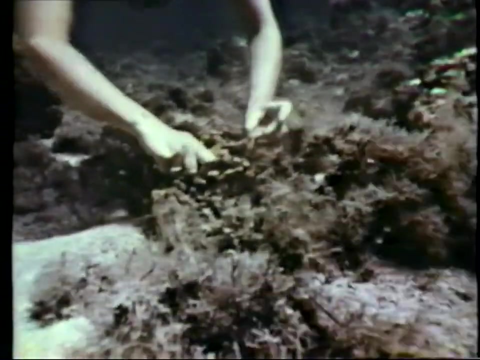 this amoeba, which probably has the same character and lifestyle as its primitive Precambrian ancestors. Like the free egg white, it consists of a single mass of protoplasm contained within one cell wall. Sponges, on the other hand, which grow on the sea floor and are also animals. 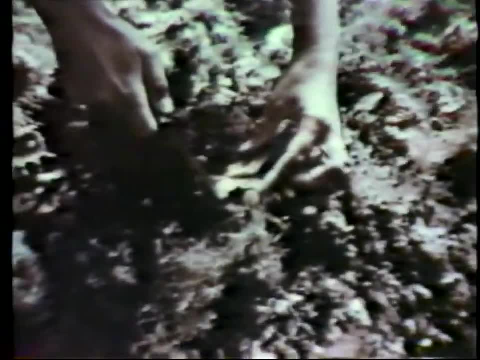 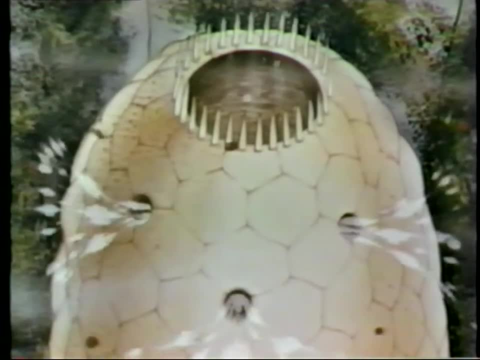 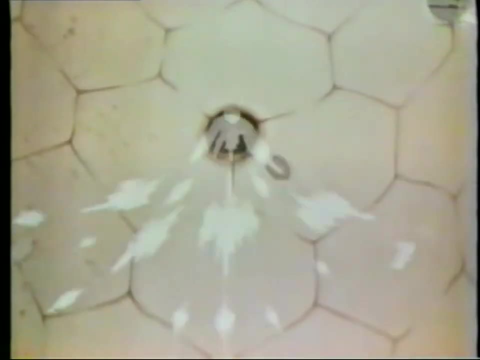 but can be cut without apparently any reaction, employ a multi-cellular form of life. This is a sponge with a hollow structure. Water enters through microscopic pores in the wall of the sponge and food particles are filtered out before the water comes out of the top. 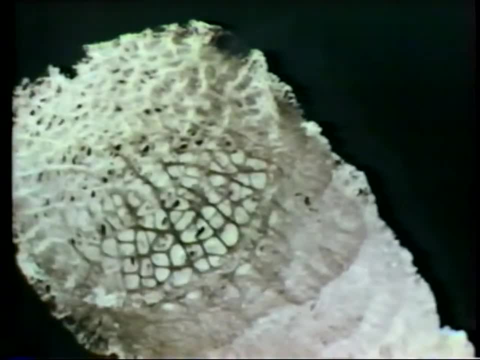 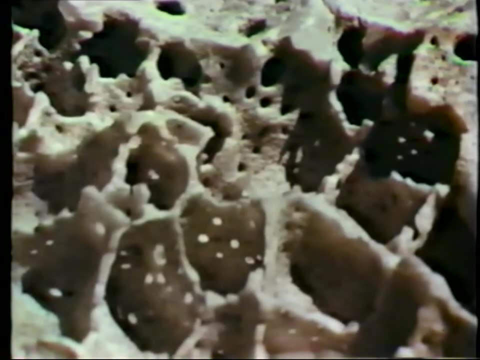 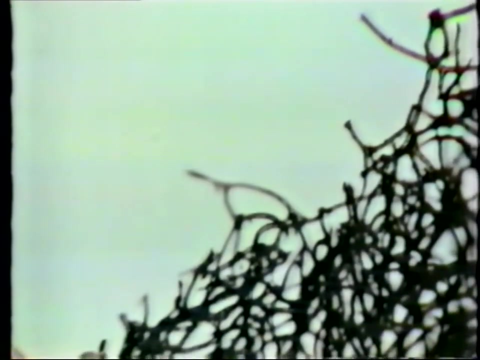 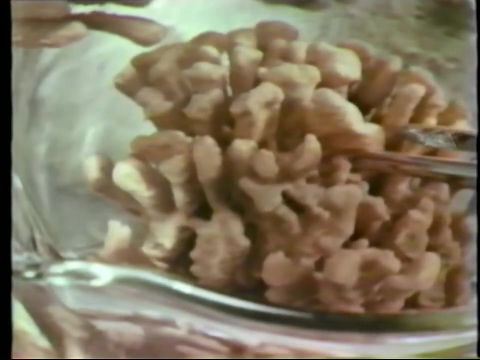 of the sponge. As well as being multi-cellular, the sponge has a supporting structure, in this case spongin, which is the material that you have for use in the bathtub. The spongin forms quite a complicated network on which the many cells of the sponge are supported, Although it's a primitive animal sponges. 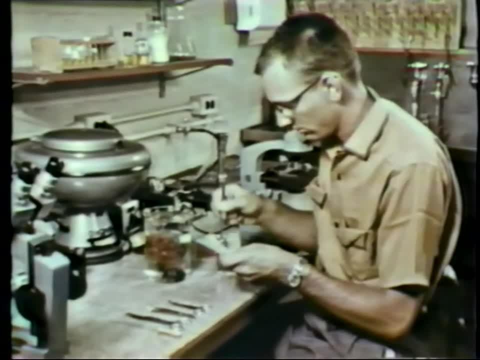 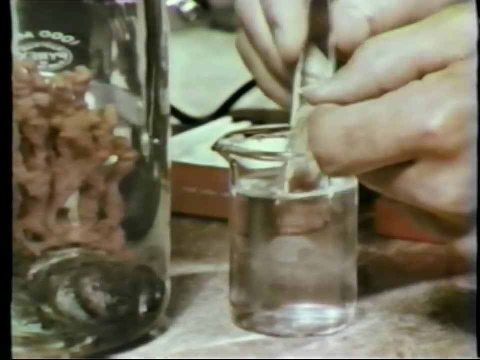 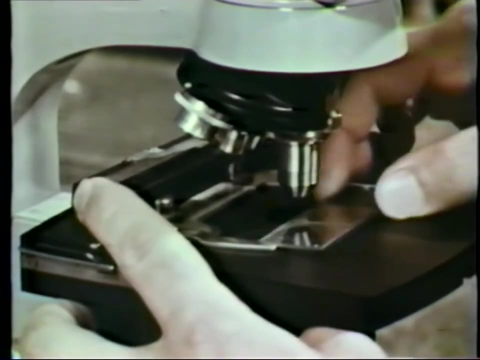 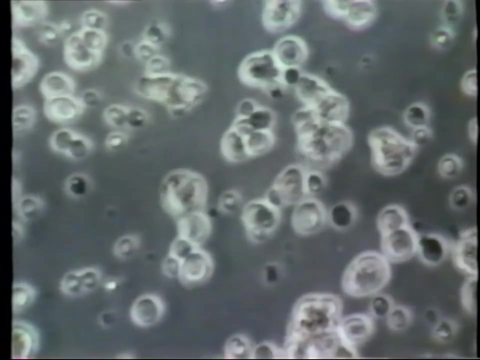 have a very peculiar property which can be investigated in the laboratory using a piece of living sponge and squeezing it, through a fragment of silk, into the seawater. The cells of the sponge have been broken away from the skeletal support and lie free in the seawater. They 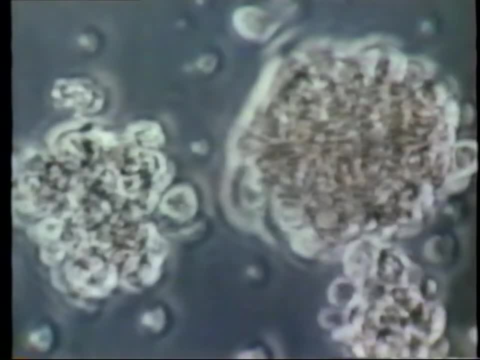 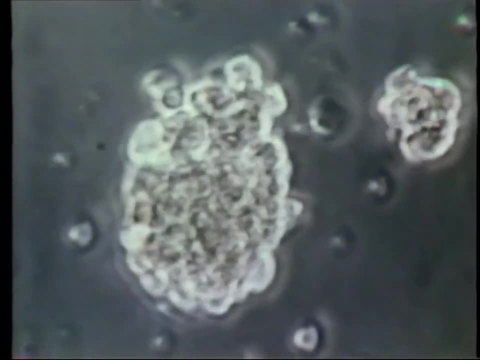 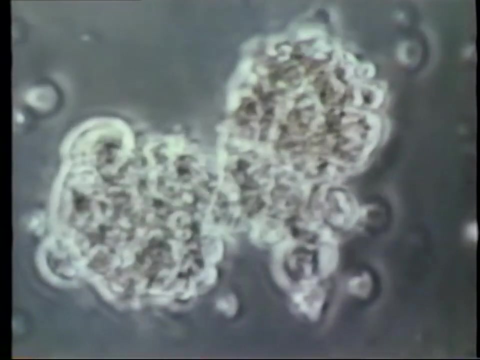 seem to be moving about at random, but this time-lapse photography shows that in fact, they're forming into groups And smaller groups are joining larger groups And the larger groups are joining together and after about two weeks, in fact, in place of the groups of sponges. 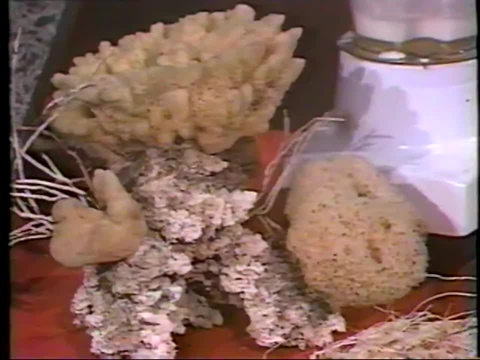 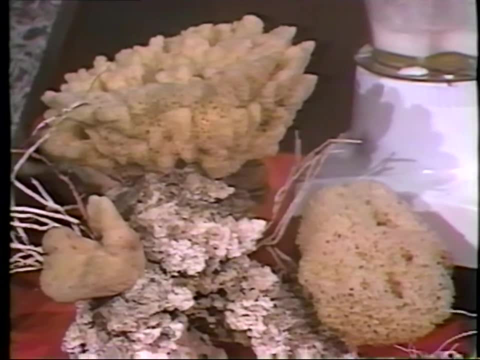 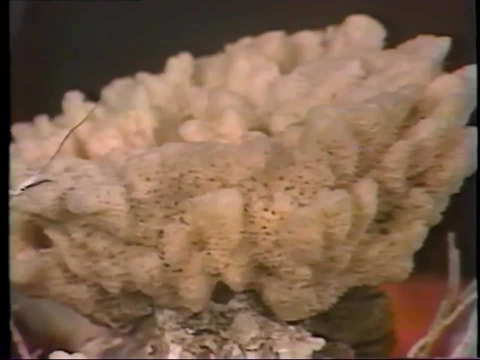 one has new sponge animals. The light brown sponges on this specimen are the skeletons on which the many cells of the sponge were arranged. They're bath sponges. The sponges are something of an offshoot and they don't belong in the 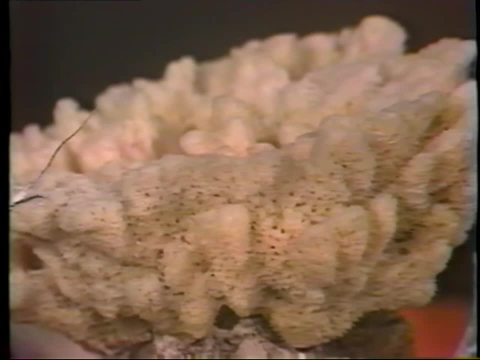 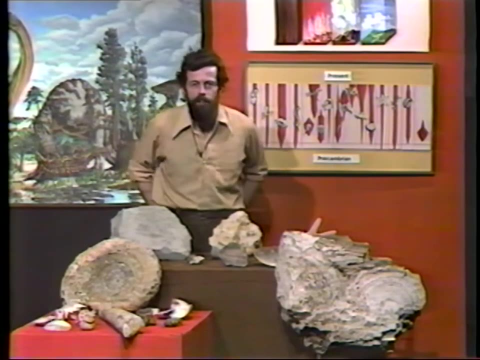 main line of development of animal life, But nevertheless they're obviously a very interesting organism. Now, the great step from the Ediacara fauna to the- to the Ediacara fauna, I'm sorry- was a very important one for animals. The next very important one we see in the Cambrian. 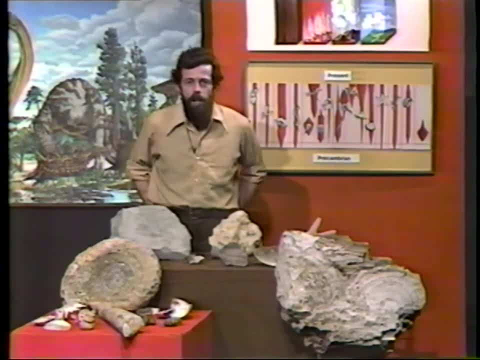 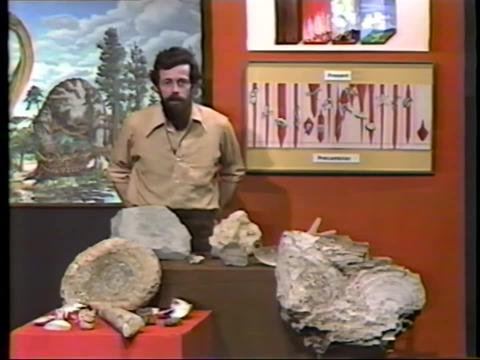 And that step is the development of hard parts of calcium carbonate, shells, for example, in which the soft bodies of organisms were encased. There are other kinds of skeletons developed at that time, also not all calcium carbonate. There are still, however, places where we find soft-bodied Cambrian organisms. 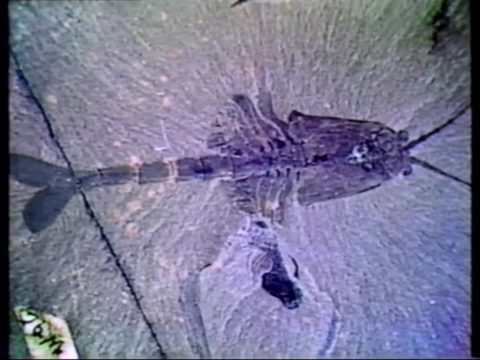 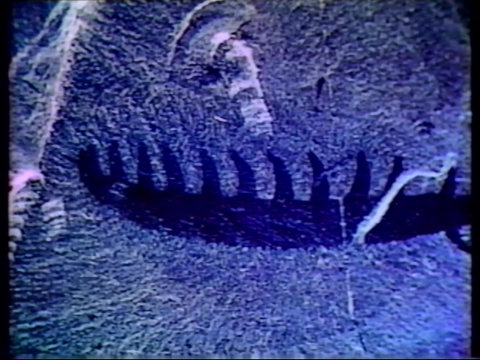 One of the most famous places is in Canada, in fact in British Columbia, where the so-called Burgess Shale near Field has yielded about 35,000 specimens since the beginning of the century, most of which are of soft-bodied organisms related to worms and quite a variety of organisms much more developed than Ediacara. 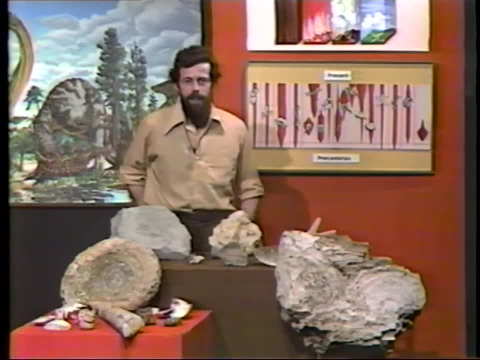 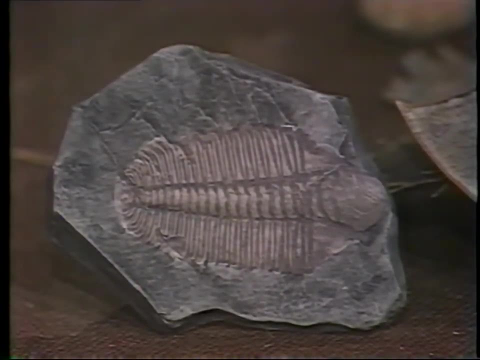 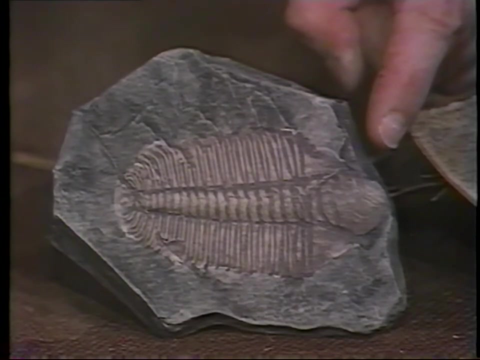 One of the principal fossils in the Cambrian, that is, about 600 years ago, is the Trilobites like this one here. They're usually about the size of this one, in other words, a few inches long, and they're clearly divided into a head, which is, at this end, the main part of the body. 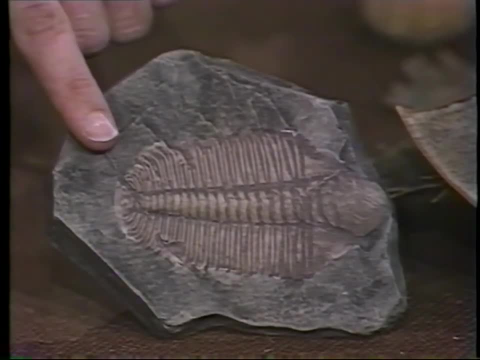 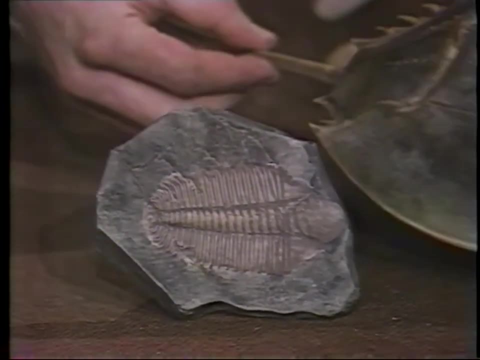 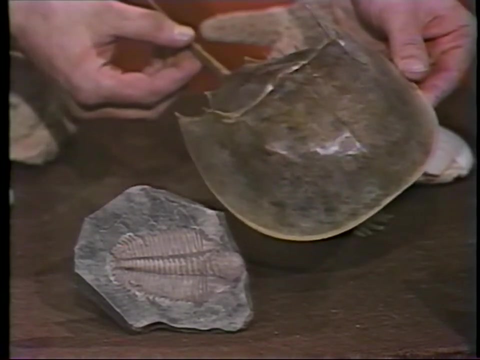 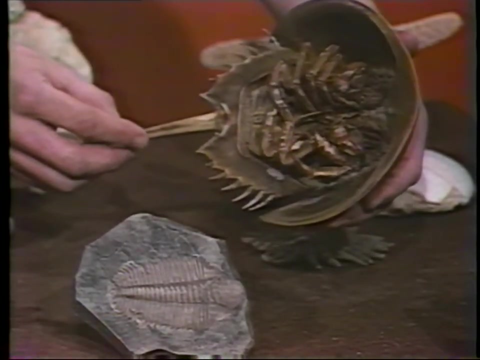 and then a tail. at this end, Three parts and therefore Trilobite, And one of their Well, not direct but fairly close present-day relatives are the Horseshoe Crabs. This is a Horseshoe Crab from Florida and underneath are the legs, rather similar to the Trilobites. 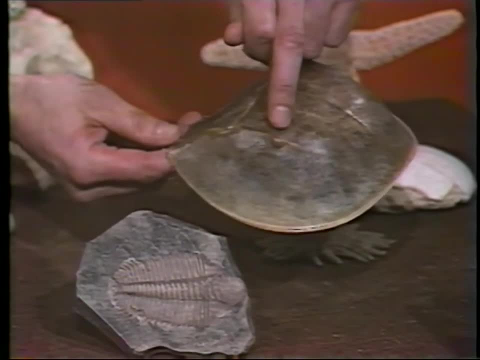 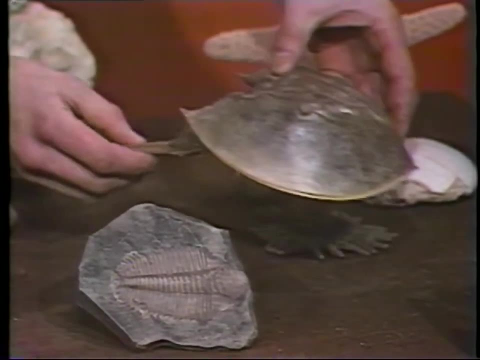 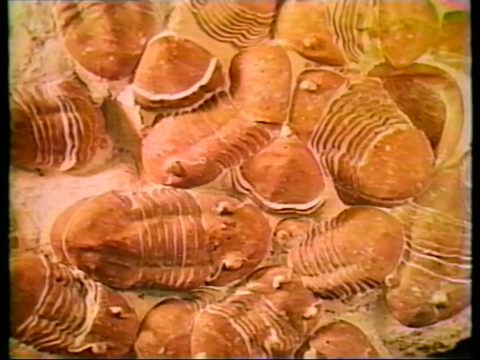 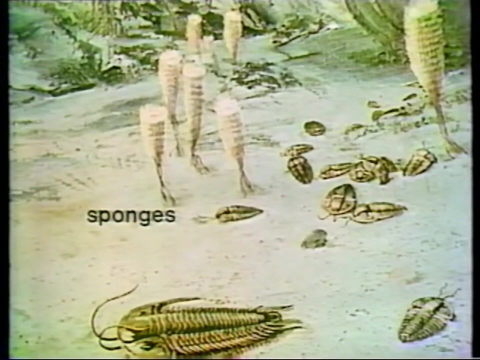 Here is the eye of the Horseshoe Crab. The eye of the Trilobite is down here, and some of them had extremely good eyes. Now the Trilobites are crawling organisms And let's have a look at a variety of those Trilobites. 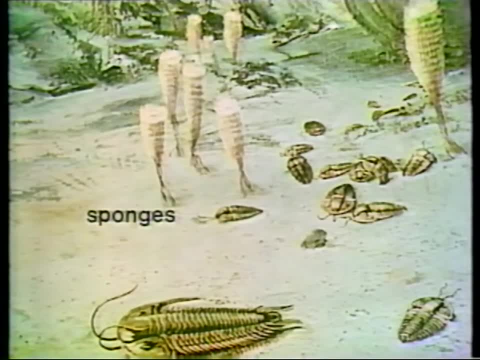 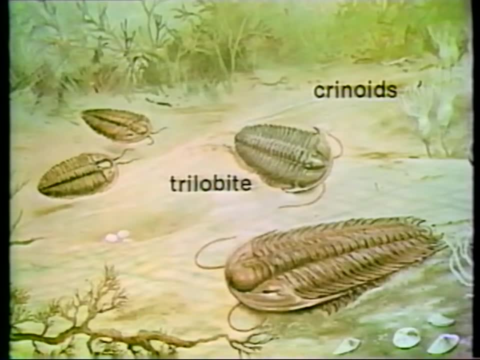 Here they are crawling on the seafloor, Sponges growing up from the seafloor- a typical Cambrian sea bottom, And here is a Trilobite on the seafloor. Here it is. Here is a Trilobite on the seafloor. 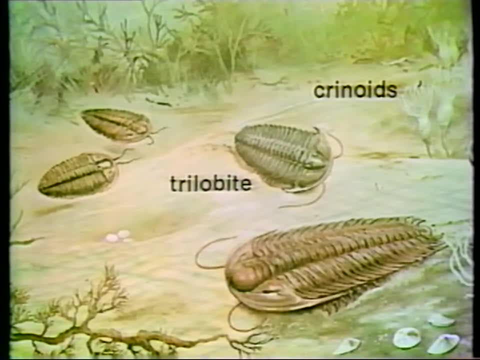 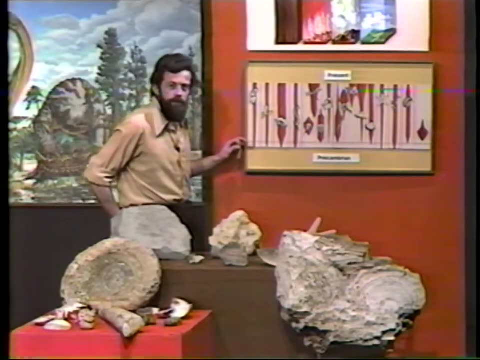 And here is the Trilobite on the seafloor. And here is the Trilobite on the seafloor are further trilobites. Now let's summarize the kinds of organisms that we've seen so far in the fossils that we've looked at. 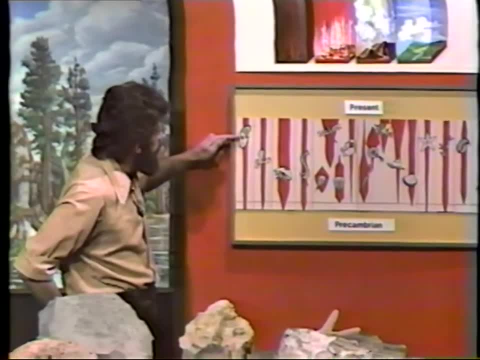 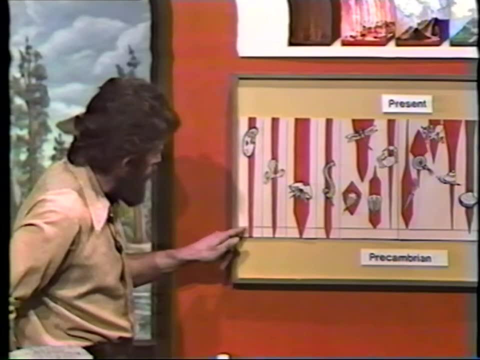 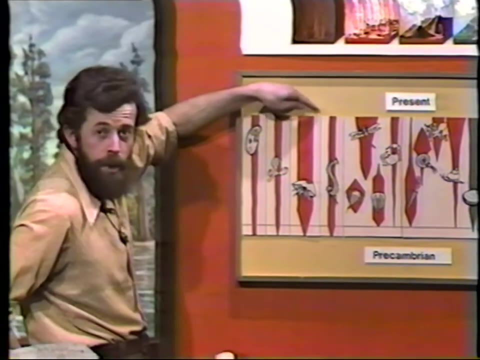 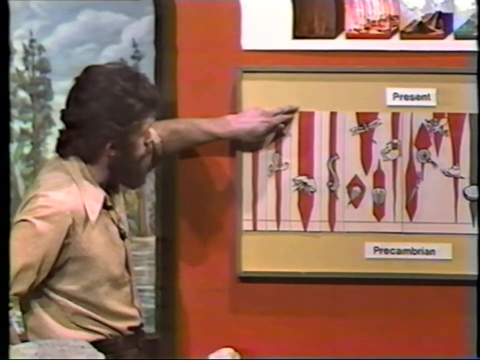 The table here with the red column indicates how long an organism existed. This bottom line represents the beginning of the Precambrian And the top represents the present. So if an organism is marked by a continuous red stripe, then it's been present from the Precambrian. 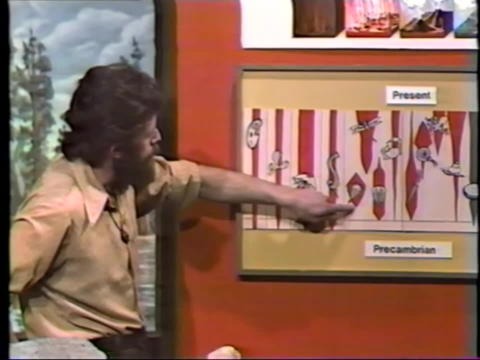 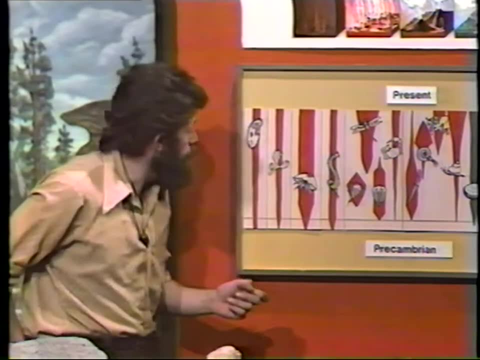 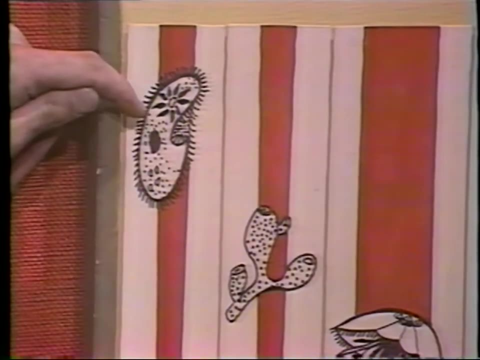 right to the present day. If it's just marked by a patch of red that begins and ends, then the organism is now extinct. The protozoa, The single-celled organisms, the primitive ones that we found in the Precambrian- 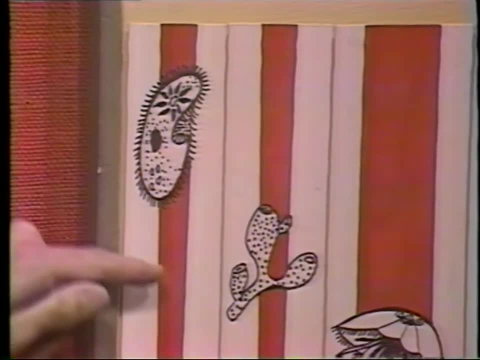 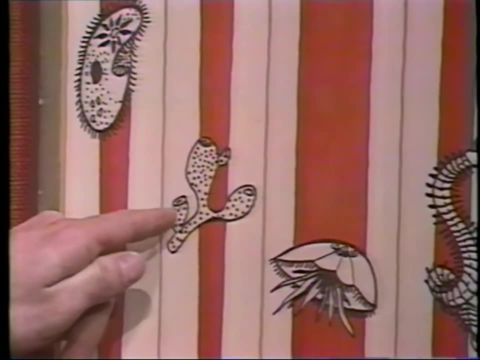 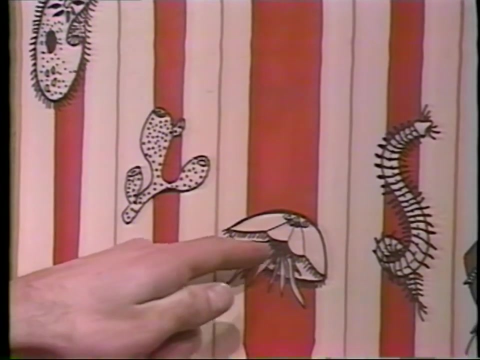 for example at Bitter Springs, are still with us today. So are the sponges which appear in the Precambrian. So are the jellyfish, which we saw at Ediacara. So are the worms, which we also saw at Ediacara. 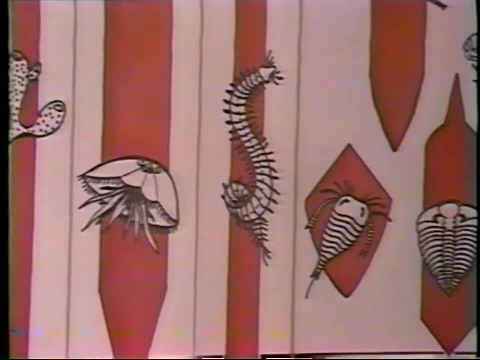 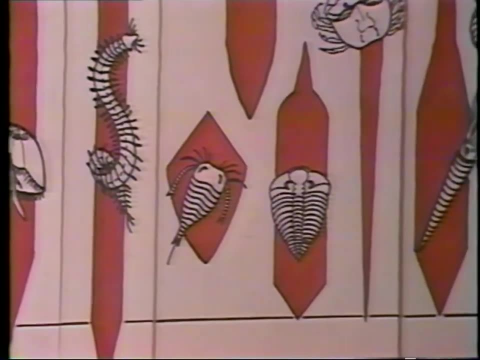 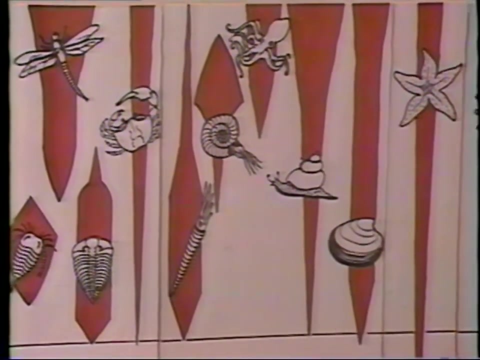 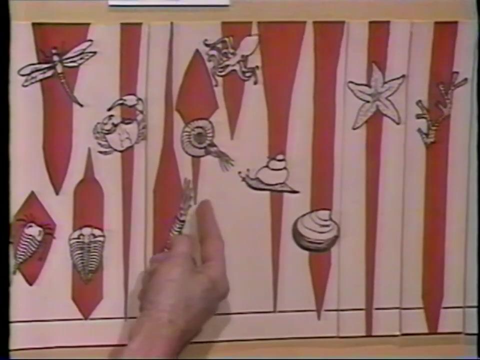 And the trilobites begin just about at the Cambrian. Now, all of those organisms are organisms that appeared in very early faunas, The mollusks which we know today from, for example, the octopus and the snail. And the And the Clams began to appear at just about the beginning of Cambrian time to join those organisms, those relatively primitive ones that we've just spoken of. Let's have a look at the character of the mollusks. These are all mollusks. 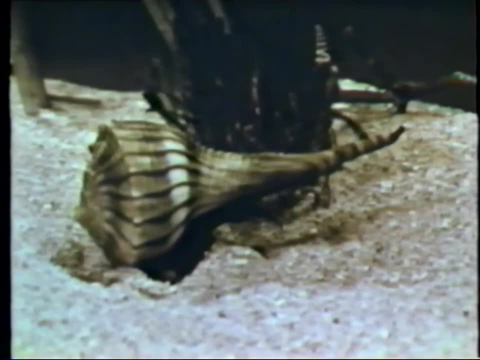 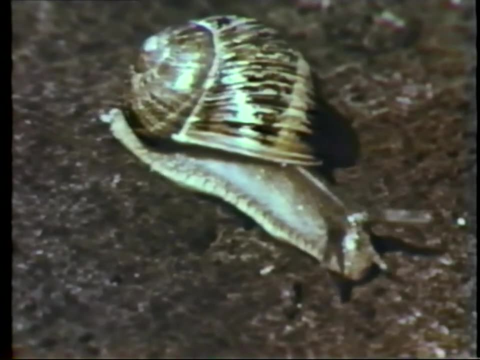 Most mollusks have a calcium carbonate shell in which the soft body of the animal is housed. The part which protrudes from the shell is largely the foot, although at the end of the foot, in the snail, is obviously the head. Here, from underneath, the mouth is 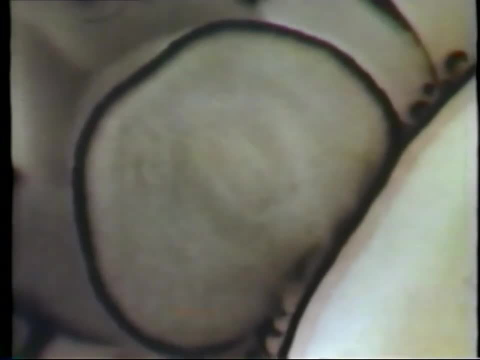 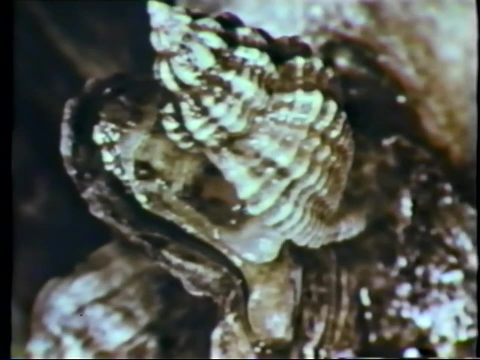 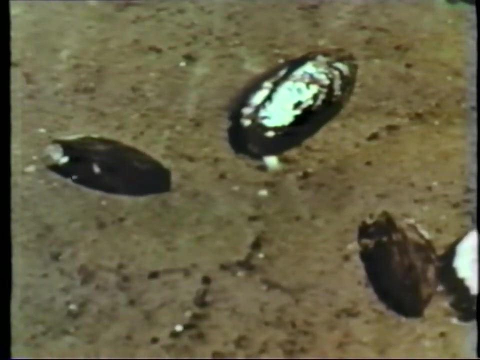 at the top left of the screen, And it's equipped with a rasping organ which the snail can use to rasp its way through shells of, for example, in this case, an oyster- in order to eat the contents, The clam uses it. 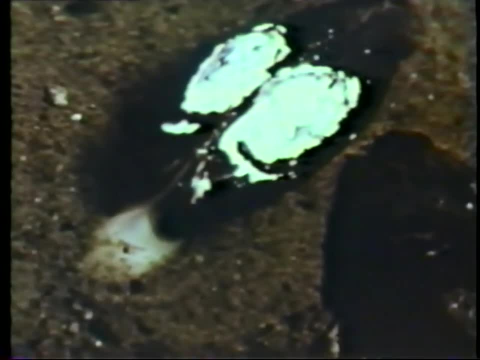 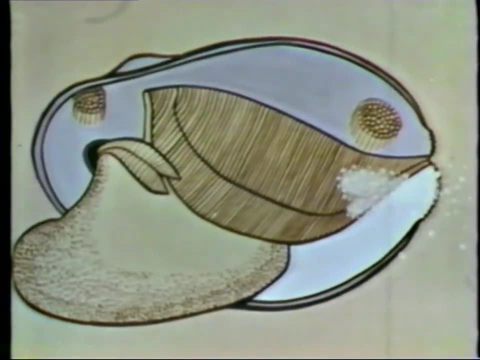 It uses its foot to dig into sand quite often And once it's in there, the clam feeds by filtering water between its shells. The food particles are filtered out of the water which comes into the shell by the gills, So the clam is a filter feeder. 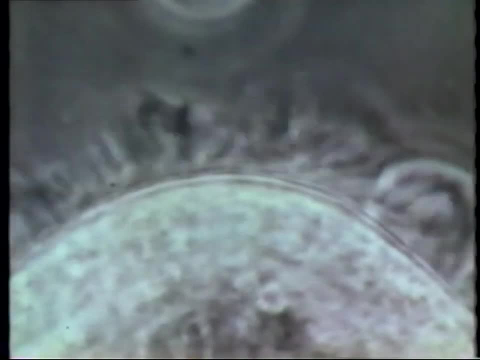 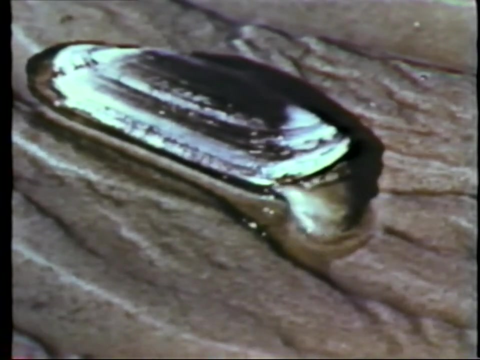 The particles of food move eventually to the mouth and are driven there by little cilia or whip-like structures which carry the microscopic food particles along. The pulsing of the foot is driving this clam into the sand- a very good device for protecting yourself from predators. 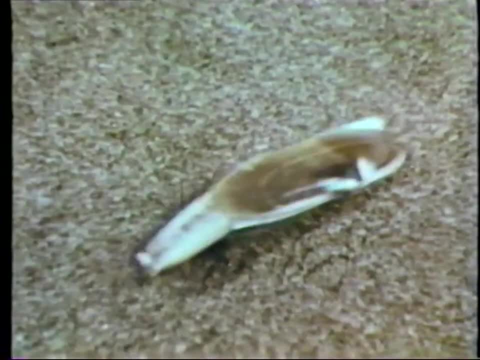 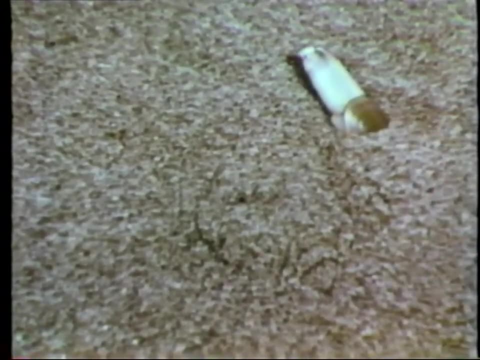 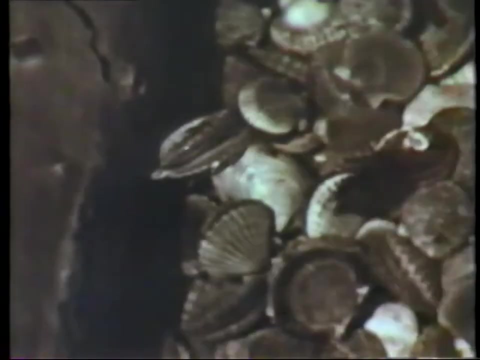 if you're a clam on a beach. Water is being emitted from the siphon of this clam as it digs itself in. The pectin, which is also a clam, can propel itself through the water for short distances by clapping its valves together. 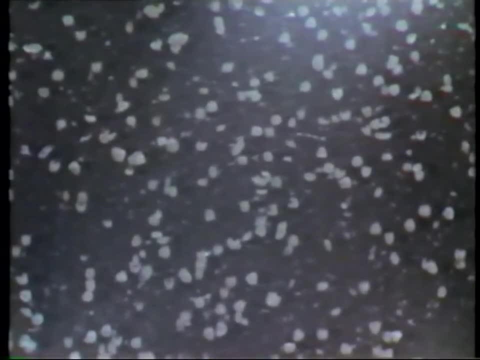 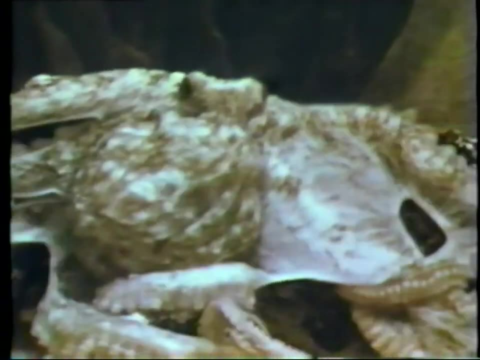 Mollusks reproduce by means of eggs and larvae, all of which are, of course, very small and light and can be carried large distances by favorable ocean currents. The octopus is a member of another kind of group of mollusks. 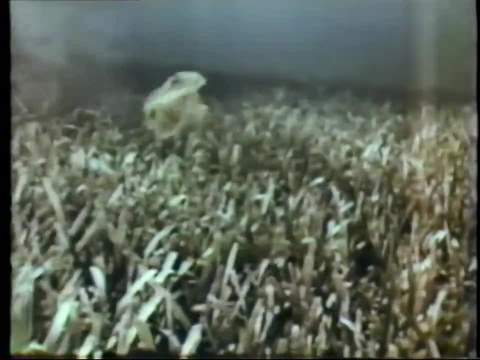 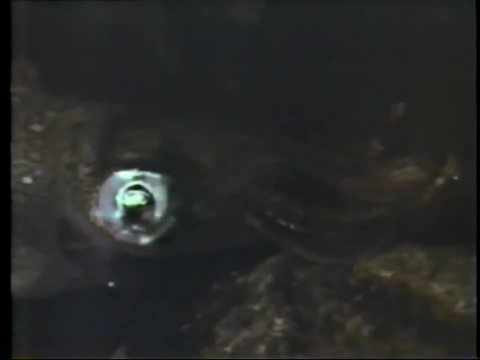 It's related to this. It's related to this, It's related to the squids, And they're called cephalopods because the head, with its large eye, lies at the base of the foot, which is divided into tentacles. In the case of the squid, there are 10 tentacles Here. they're propelling themselves along by ejecting water in a jet-like fashion. The octopus has got eight tentacles And they're equipped with suckers, which are very good for getting hold of prey. 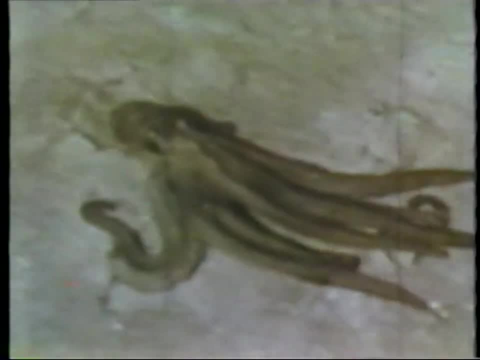 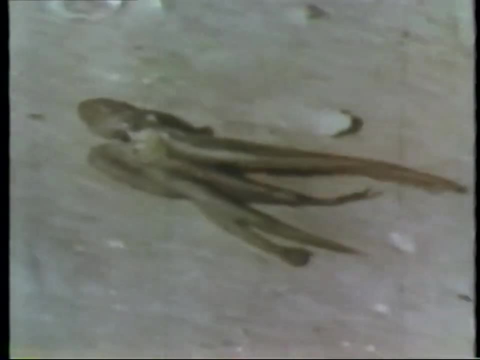 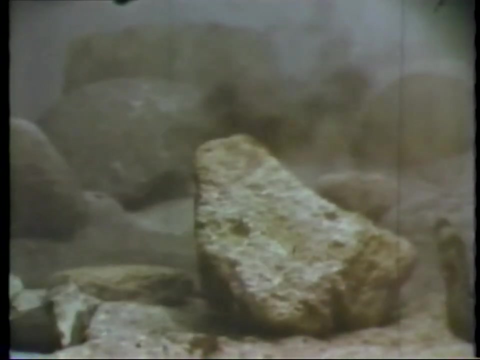 and holding on to food. The octopus can move its tentacles in order to move itself through the water too. For protection, the octopus can extrude an inky fluid. The mollusks show just about every different way of living in the sea. 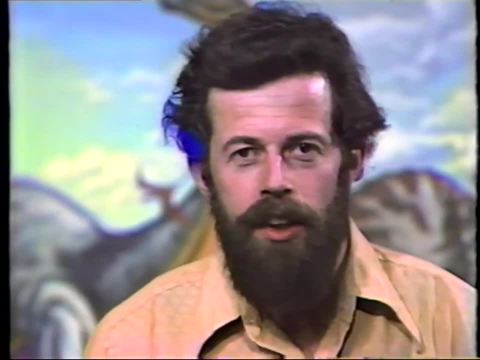 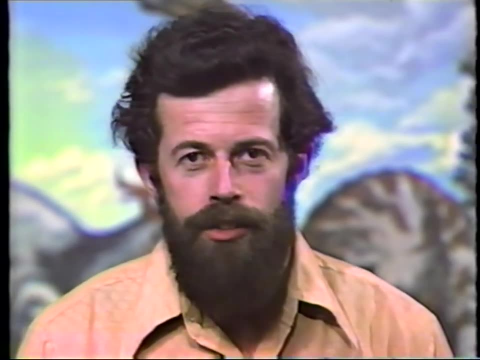 Let's just review them quickly. Remember the snails, or the gastropods as they're called. They're the most common species of mollusks in the world And they're called cephalopods. They're called the snails. 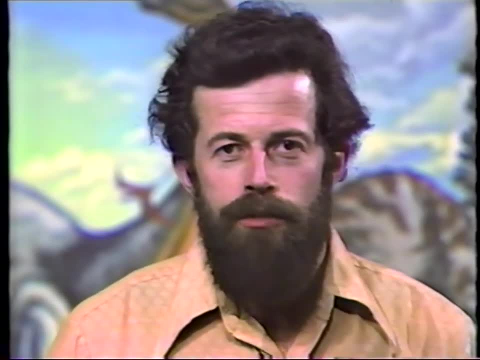 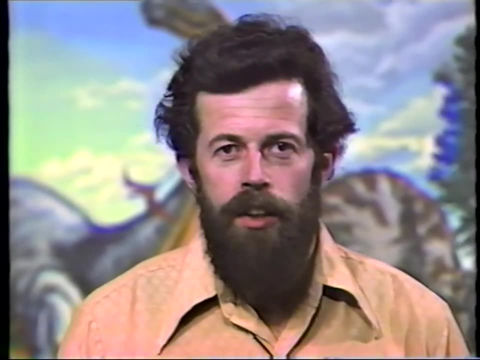 They're called the snails. They're called the snails. The snails live in two different ways. Those with the radula that grind through the shells of oysters, for example, are carnivores. They eat the flesh of the oyster because they 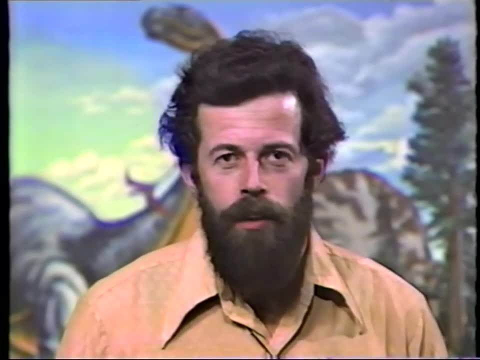 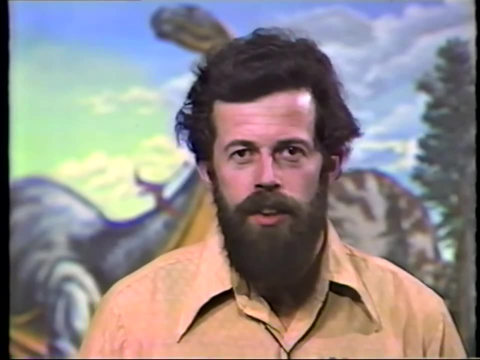 have a good, efficient radula, a good, efficient, tooth-like organism for grinding through the shell. Those that don't have that tend to eat the flesh of the oysters, or those that don't eat the flesh of the oysters are called the sea snails. 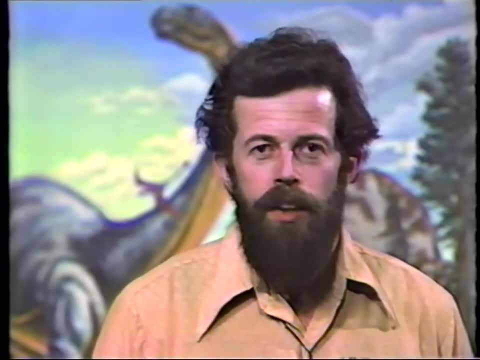 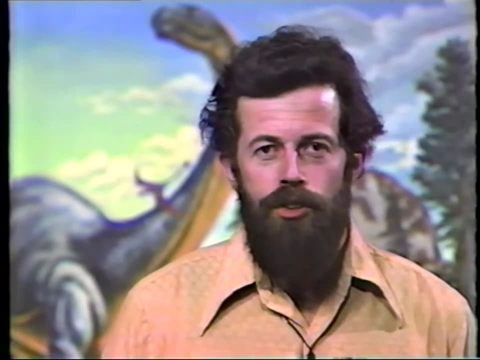 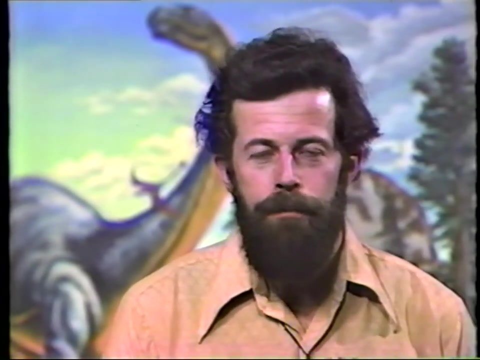 And they're called sea snails because they can feed on the water from the sea floor. They're what we call deposit feeders. They feed on the deposits on the sea floor, Then the clams, or the bivalves as we call them. 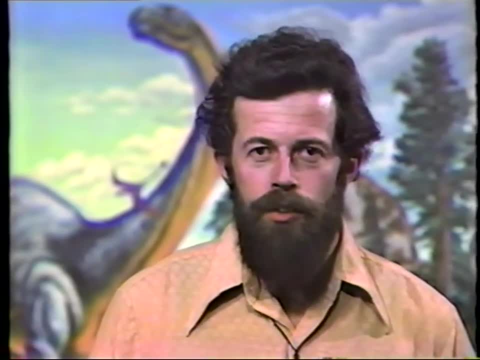 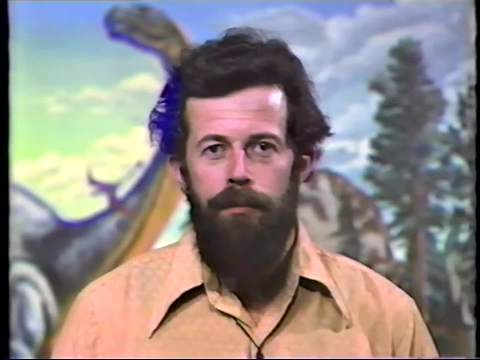 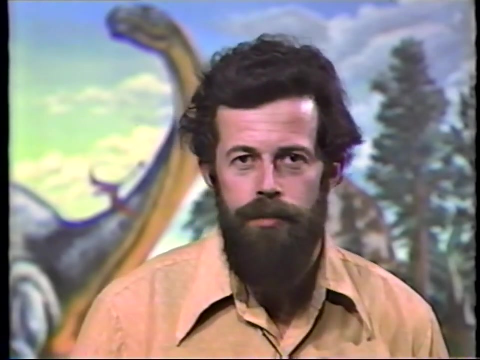 those mollusks that have two shells that join together, that they then pass to their mouth using the gills. so the clams are filter feeders. yet a third different kind of way of life that the mollusks have. then think of the octopus. 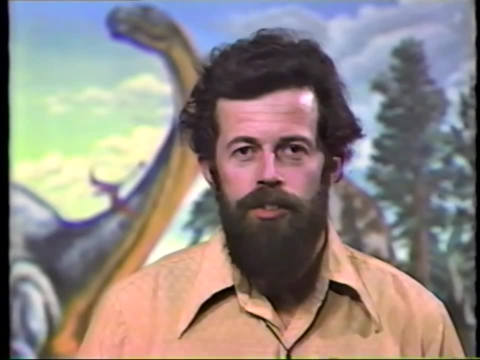 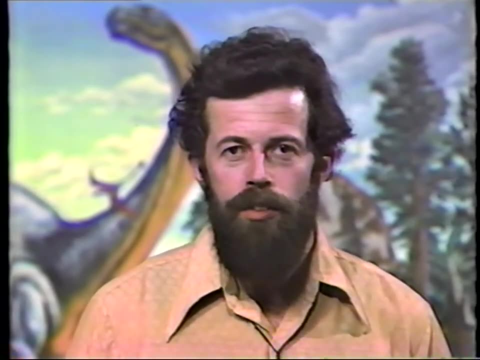 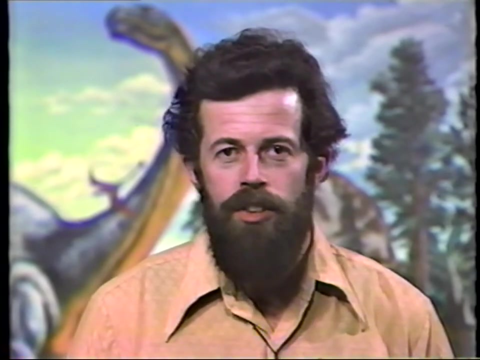 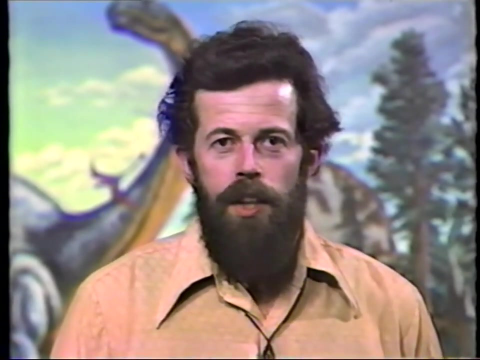 and also the squids. the octopus and the squids have tentacles which they use for capturing prey, such as crabs in the case of the octopus, which they then eat. so the, the cephalopods as they're called, with the tentacles are carnivores- again carnivores of mobile organisms, and the, the squids. 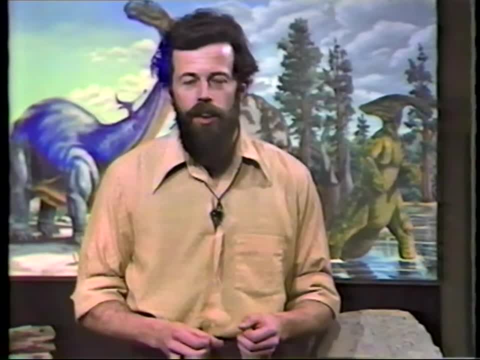 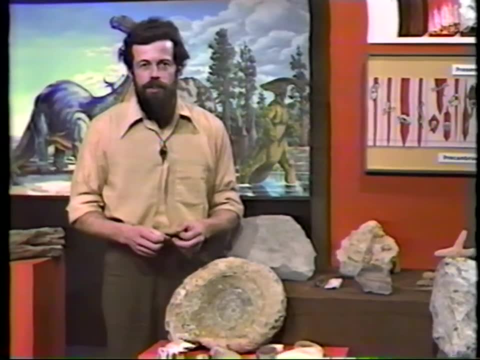 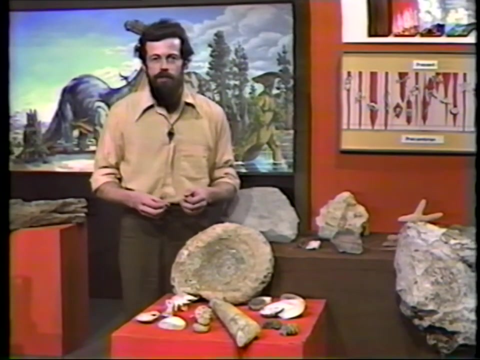 can swim, rather like fish, so they can capture organisms in the main body of the, the water, a very wide variety of different kinds of lifestyles. we say that the mollusks have radiated. they've adapted to very many different kinds of ways of life. they've radiated out from a simple organism to very many varieties. let's look at the. 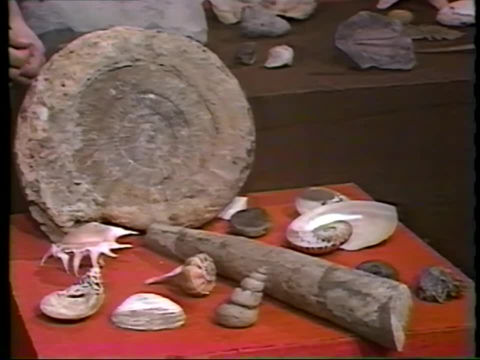 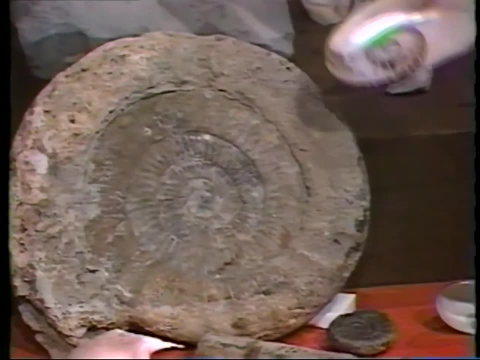 mollusks that we've got here in the studio and identify those different ways of life, of life. so the mollusks that we've got here in the studio, or the mollusks in the studio, are essentially more or less the ornithologist, are different kinds of life. 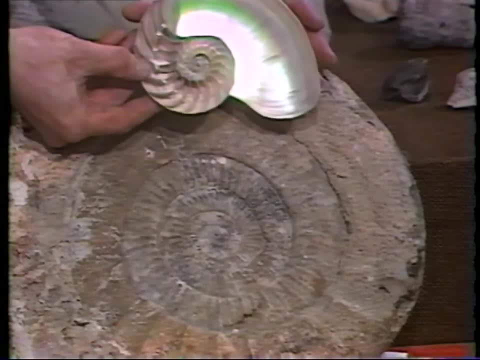 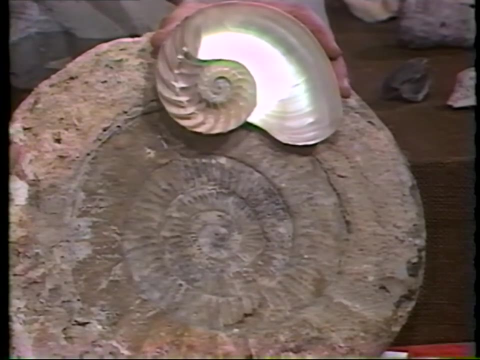 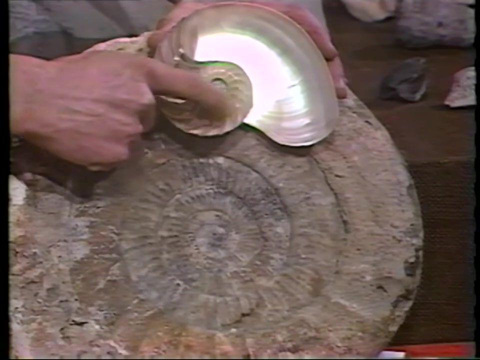 the cephalopods are typified by this very large coiled ammonite, as we call it. the internal structure can be shown by comparing that coiled shell with a recent relative that's been cut through, and here you can see that the shell consists of. 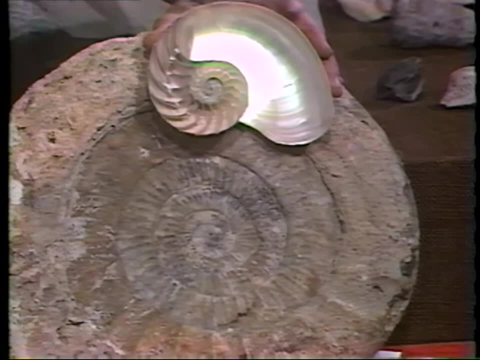 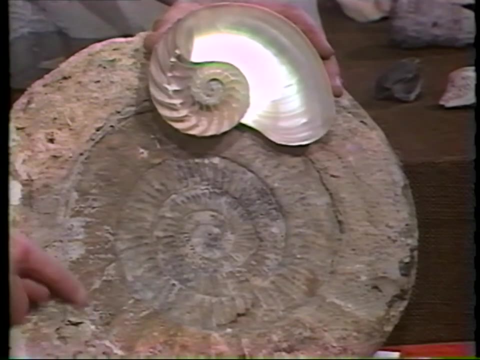 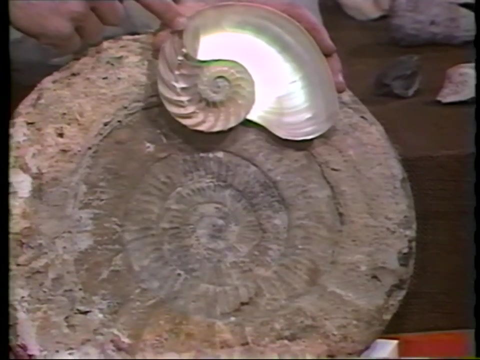 And it's in this last chamber, this one here, that the organism lives. So in this fossil example, the organism would have lived in this last part, here This is. this coil shell is related to the octopuses and the squids. 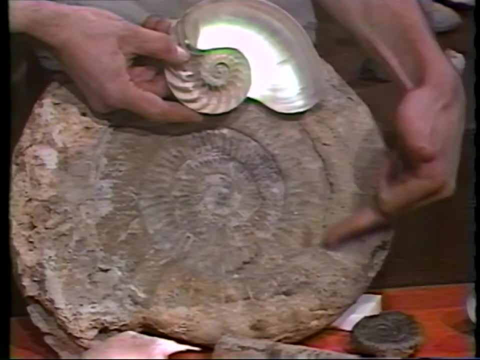 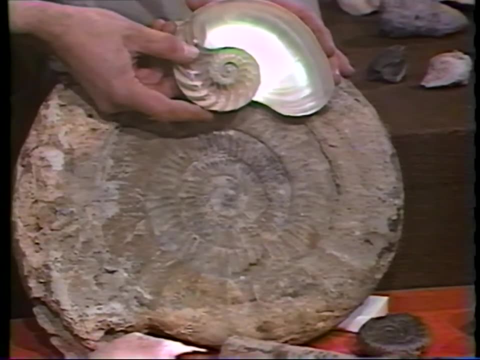 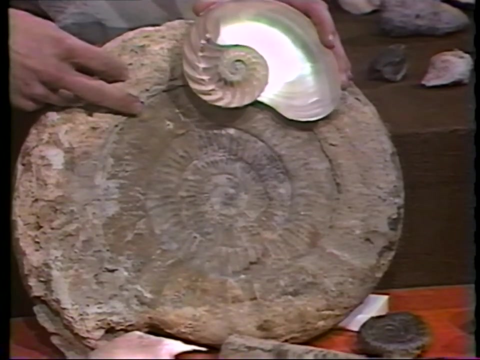 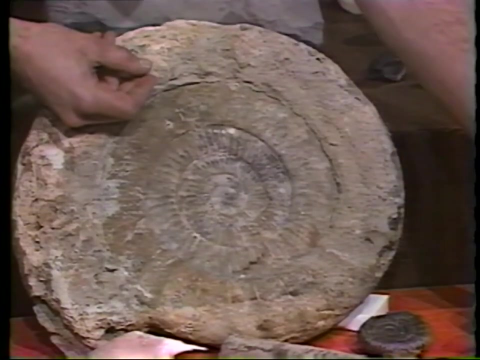 In other words, tentacles, emerged from here. The organism had an eye and it used those tentacles to catch prey that it could see. So these organisms, these mollusks, the cephalopods, are carnivores. They eat other organisms. 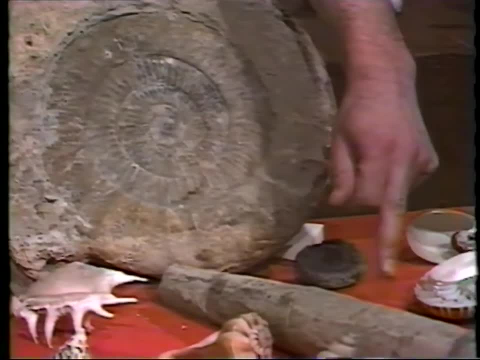 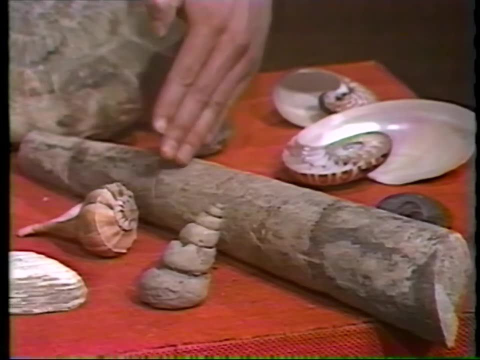 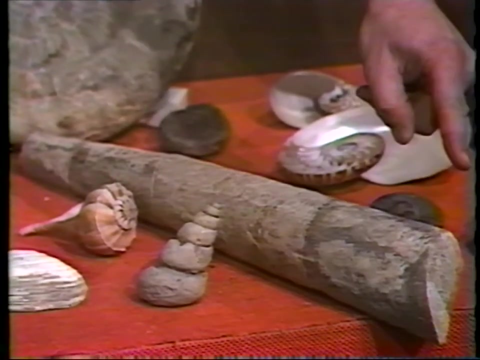 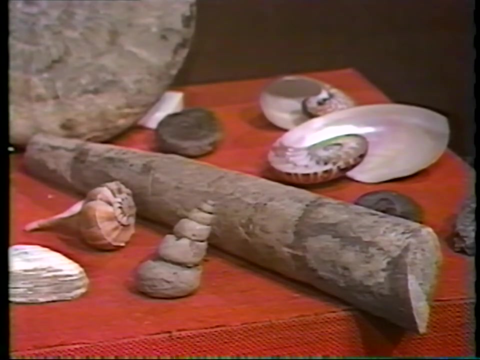 This is another cephalopod, a long straight one in this case, And the chambers run across Like this And the tentacles would have emerged out of this end, the far end. The chambers are filled with gas and they help to keep the cephalopod afloat. 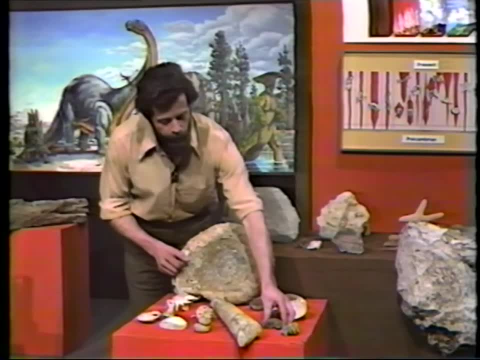 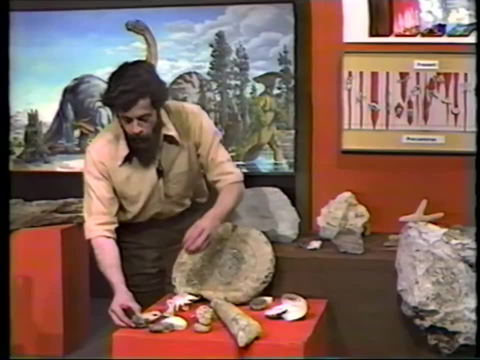 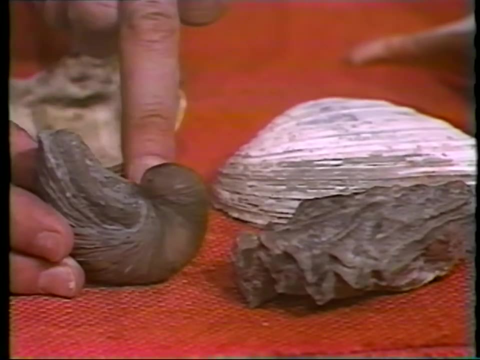 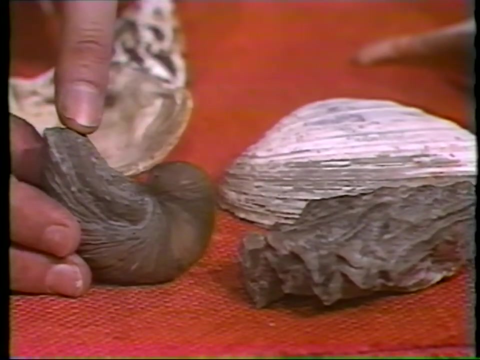 Now let's look at the bivalves, at the clams. Here are some. This is a falcon, A fossil oyster. Here is one shell, or valve as we call it. Here is the second, a smaller one. 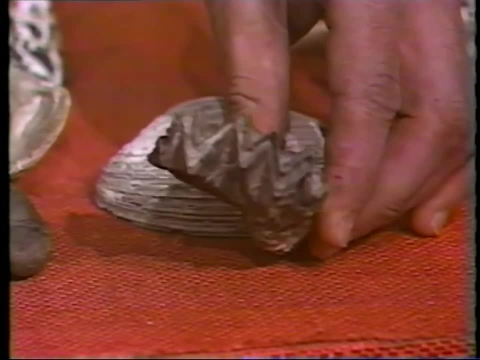 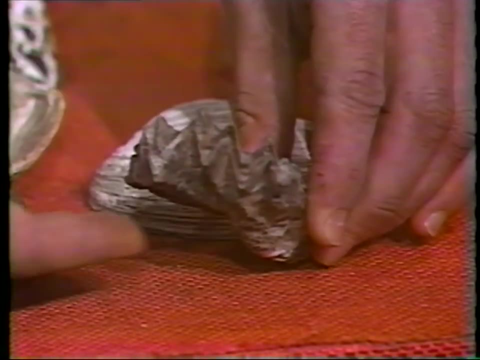 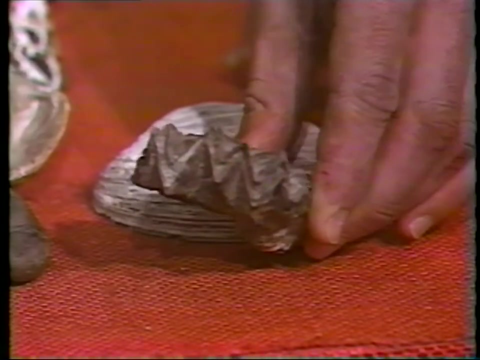 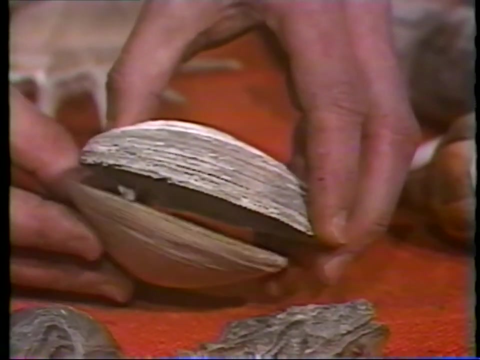 This is also a kind of oyster, And the shells fit together in a V fashion. Here is one shell, The other is there, And they would open and close like. so. Those are both fossils from Jurassic. These are also bivalves. 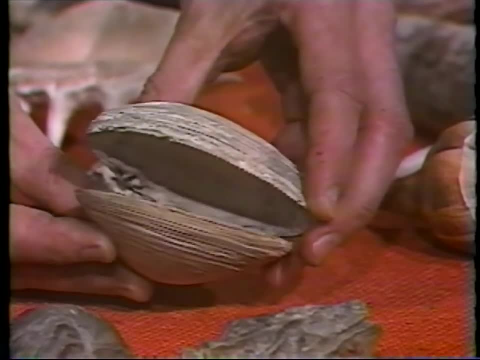 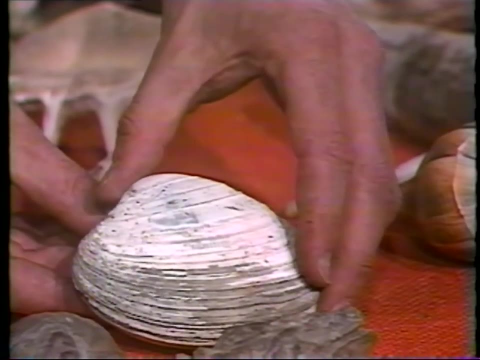 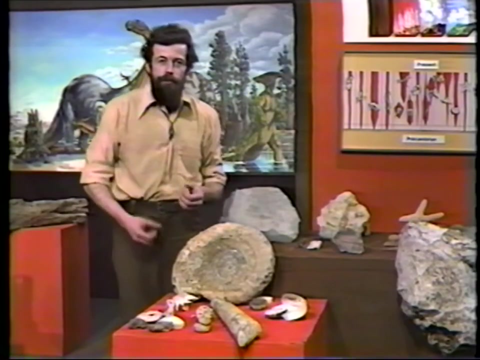 And if they were a good pair they'd fit together like. so. This bivalve might have buried itself in the sand like one of those that you've just seen and filtered the water. So those clams are filter feeders. They filter the water. 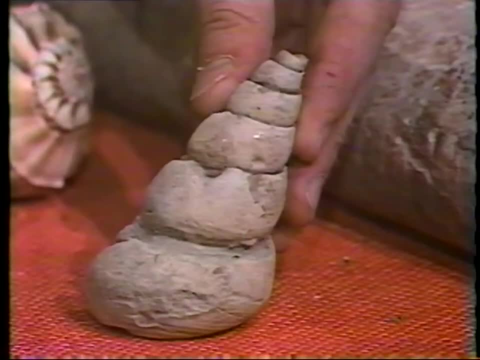 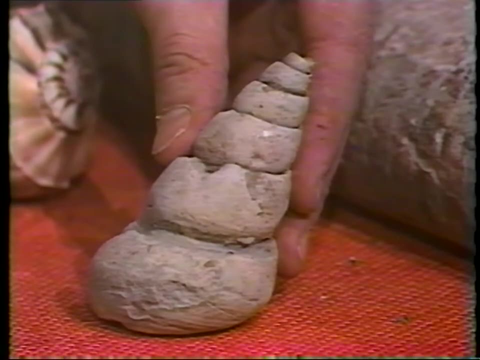 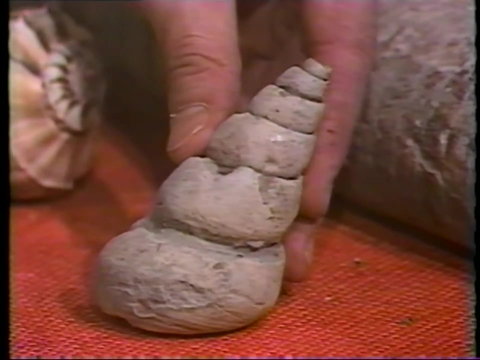 This gastropod, Gastropod or snail with the high tall spire, might have lived in one of two ways: It might have lived as a deposit feeder, eating the mud on the sea floor or the organic material in it, or it might have rasped its way through the shells of a clam. 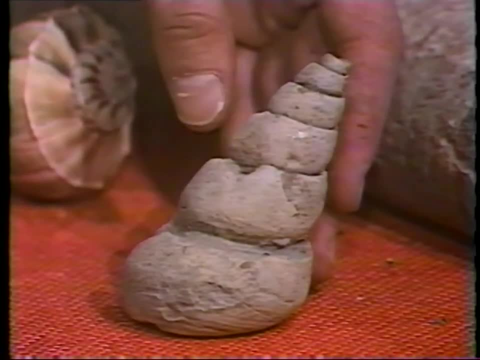 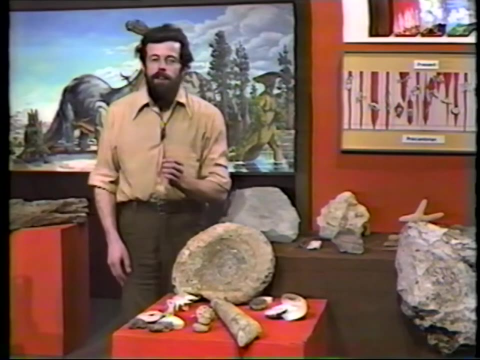 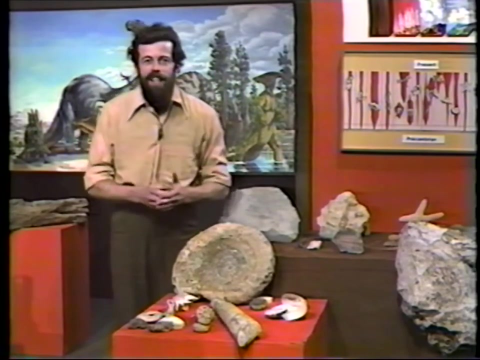 So it might have been a deposit feeder or a carnivore. We can't really tell just by looking at the fossil organism. Now then, What's of interest is to identify the kind of mollusk which first appeared in the Cambrian. Which of those different ways of life that the mollusks can lead? 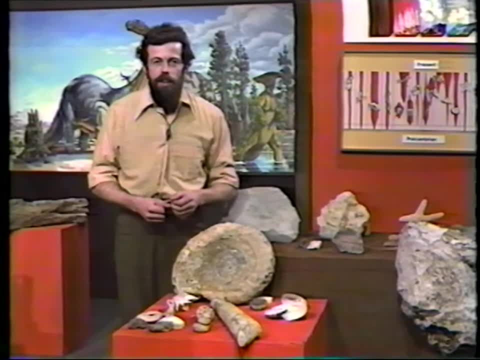 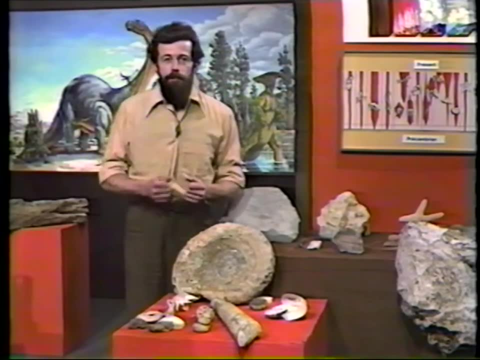 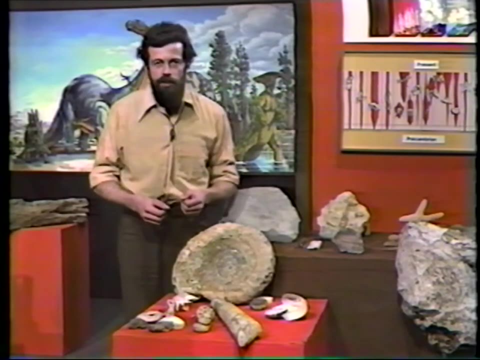 was led by those that appeared first in the Cambrian. Well, the ones which first appeared in the Cambrian were those which were deposit feeders. They were gastropods, dominantly the snails that crawled across the muddy sea floor and ate the mud or ate the organic material in the mud. 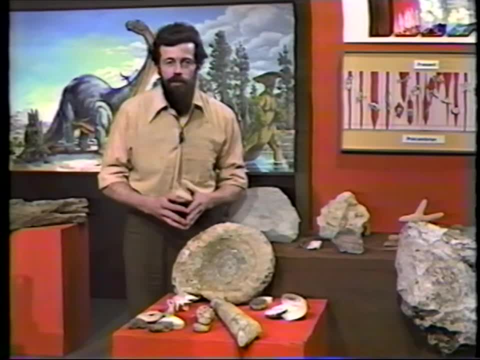 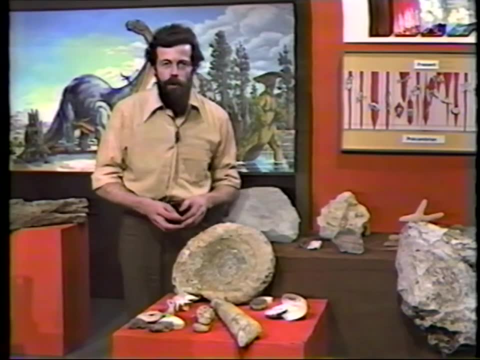 There were not very many filter feeder mollusks like the clams in the Cambrian or on the Cambrian sea floor. There were not very many carnivores. There were not very many of the octopus-like cephalopods with tentacles that captured moving prey. 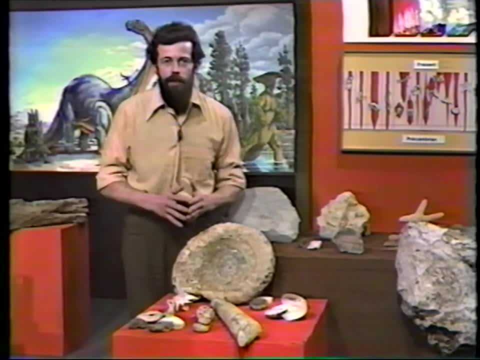 on the Cambrian sea floor. There were some, but not very many. Now, what does this tell us? Well, it seems to show that the Cambrian sea floor was dominated by organisms which were deposit feeders, By things like worms which crawled through the mud. 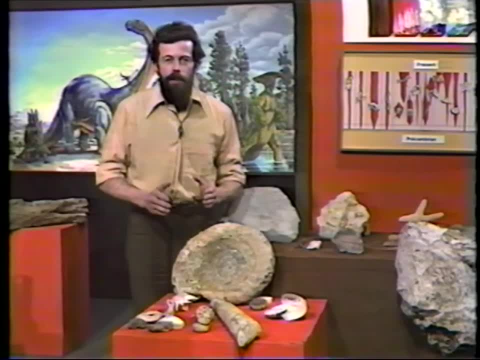 The Cambrian fauna is very similar to the Ediacara fauna, that pre-Cambrian collection of organisms that we showed you earlier. There also, the dominant organisms were deposit feeders. This is an interesting conclusion. It means that, although the organisms that we see in the Cambrian 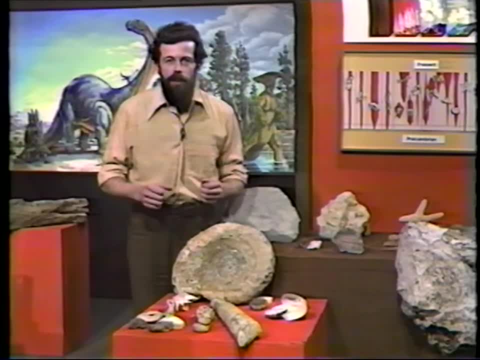 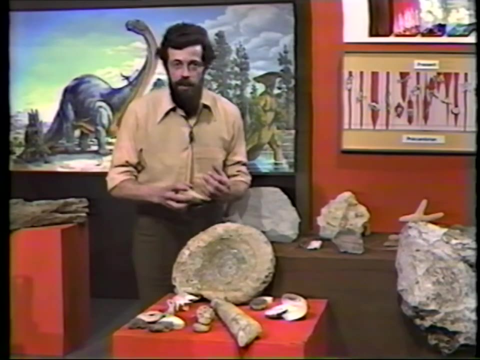 had suddenly developed skeletons of a kind calcium carbonate shell and, in the case of the trilobites, a kind of a horny material that's related to the kind of skeleton that beetles have. although these organisms developed skeletons, they were basically living the same kind of life. 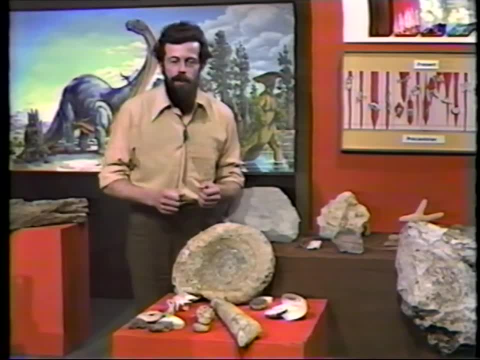 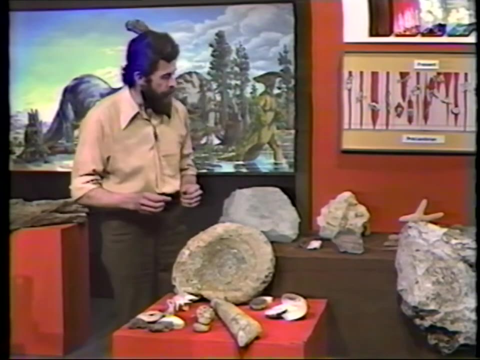 as the multi-celled pre-Cambrian organisms. Now that didn't continue, because later on in the Ordovician we see the advent of different kinds of organisms. Let's have a look at some of those Succeeding the Cambrian in the Ordovician. 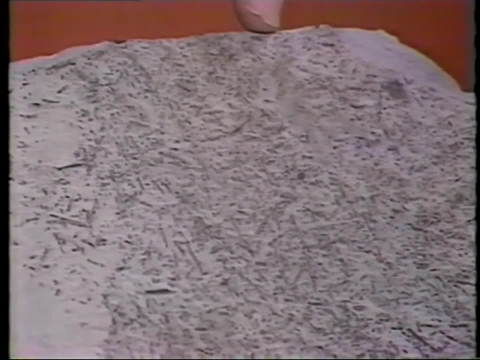 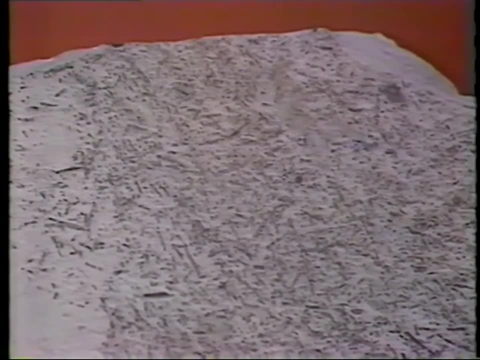 we had the burst of graptolites. Now you don't see them very well on this specimen because graptolites are very, very small fossils. They floated. They weren't deposit feeders, They floated high in the water. 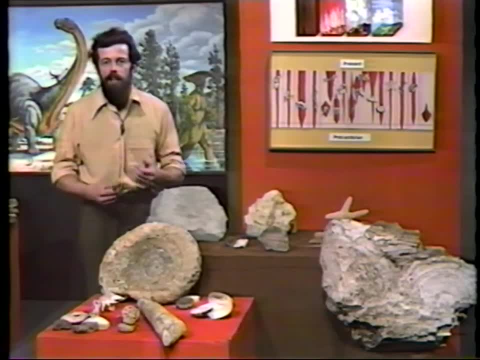 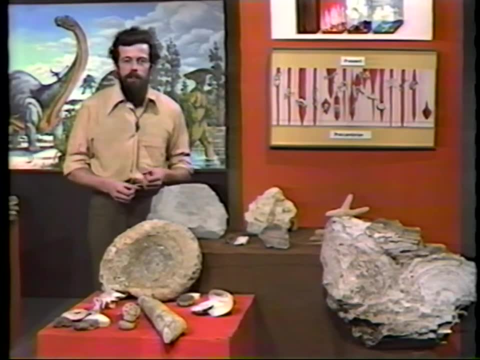 probably just beneath the surface, rather like floating seaweed, although they were animals. There are some very, very well-preserved graptolites which we can dissolve out of limestone, remembering that the silicification means of being fossilized. 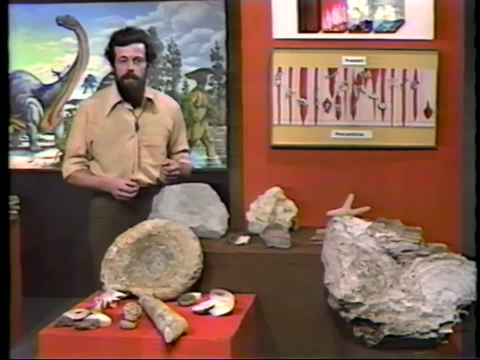 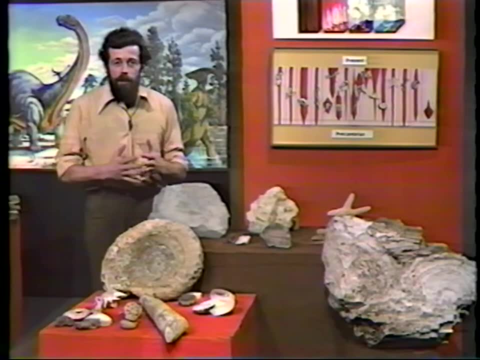 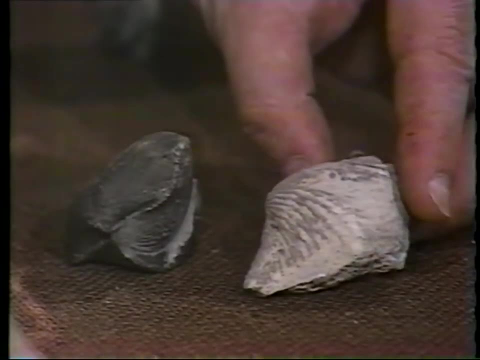 We can dissolve out some graptolites in the same kind of fashion as we can dissolve out silicified fossils, The graptolites, then floating organisms, Another fossil that we find dominant in the Ordovician system, Ordovician sea floor occupants. 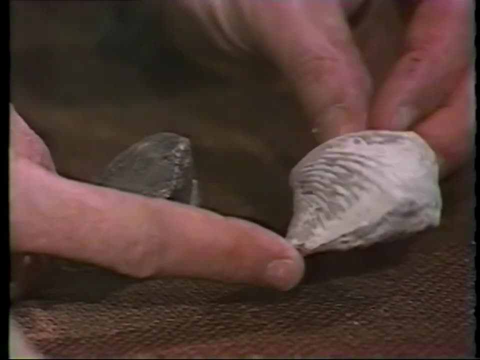 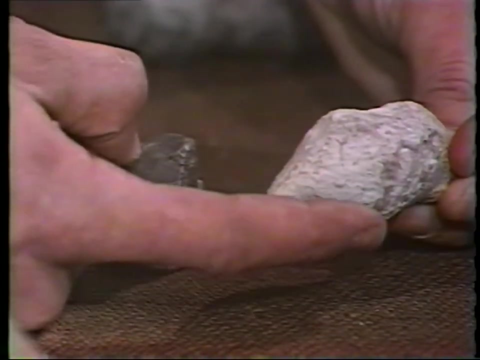 are the brachiopods. The brachiopods, like the clams, have two shells- Here is one and here on the other side is the other- and they were hinged together and the brachiopod lived like this on the sea floor. 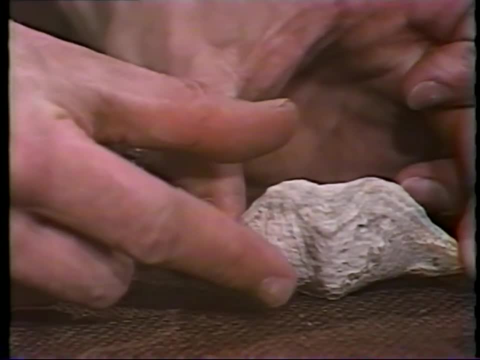 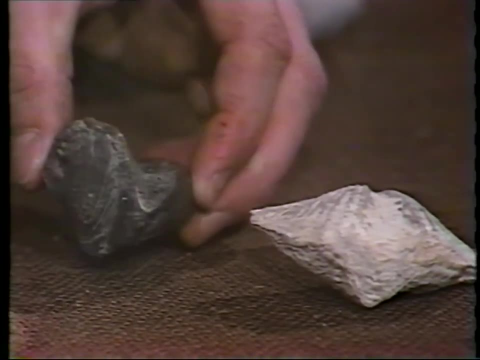 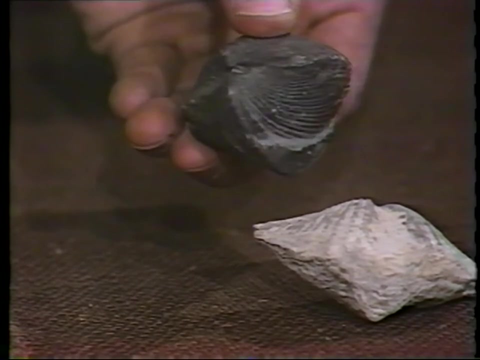 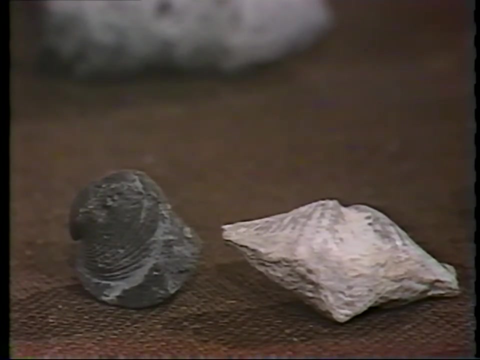 opening its valves or its shells, like so. And how did it live? It lived by filtering the seawater. Here is another brachiopod, Again two valves, and remember, brachiopods, filter feeders, filtering microorganisms out of the seawater. 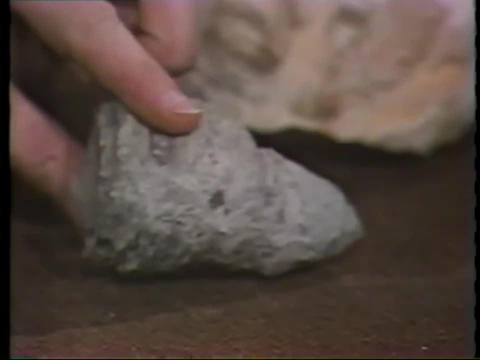 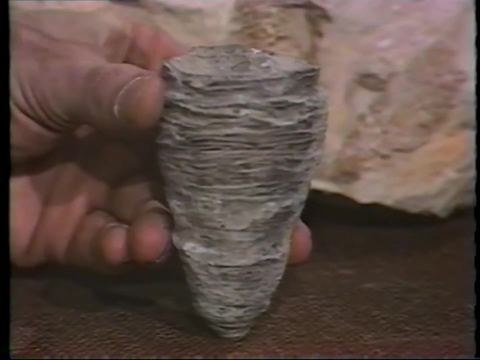 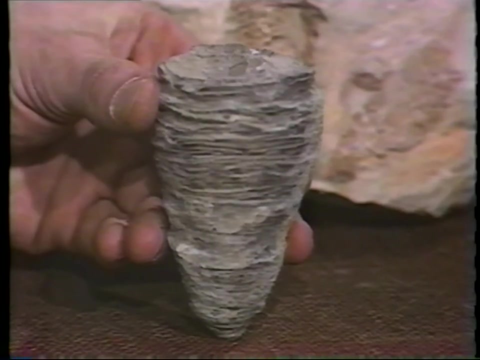 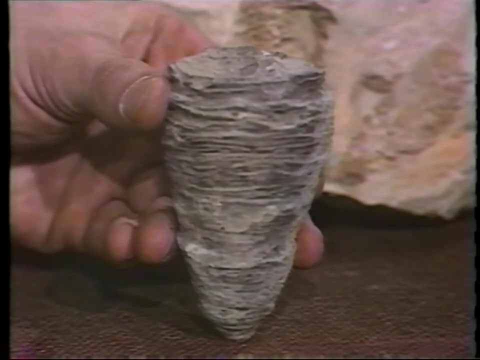 The same applies to the corals. This is a horn coral that lived like this on the sea floor, with filter arms, if you like, to filter the water that flowed over the top of it. It stood maybe six inches above the sea floor. 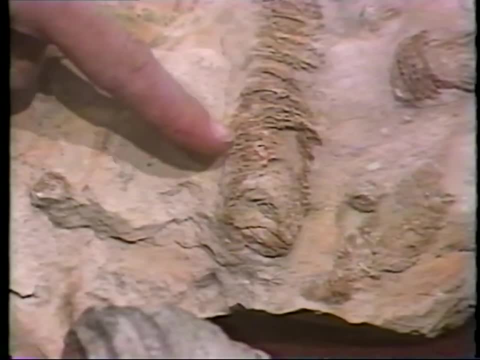 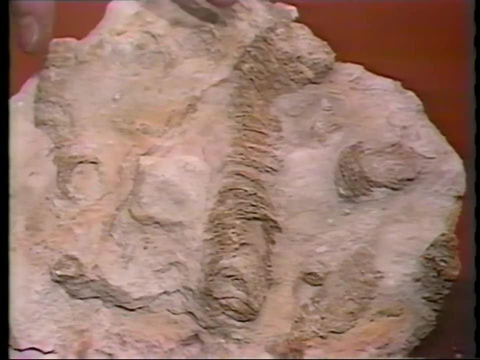 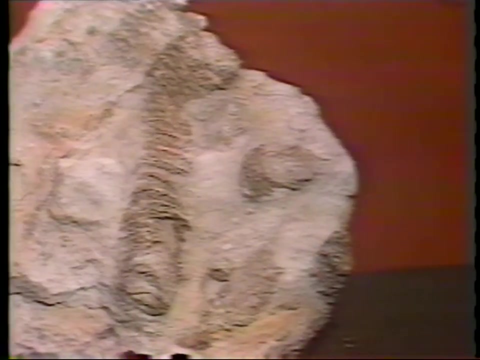 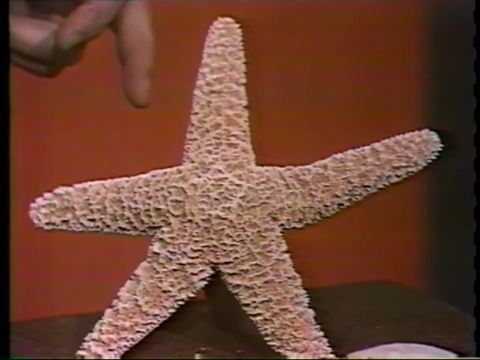 Here are other horn corals with a less distinctive, less distinctive shape, But remember filter feeders. And then, finally, we've got the echinoderms here. This is a recent sea star, one from the Pacific coast. You must have seen these. 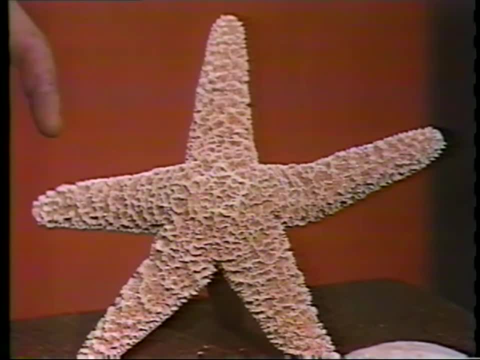 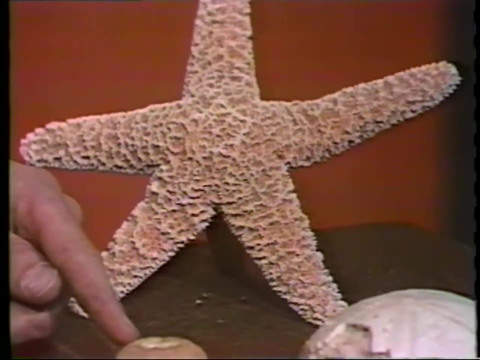 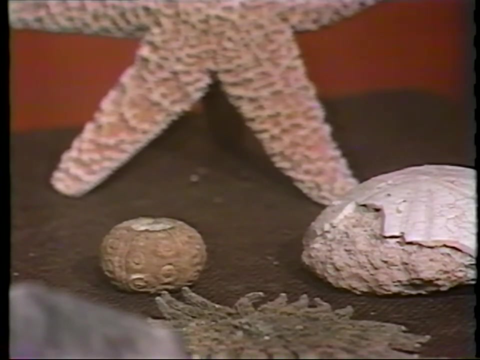 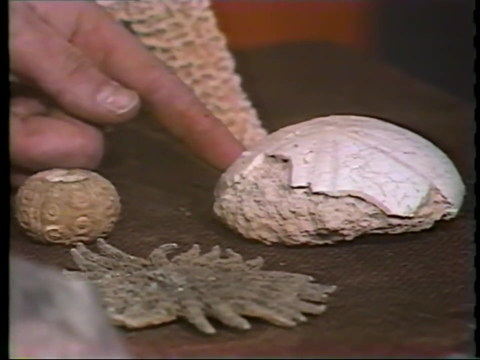 It's one of the echinoderms, the spiny-skinned organisms, A carnivore. And here is a related echinoderm, a sea urchin from the Jurassic, And here another, this from the Cretaceous. 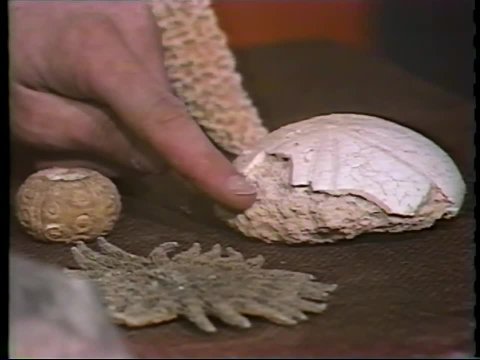 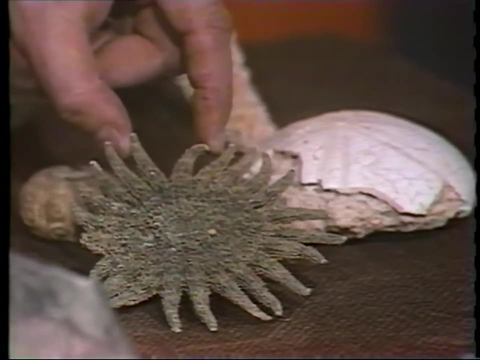 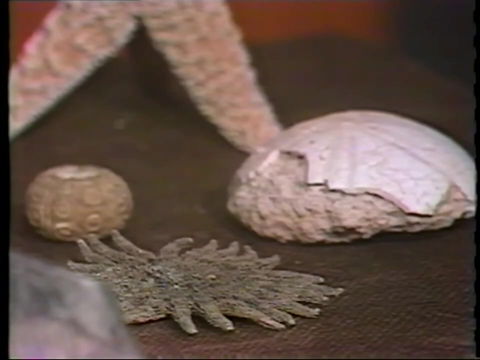 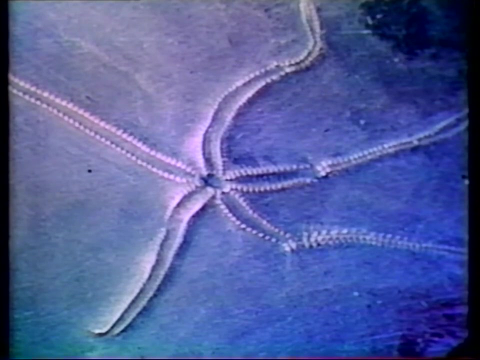 and showing the sediment inside the fossil. This is another recent sea star, this time with many, many arms, instead of just the five of most sea stars, Those sea urchins and sea stars are carnivores and filter feeders. So in the Ordovician, 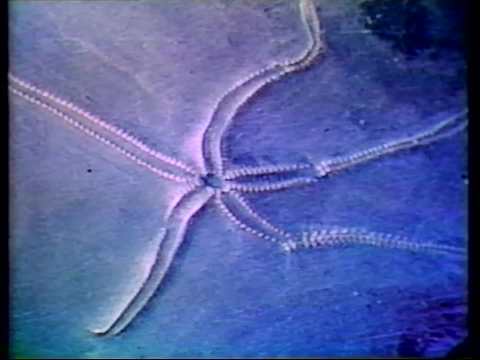 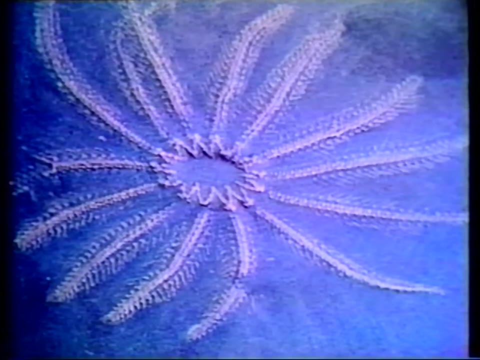 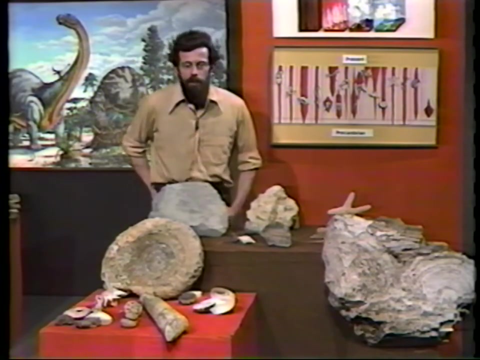 what we have are sea stars like this from the fossil record and like this one. The appearance in the Ordovician, to continue into the Silurian and the Devonian and the later Paleozoic systems. the appearance of many filter feeding organisms. 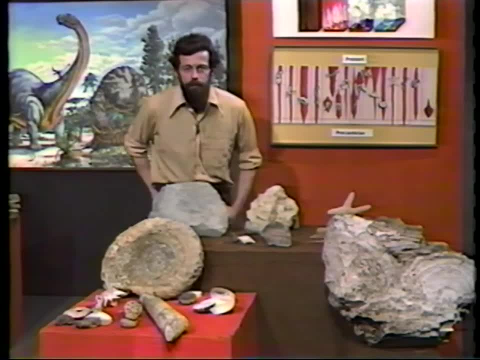 Quite a change from the Cambrian. Now then, why might that have come about? Why do we get deposit feeders in the Precambrian, deposit feeders in the Cambrian, and then this change in the Ordovician bringing in this multitude? 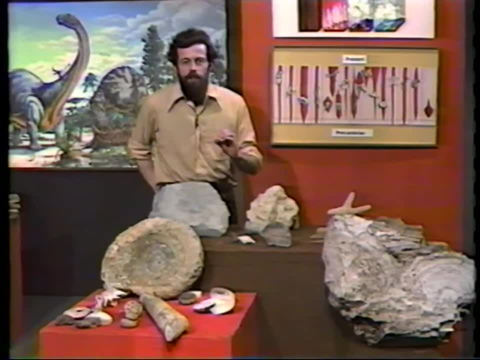 of different organisms, many of which are deposit feeders, some of them carnivores. Well, that's a question that's only just begun to be answered. In the last five years, it's been suggested that, in fact, continental drift provides us. 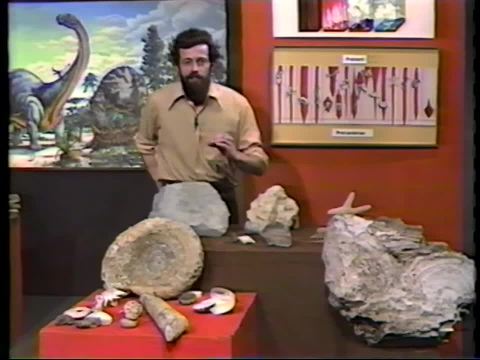 with the answer to this pattern of development of the animal life on the Paleozoic sea floor. Think of what the climate is like surrounding a large continent. Think of, for example, North America. Our own climate in Ontario is very extreme. 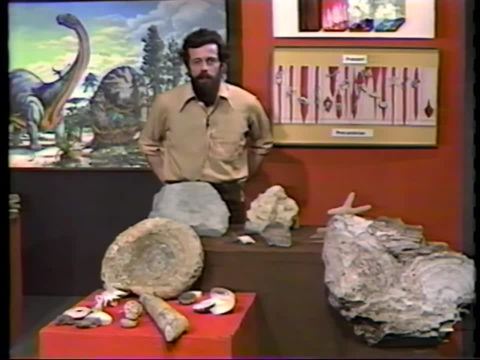 During the winter it's very cold, During the summer it's quite hot, And that continental climate on the land controls very much the kind of conditions that exist in the shallow seas off the coast of our continent. During the winter, cold winds tend to blow over those shallow seas. and during the summer the water can get much warmer because the cold winds have ceased. Now that's very much a generalization, but we can basically say that around large continents the seasonal fluctuations in the seawater are very much greater than around small continents. 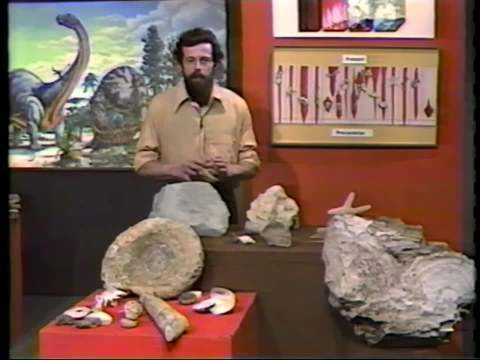 broken-up continents, because the influence of the land mass on the climate is very much less. Now then, in the Precambrian, it's thought that the continents were probably gathered together to create supercontinents, And this would mean that the climate 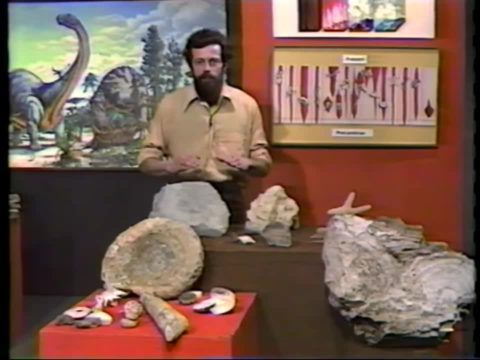 would be quite extreme, and the conditions in the shallow seas around the continent would fluctuate markedly, And that would mean that things like algae floating microorganisms would have a pretty tough time. They'd have a cold winter and a warm summer. 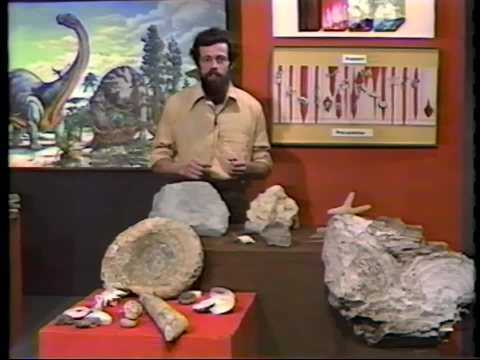 They'd have a tough time living, And that would mean that there was probably not the kind of food around that filter-feeding organisms needed in order to exist. The best place to live at that time was right on the sea floor, eating whatever settled to the bottom of the sea floor. 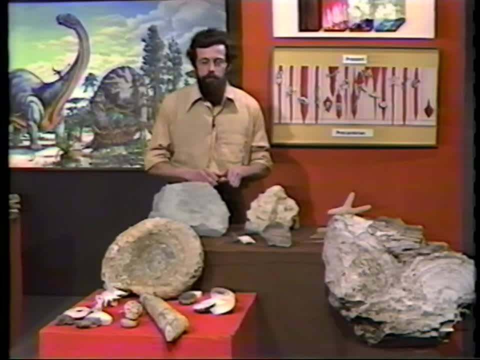 Now, then, in the Cambrian, the situation began to be slightly different. apparently, There are three major different kinds of Cambrian faunas- fossil communities, if you like- across the world, Whereas in the pre-Cambrian we can only identify the Ediacara kind. 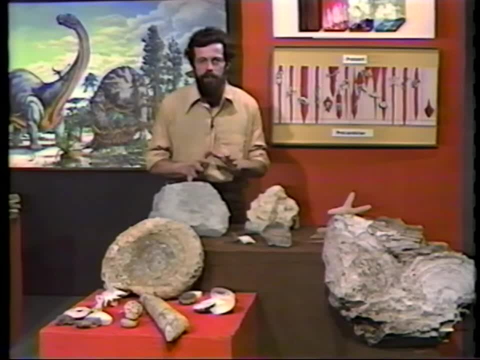 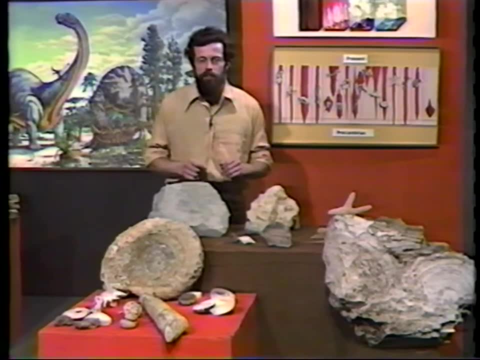 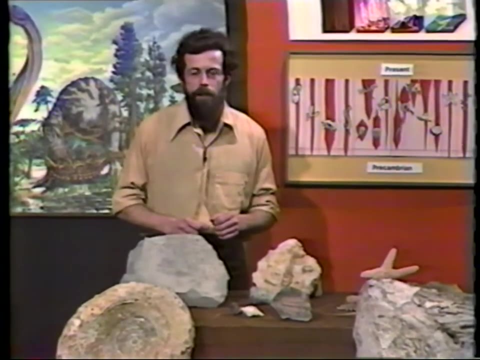 This seems to indicate that that massive pre-Cambrian continent was perhaps beginning to break up into pieces, And as it was breaking up into pieces, the conditions became somewhat less extreme in terms of climate around the coast of those pieces, And this gave an opportunity. 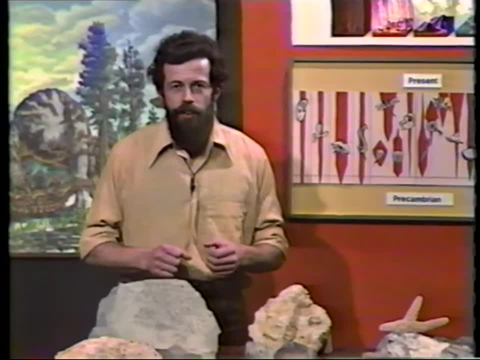 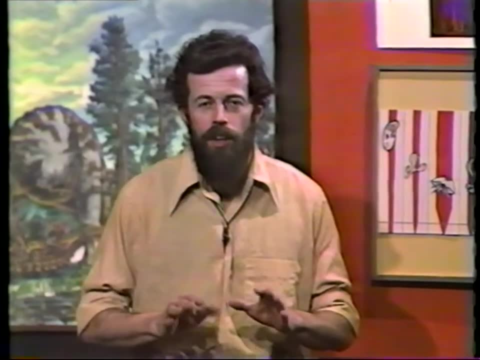 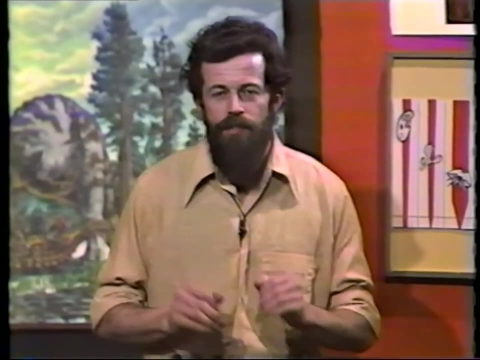 for organisms to begin to develop filter-feeding, because algae would be able to thrive in those more stable conditions around the smaller continents and they would be able to provide the food for early filter-feeding organisms. but still not very many filter-feeding organisms. And then in the Ordovician, the real fragmentation of that early pre-Cambrian continent was finalized. We had several continents in the Ordovician and around. those small pieces of continent is where the filter-feeders finally had their heyday, so to speak. 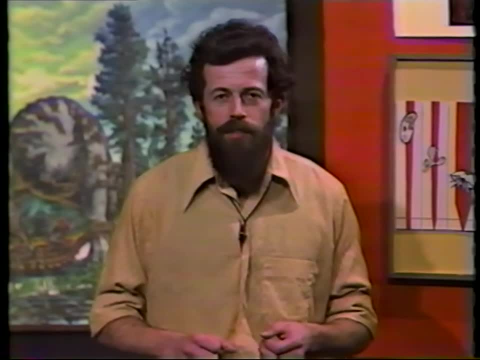 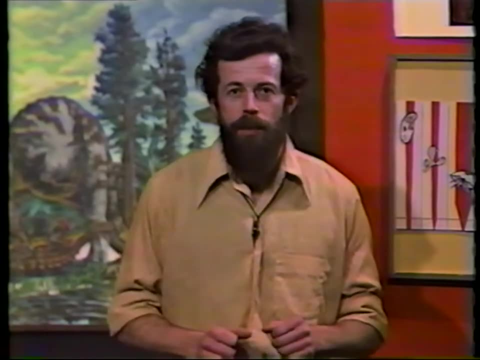 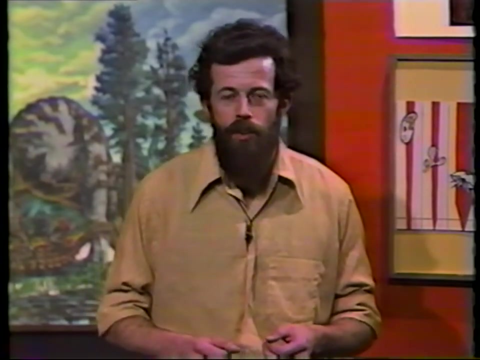 Algae were able to thrive in the water around those small pieces of continent. They provided the food for the filter-feeders and suddenly there was an opportunity for filter-feeders to thrive, And that's why we think the filter-feeders came into their own in the Ordovician. 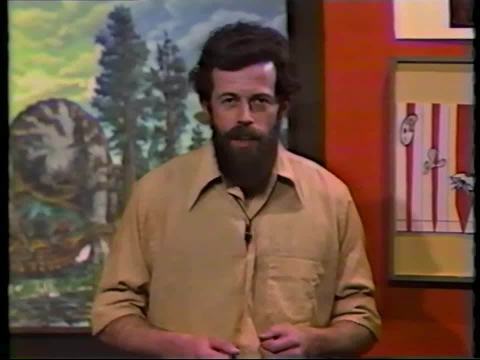 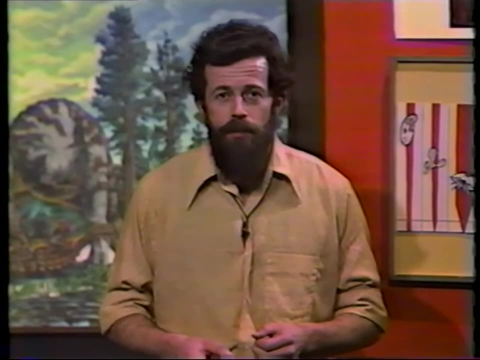 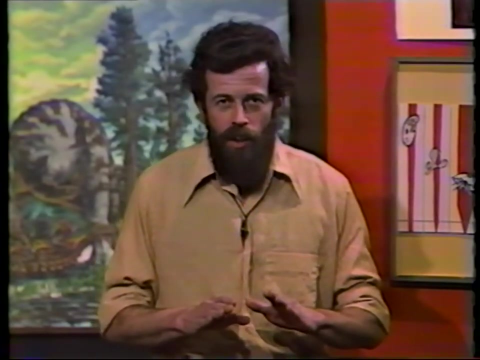 and to continue that way through the Paleozoic. Now, you'll remember, at the end of the Paleozoic is the time that Europe and North America collided to give the Appalachians And the creation of Pangaea, that supercontinent of the Permian. reversed the situation, And that's what we've just seen develop. The continents glued themselves together again, so to speak, became welded back together in one supercontinent. What happened? Well, at the end of Permian time, when the landmasses were all joined back together again. 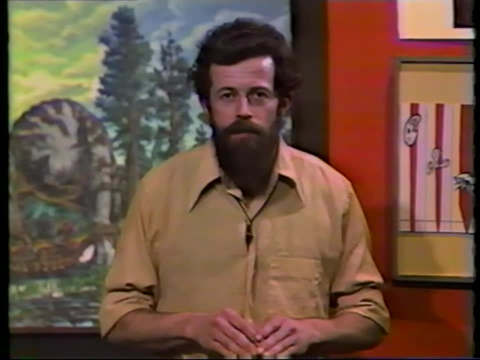 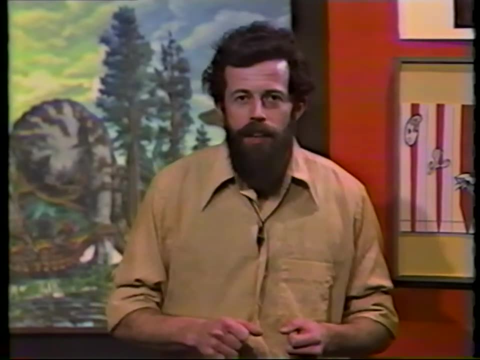 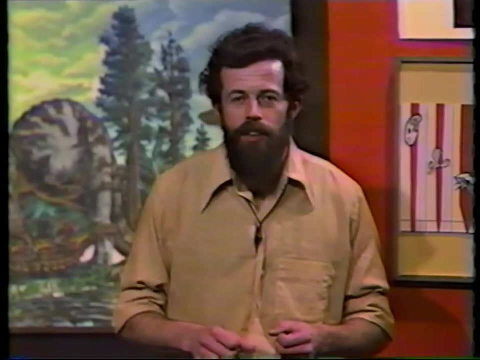 conditions became, we think, more extreme. the climatic conditions and the life for algae became more difficult. because it became more difficult, there were fewer algae in the water and the filter-feeders began to die out And in about 5 or 10 million years, 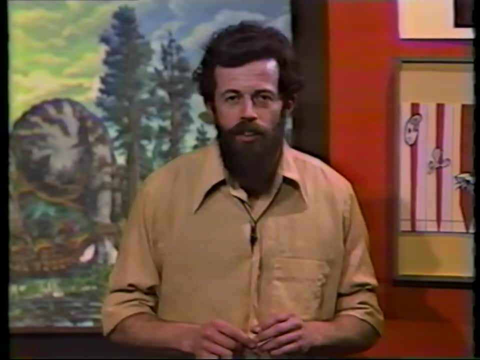 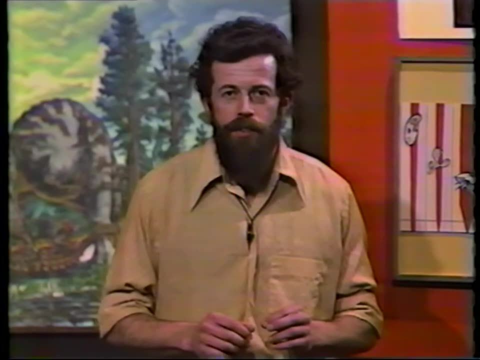 at the end of Permian time, we see a massive extinction of many, many different kinds of filter-feeders, The brachiopods, for example, which were filter-feeders of the late Paleozoic par excellence. very many brachiopods. had a really hard time at the end of the Permian, And the same goes for some of the carnivores. There was not so much in the way of life in the seas for the carnivores to eat, So they had a hard time too. 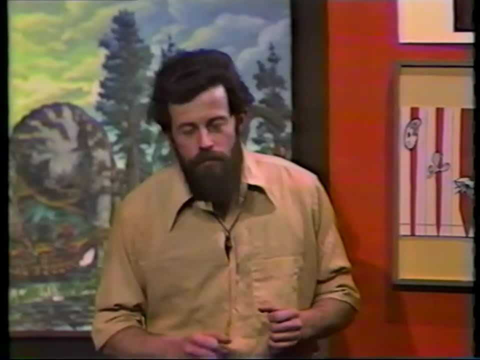 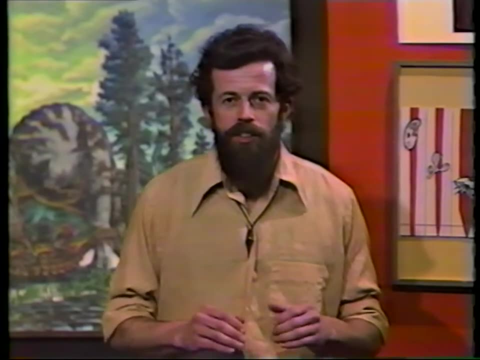 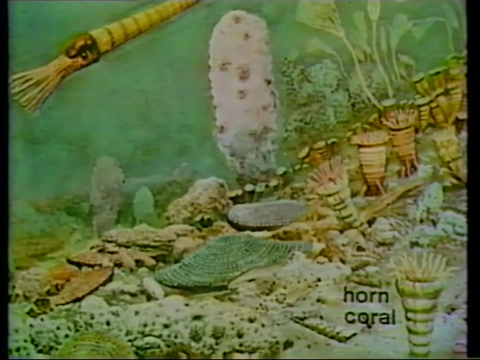 So what we're seeing is that the movement of the continents and the kinds of conditions that maintained that existed in those shallow seas around the continents was largely responsible for the conditions under which organisms had to live, And because they were responsible for those conditions, 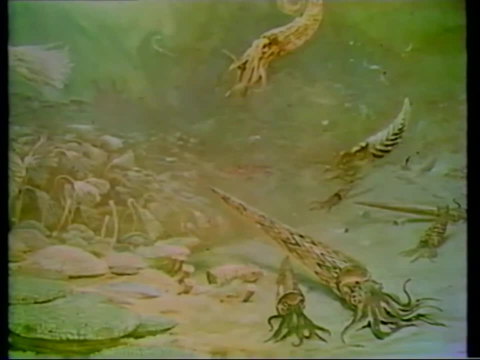 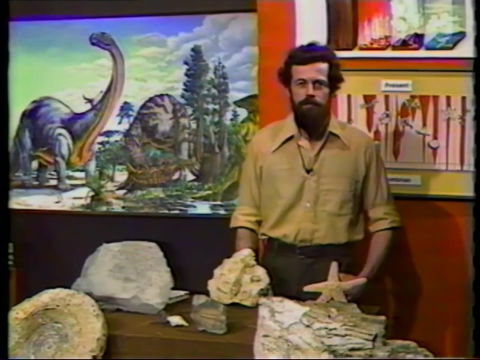 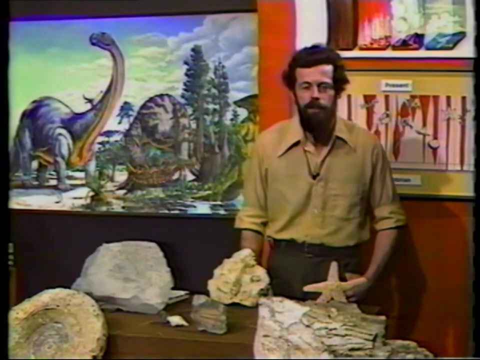 under which the organisms had to live. then they governed the kinds of organisms which were able to survive and adapt to the environment. The supercontinent of Pangaea broke up in the middle of the Cretaceous to give us the numerous small continents that we have now. 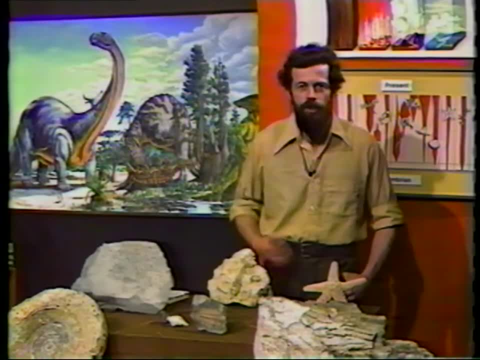 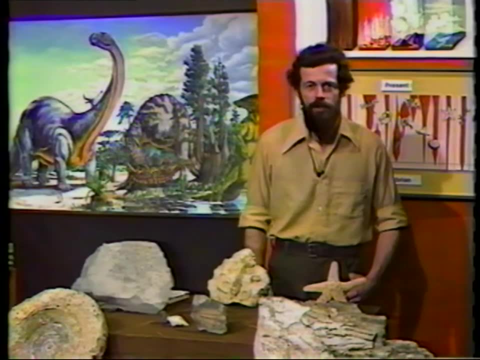 And as conditions became more stable, more oceanic, if you like, once again, the filter-feeders had their heyday. The main filter-feeders at the present time are the bivalve mollusks, the clams that we find in profusion on our seashores. 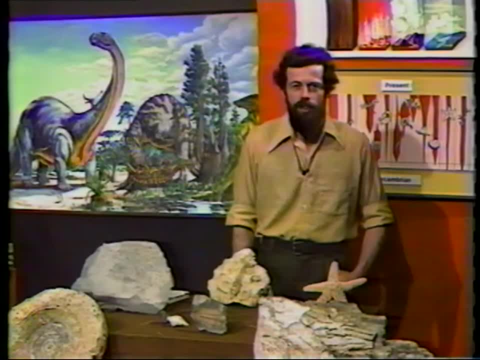 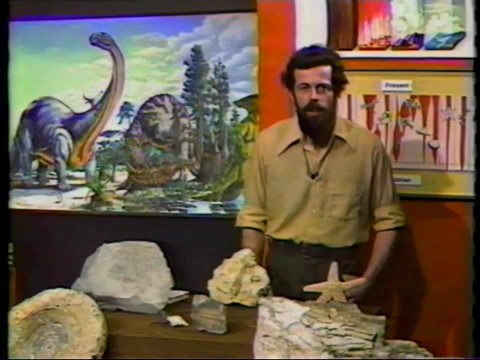 One very important group that's present throughout the fossil record, from probably the Precambrian, with soft-bodied relatives right up to the present day, are the echinoderms. It's a very important group and we ought not to leave our discussion. 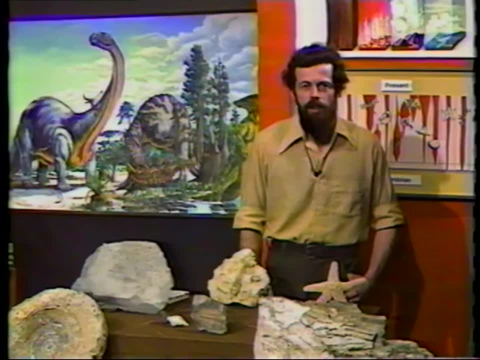 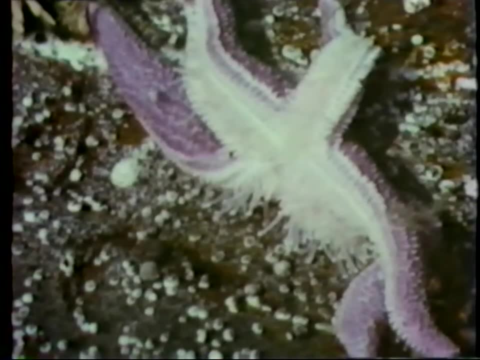 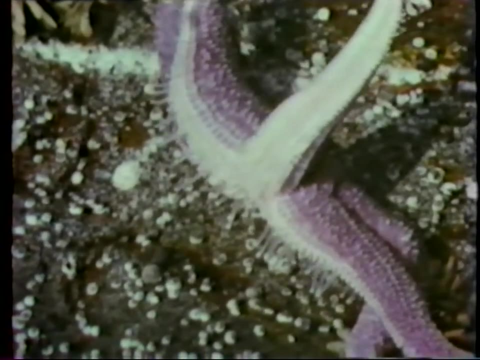 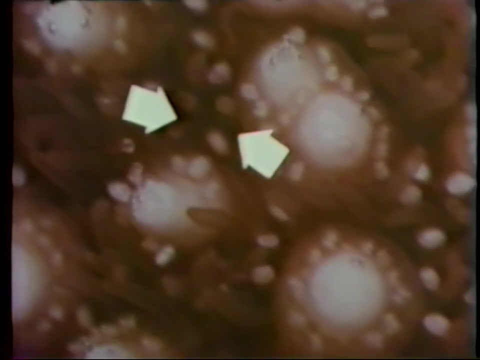 of fossils and their relatives without having a look at the mode of life and the variety of the echinoderms. The skeleton of the sea star when it's alive is quite flexible. Respiration is carried on through many skin gills distributed amongst the spiny knobs. 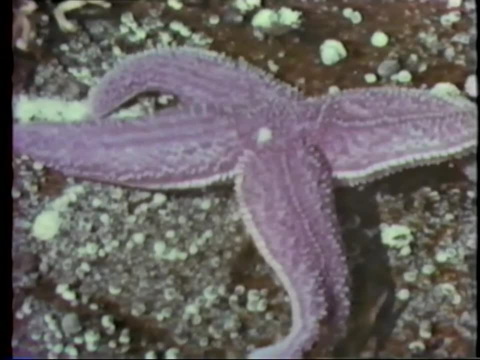 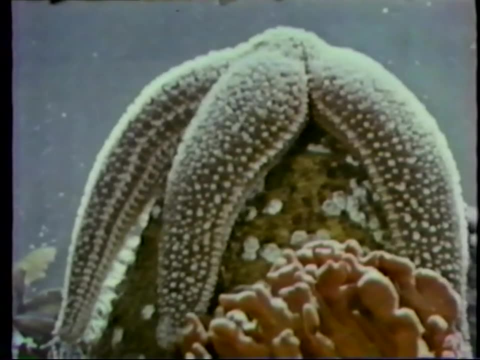 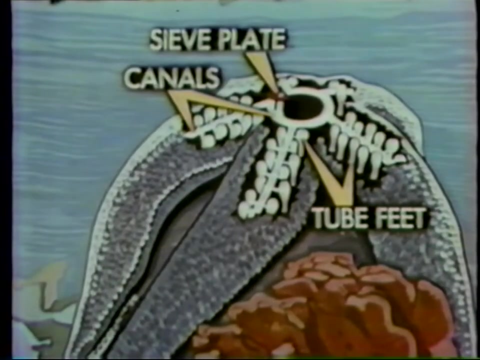 on the outside of the sea star. Oxygen diffuses through them directly into the body of the animal. Movement depends upon a kind of hydraulic system. Water enters through the so-called sieve plate at the top of the animal and flows into the ring canals. 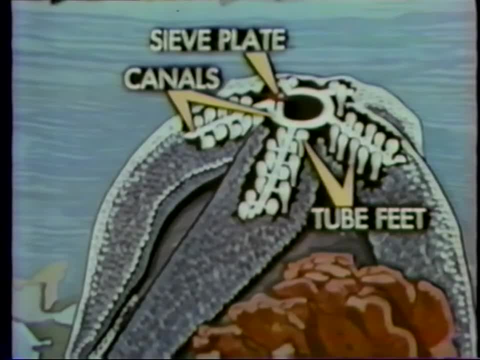 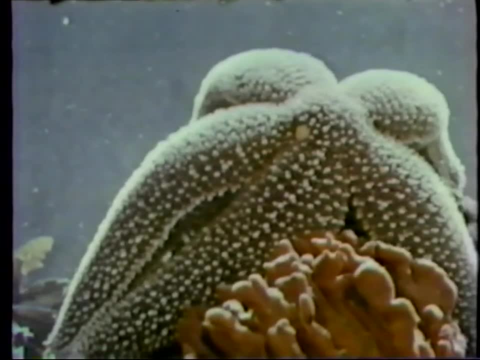 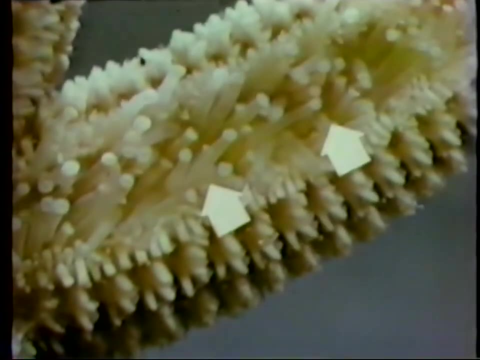 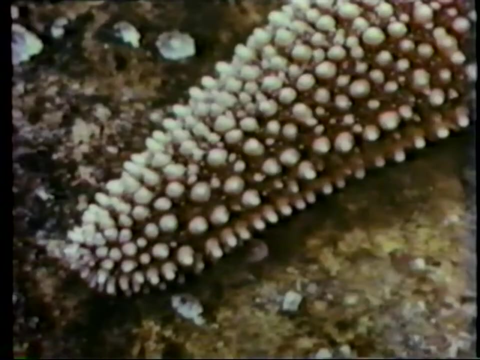 and then into the radial canals in each arm. It finally reaches the many tube feet. through the pressure It causes the tube feet to extend and the little suckers at the end of the tube feet hold onto the substratum and the combined action of the many tube feet. 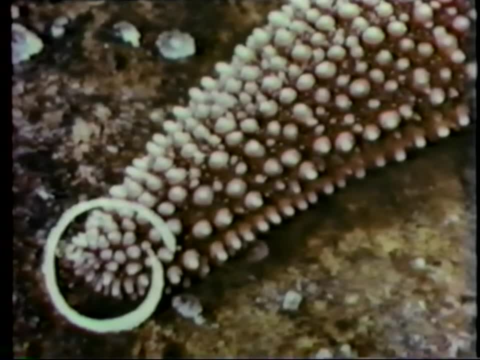 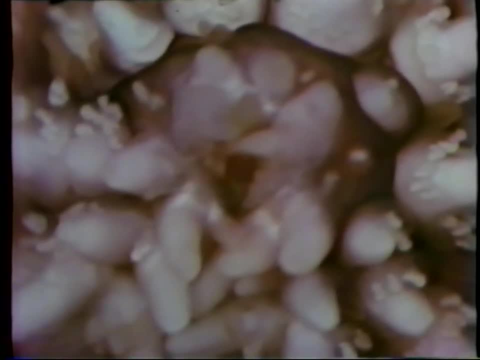 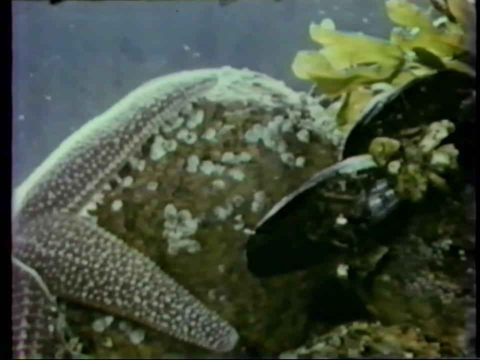 then propels the sea star along. At the tip of each arm is a tiny tentacle especially sensitive to touch and there's also a patch of light-sensitive cells, the eye spot. The starfish is a carnivore. It eats flesh. 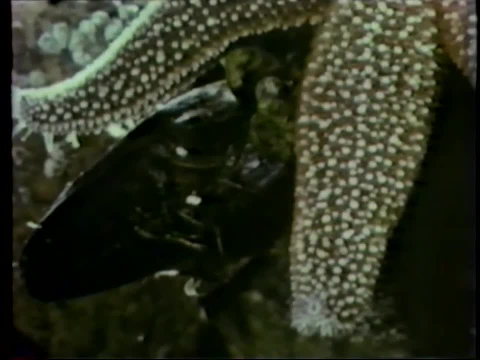 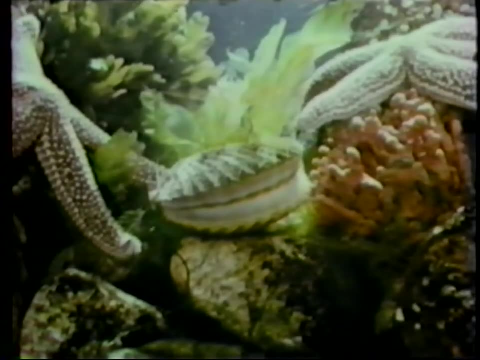 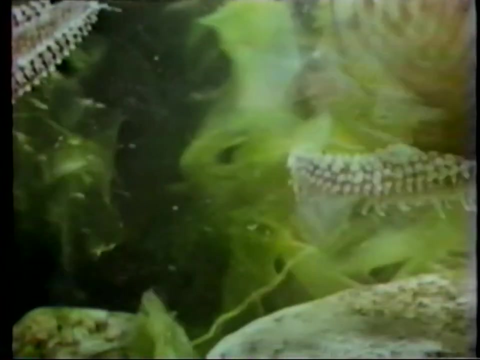 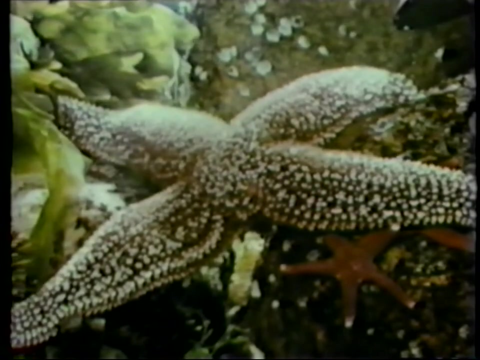 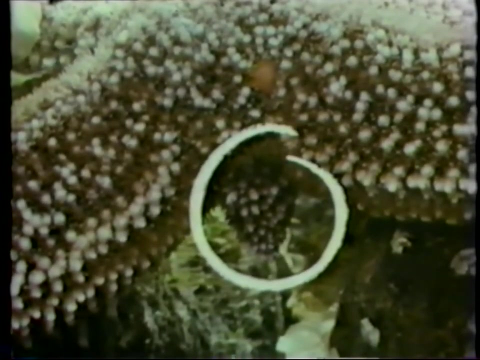 and it seldom has much trouble in catching its prey, the almost immobile clams, But sometimes it has more trouble. This scallop is not an easy meal. Sea stars sometimes lose an arm, in which case they're able to very quickly regenerate another one. 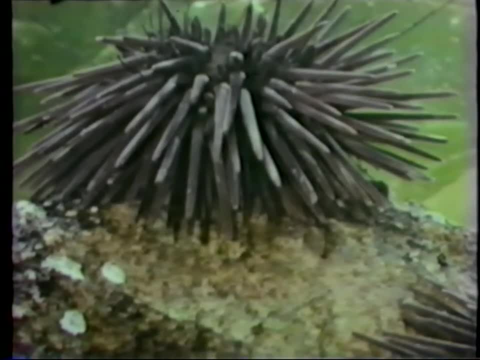 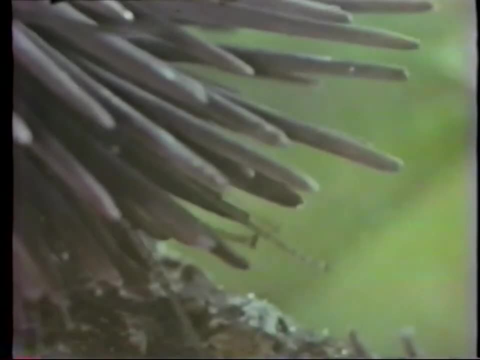 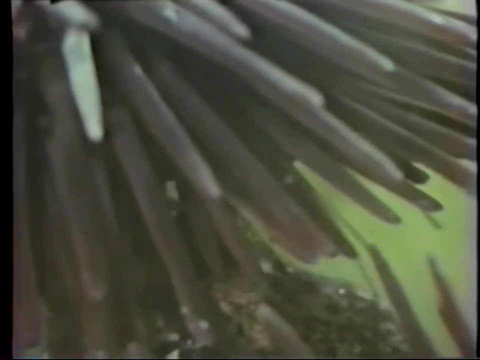 Sea urchins are rather like walking pincushions. Their rather globular body is covered by spines and between the spines are tube feet which enable the sea urchin to move. The sea urchins are scavengers. 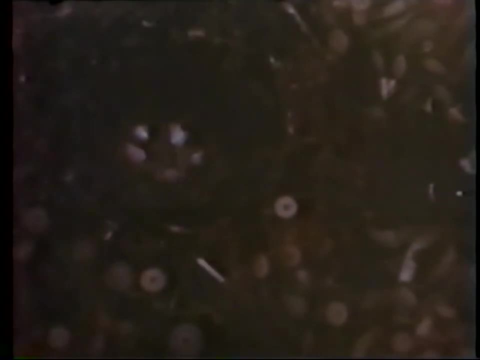 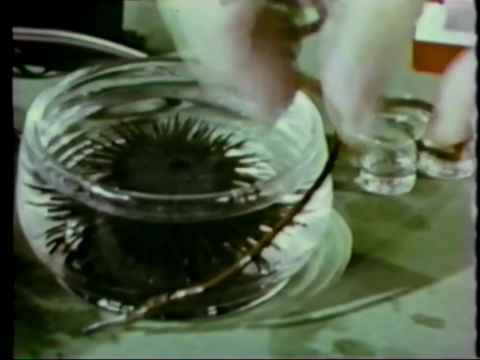 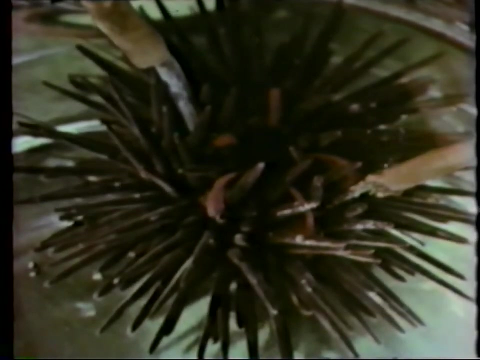 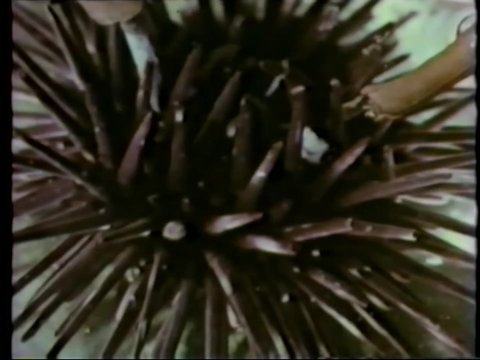 and the mouth is a rather vicious-looking instrument composed of five claw-like organs. The sea urchin is bisexual, and the male and the female can be readily induced to release the eggs and the sperm with the application of an electric device. The sea urchins are very sensitive to current. 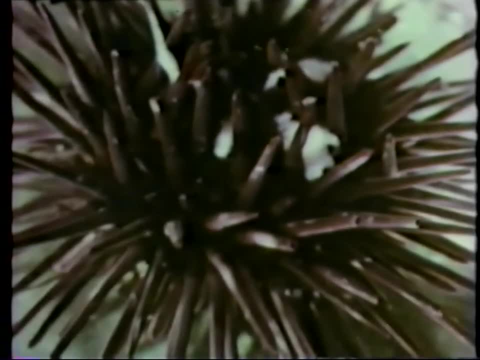 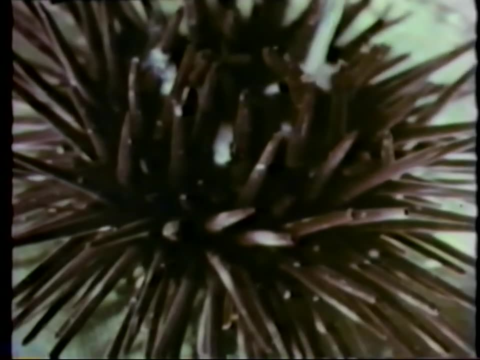 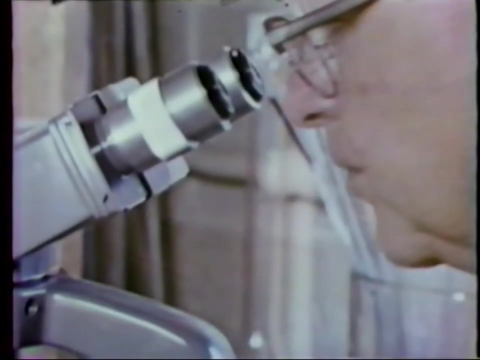 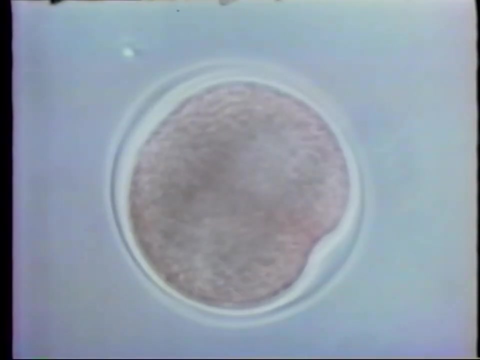 This makes them very useful in studying the mechanism of fertilization and embryonic development. The stream of sperm is gathered up here in a pipette and added to egg cells and examined under the microscope. The sperms are here fertilizing the egg, which quite rapidly divides into two. 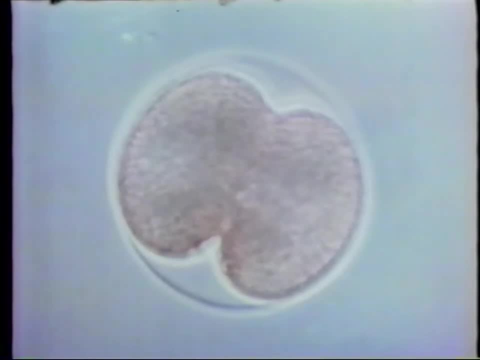 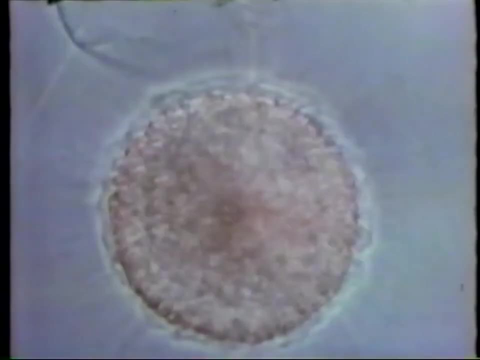 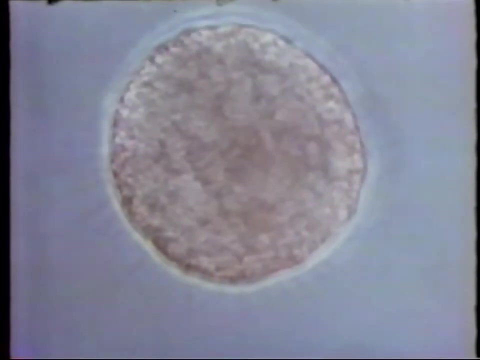 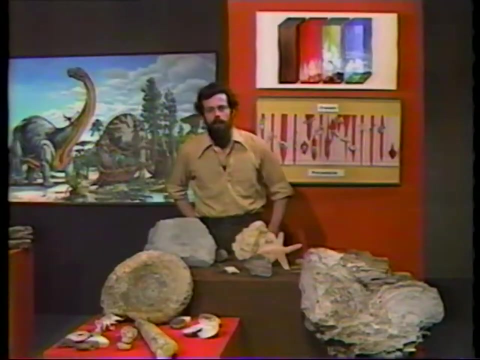 within, in fact about 24 hours, The developing embryo becomes free of the membrane of the egg and moves around by means of little cilia, little whip-like organs, and eventually becomes a free-moving blastula. The larval development that the present-day echinoderms show. 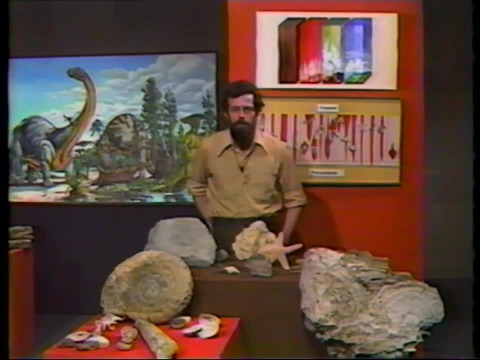 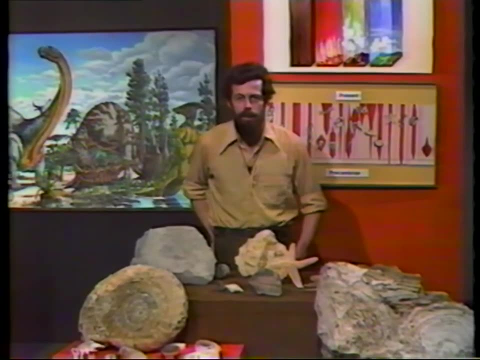 is different from that of other invertebrates, and that's probably one of the most interesting things about the group. It suggests that perhaps the echinoderms are somehow special, and it's even been suggested that they have something to do with the origin of the vertebrates. 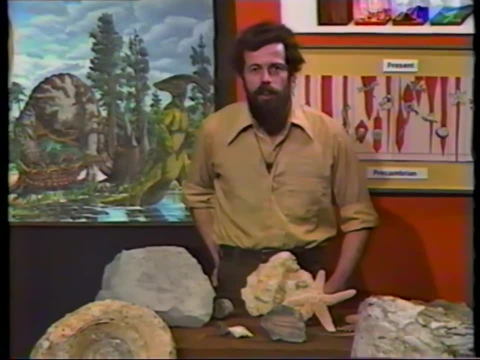 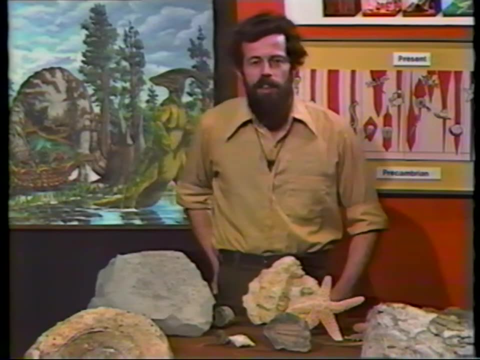 Now our understanding of fossils at the present day is, as you, I hope you've seen, quite sophisticated. We can do important things with fossils, But in the past the understanding of fossils was much less exact In the early part of the 18th century. 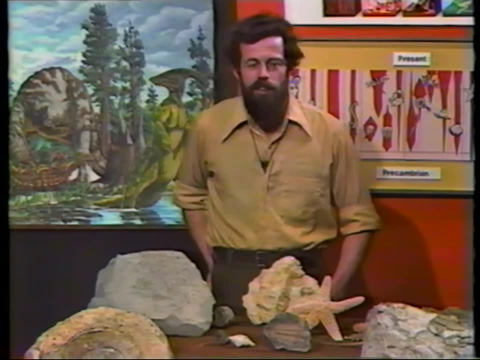 Johannes Behringer was the Dean of Medicine at the German University of Würzburg, very interested in fossils, and he had three boys collect fossils for him And eventually he published a monograph, But unbeknown to him, the fossils that the boys were collecting. 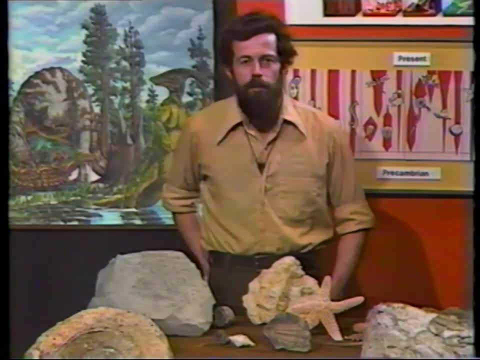 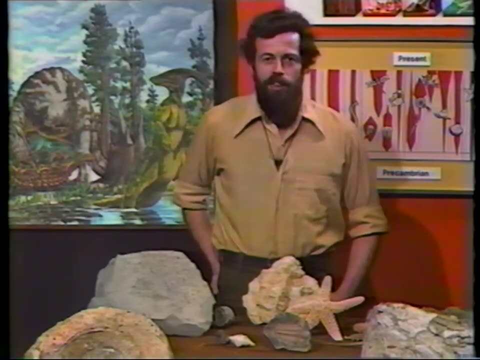 were fossils that had been carved by some of his colleagues, by the professor of geography and mathematics, aided by the university librarian and one of the local barons. Apparently, they wanted to demonstrate Behringer's gullibility and they decided that they would hoax him. 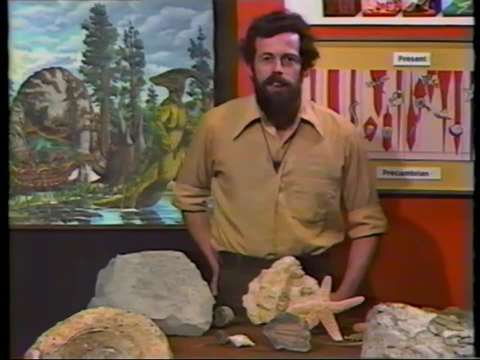 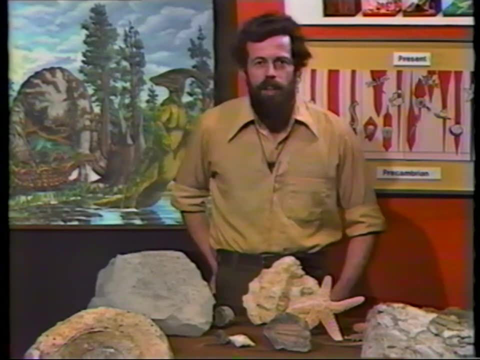 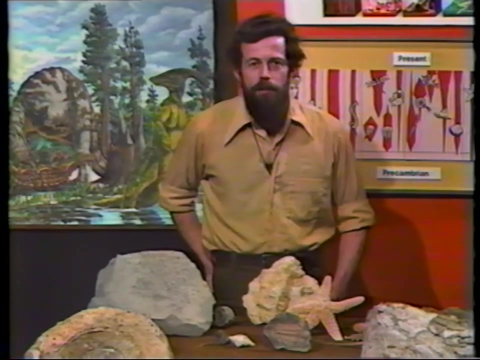 Even after they admitted the hoax, Behringer refused to believe that he had in fact been fooled and he went ahead with his monograph anyway. Eventually, he was convinced when one of the fossils that was brought to him had his own name in Hebrew on it. 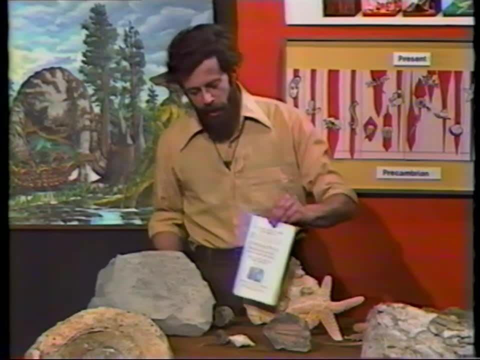 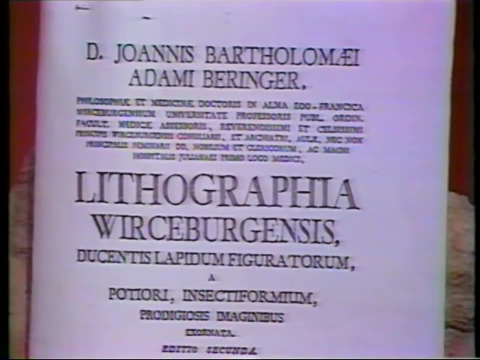 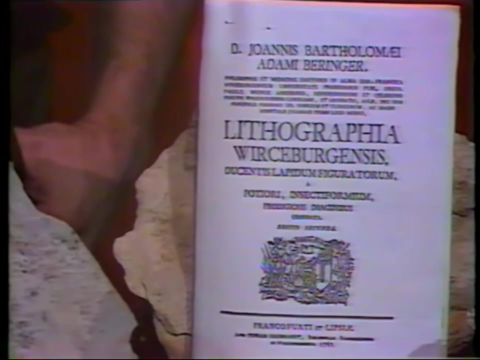 The fossils that Behringer illustrated in his monograph are indeed an exotic collection. Eventually, when Behringer realized that he'd been hoaxed and his monograph had already been published, he tried to buy back the original copies and burn them, But he didn't succeed and some survived. 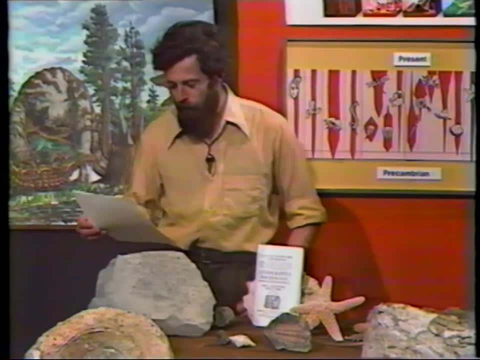 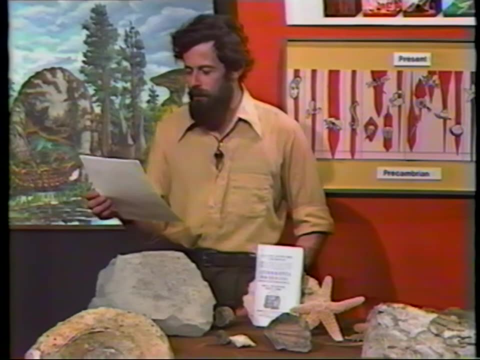 and I can quote to you what Behringer wrote. I doubt that any more heartwarming spectacle can come to the eye of a scholar of natural science, for all these figures are not merely outlined or sketched, but stand out so boldly. after the manner. 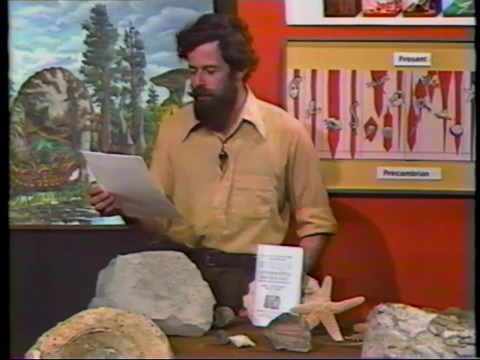 of sculptured relief that many erudite scholars and illustrious men of letters could not refrain from suspecting that some imposture lay hidden beneath these extraordinary mysteries, that the stones were fictitious and were fabricated in secret for the purposes of fraudulent avarice. 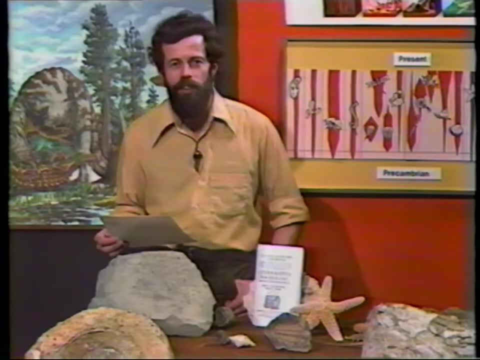 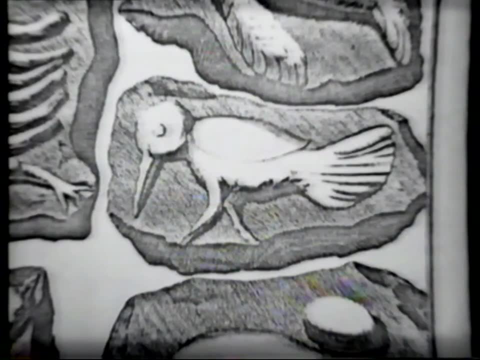 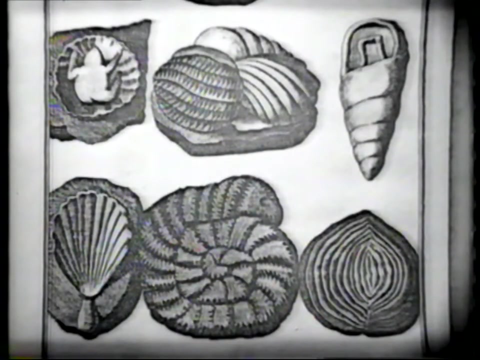 Let's look at some of those fossils that Behringer realized too late were frauds. Some of them, such as these shells, do bear some kind of resemblance to what might be expected of fossils, although the baby in the top left is rather odd. 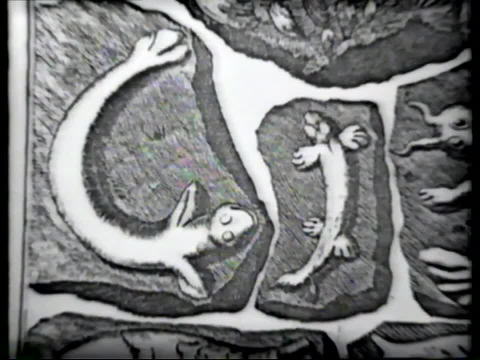 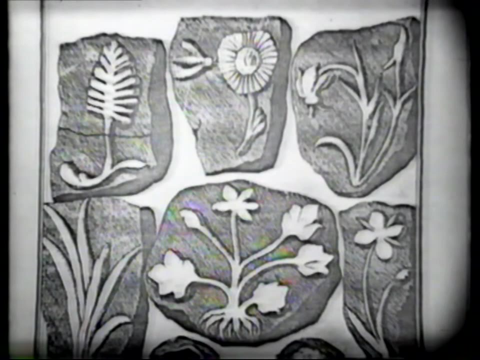 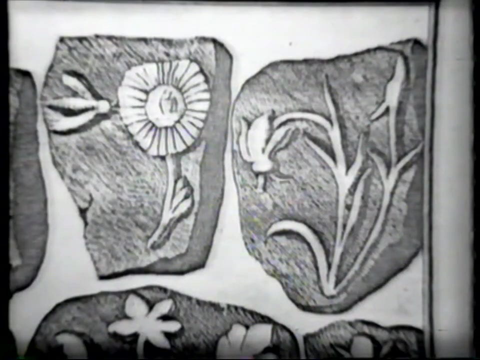 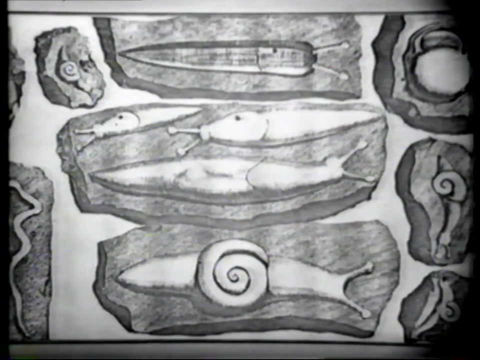 On the other hand, some of the others, such as these lizards, begin to look a little inventive. This lobster is quite formidable and the bee about to alight on the flower in the top of the screen is very imaginative: The soft parts of snails and spiders' webs. 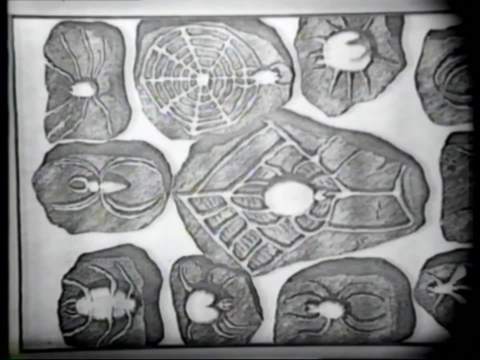 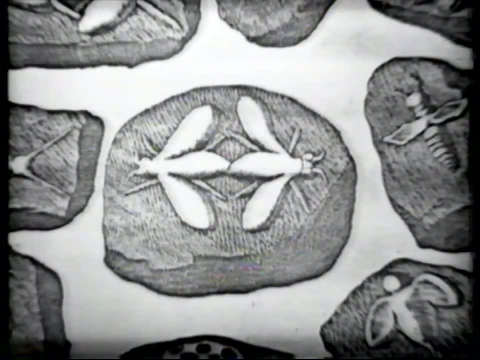 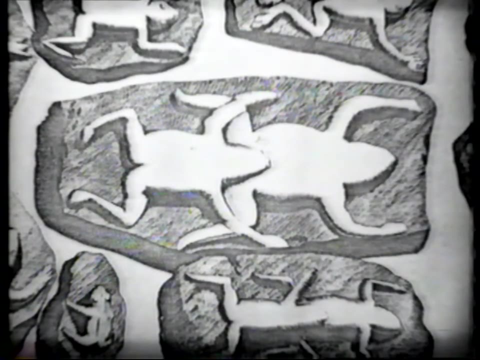 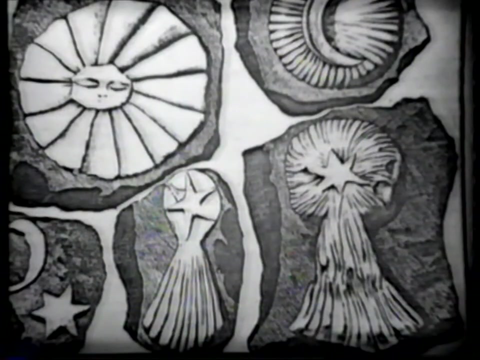 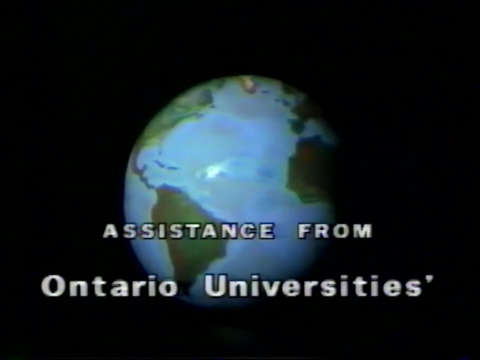 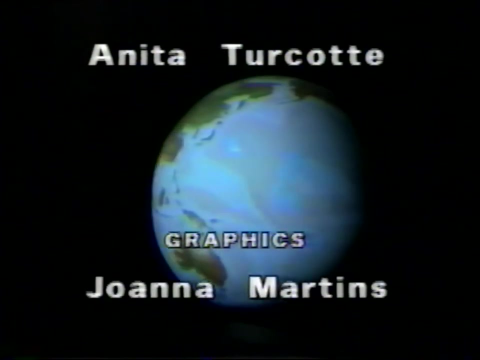 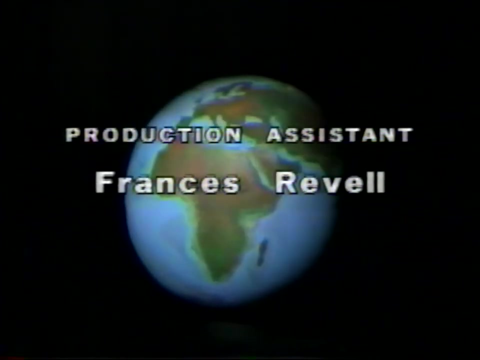 begin to look just too good to be true. Two insects getting together and two frogs And quite a party of reptiles and lobsters, and the sun and the moon and comets, And quite much to the rogue of the reptiles. 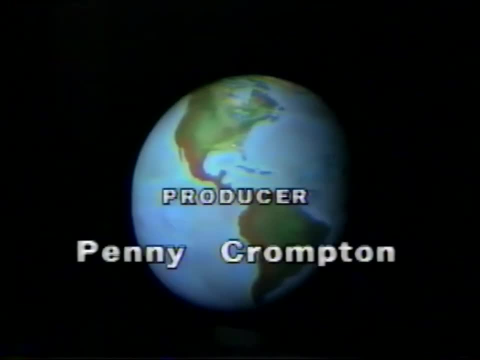 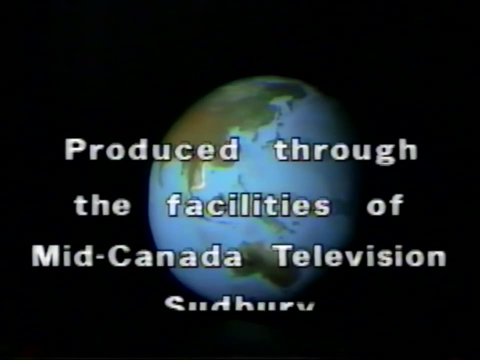 And quite a tiny little bug-legged bug about to form on a single flower. In fact, there are many reptiles in this very region, as well as on the other side of the ocean, and on the other side of the ocean, and on the other side of the ocean.